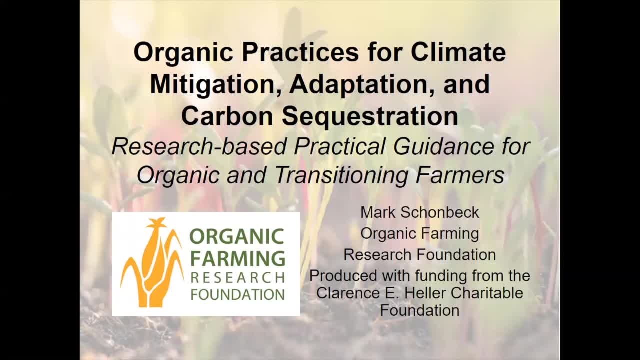 with funding from the Clarence Heller Foundation. I'm your host, Alice Formiga of eOrganic. eOrganic has many articles, videos and webinars about organic farming and research, and you can find all of them by typing webinars by eOrganic into a search engine, and you can also find the 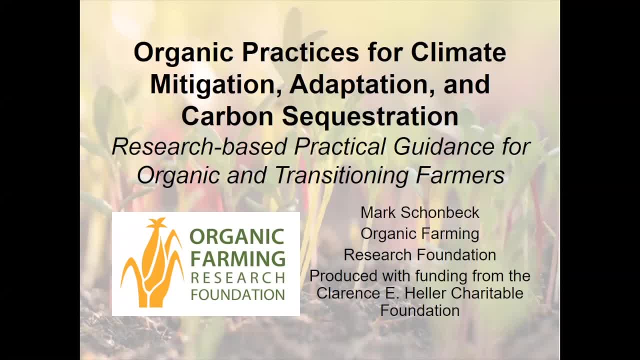 recordings on the eOrganic YouTube channel. We are recording this webinar and we'll have the recording available on YouTube within one to two weeks. This webinar will last about an hour and when it's over we'll have 30 minutes for questions, If you have a question. 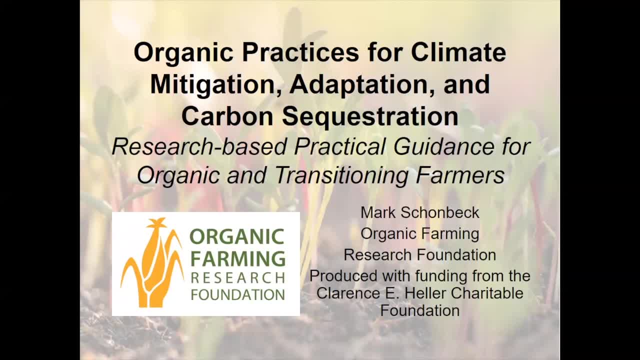 feel free to type it into the Q&A box on your webinar control panel. If you don't see the Q&A box, there should be a black bar with some controls at the bottom of your screen and if you hover over that, that should pull up the Q&A one. There's also a link to a PDF. 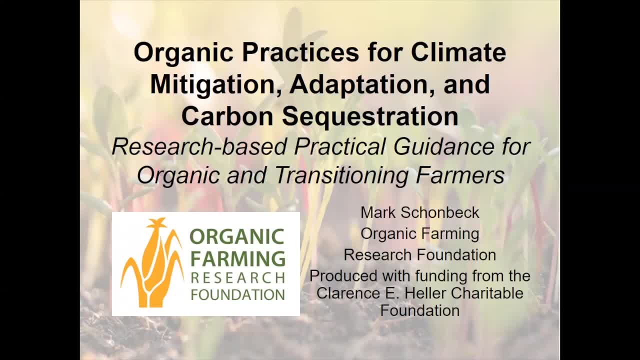 handout of the slides in your chat box and we'll be sending those and extra presentation notes that Mark prepared in a follow-up email that you'll be receiving with an invitation to fill out a survey. So I'd like to welcome back the presenter of this webinar series, Mark Schoenbeck. Mark is a research associate at the Organic 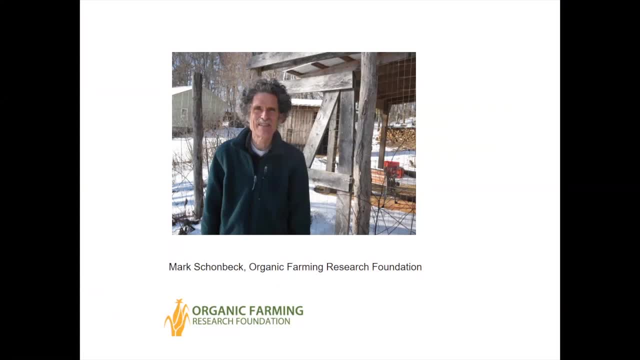 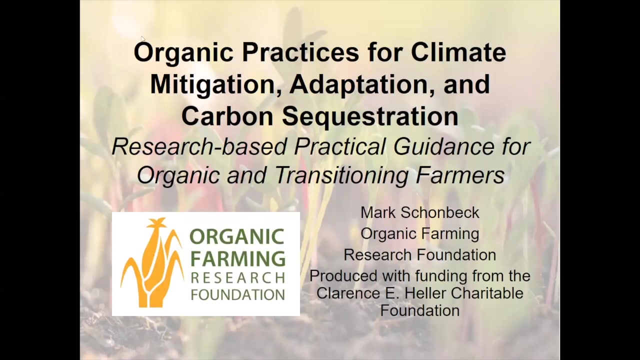 Farming Research Foundation and he's worked for 31 years as a researcher, consultant and educator in sustainable and organic agriculture. He's also been very active in the Virginia Association for Biological Farming. So welcome, Mark, and I'm going to hand over the. 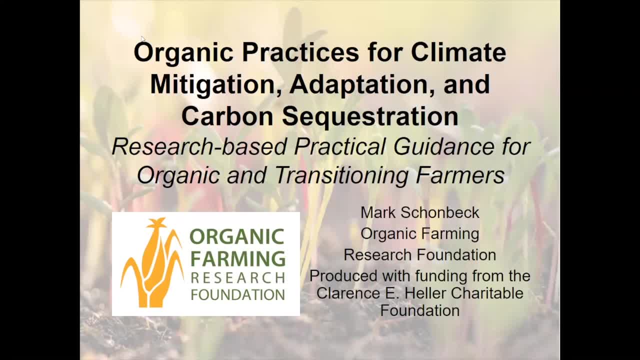 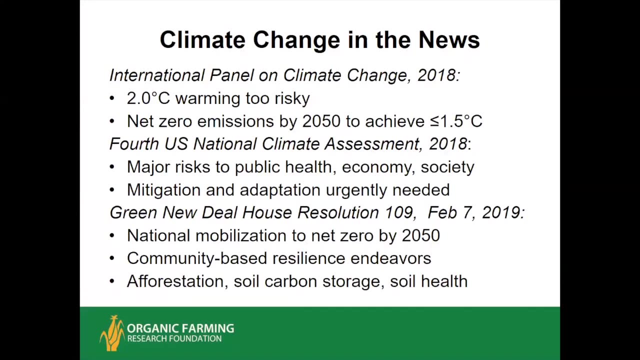 remote control of the slides to you and, just as a reminder, click on that screen to activate. Okay, thank you. Okay, welcome everyone, and today we'll be talking about the climate. It's been in the news lately, As summarized here on this slide in 2018, last fall, the International Panel on Climate Change. 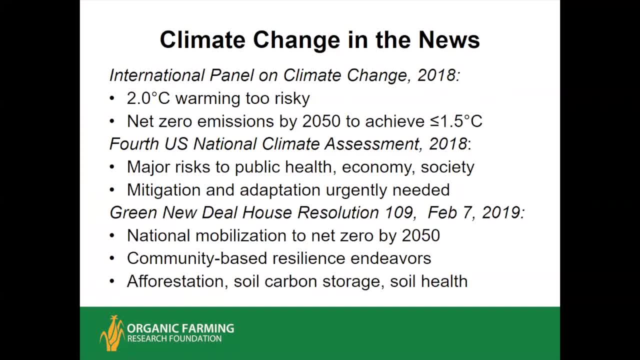 issued a report analyzing the impacts of a 1.5 degree Celsius increase in the average global temperature. we are now approximately at 1.0 degrees and already feeling significant effects, So there was widespread concern that allowing it to get as high as two degrees Celsius or 3.6. 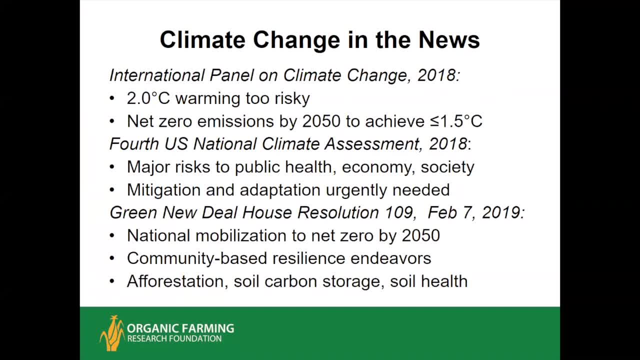 Fahrenheit was simply too risky. For example, it could cause a 99% loss of coral reefs from our oceans, And that could have some pretty serious and wide ranging impacts, and not just on tourism. So what the IPCC did is not only look at the impacts of 1.5 degrees, which themselves are 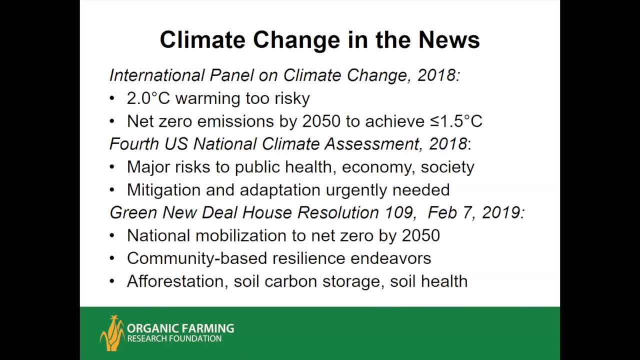 significant but also projected what it would take, that basically, we need to get the earth to net zero greenhouse gas emissions by the year 2050.. In other words, we need to be sequestering enough carbon through sustainable agriculture and other activities as we are emitting in. 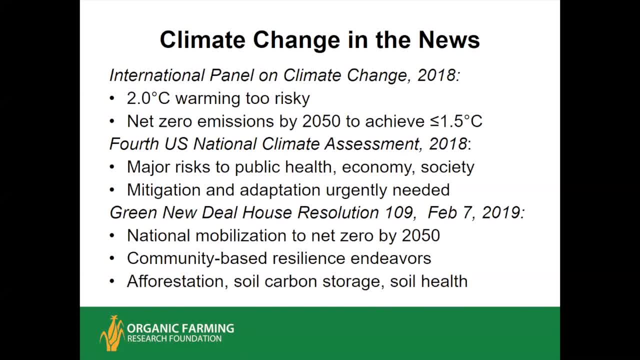 equivalence in terms of the greenhouse gas emissions. So that's what the IPCC did In terms of greenhouse gas global warming potential. Last fall, also, the United States fourth national climate assessment was issued. This is a joint publication by a number of agencies, including Environmental Protection Agency, Department of the Interior Department. 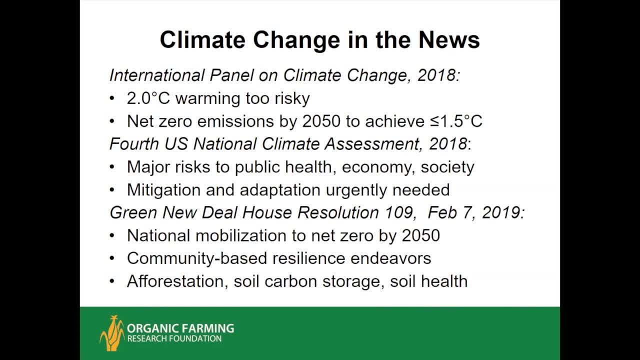 of Agriculture, et cetera, And basically, one of the findings was that, yes, we are, as a society, beginning to tackle this problem, with both climate change and environmental protection, And so we need to be looking at both: adaptation, preparing communities for the impacts of 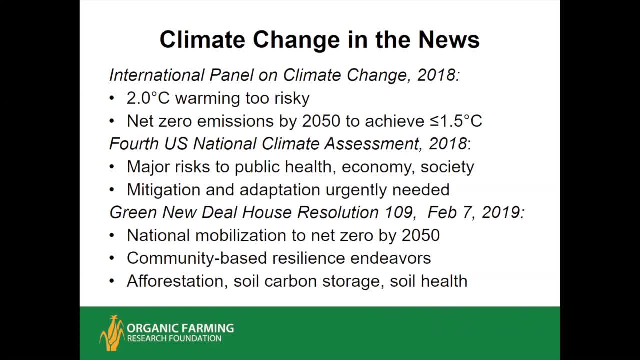 climate change and mitigation efforts to both reduce emissions and improve the return of carbon out of the atmosphere into biomass and soils. This fall actually this year in February. in the same week in the House of Representatives, a Green New Deal House resolution was introduced by Representative Ocasio-Cortez and Senator. 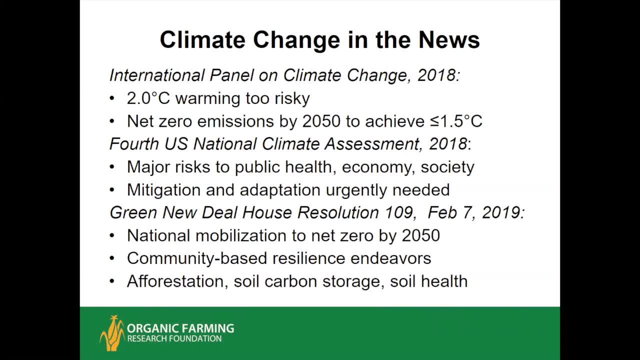 Markey, Okay, And this was the first time that the governor was meeting with the people around the country about the Environment Green Deal And it was quite a change actually in the history of the Green Deal And there was a lot of discussion around this. 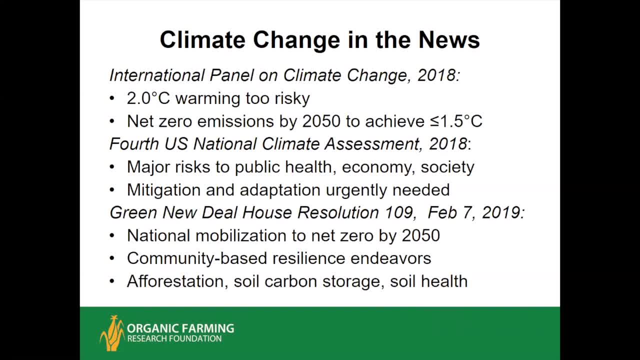 I think it was very much a conversation about how, how the might be you know how these changes should be implemented in our environment, how these changes should be used for ways to improve a healthy agriculture. Oh, I think we've lost a lot of places here. 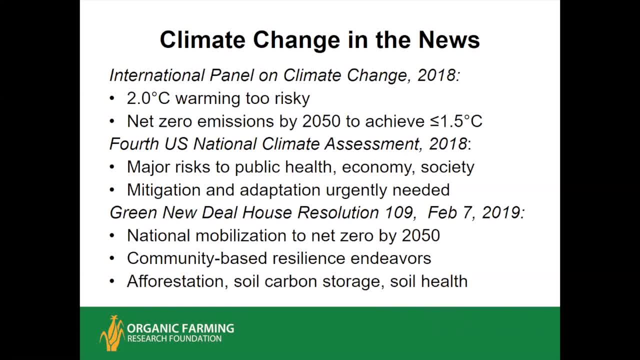 I'm sorry. Yes, Yeah, they're both great. Yeah, All right. Thanks, It was nice talking to you, Steve, And I think I'm going to pass it back to you, Whitley. Thanks, Steve, I'm sure you're going to have plenty of answers. 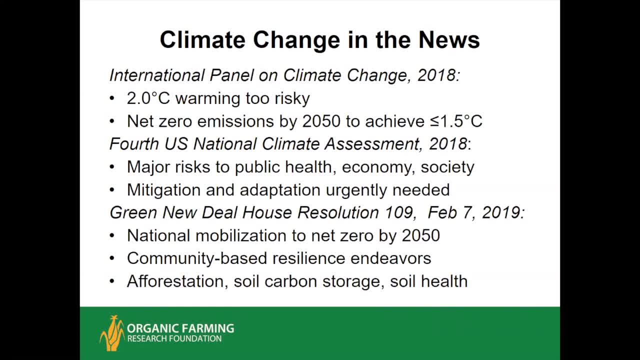 I'll keep you posted for any of these questions of the solution, but it did not really seem to fully depict the potential for sustainable agriculture to bring about real benefits in this area. That same week, the Speaker of the House also reconvened a select committee on the climate crisis and there were several hearings, So it's. 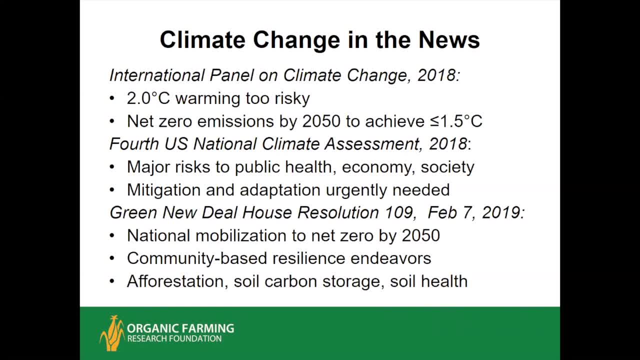 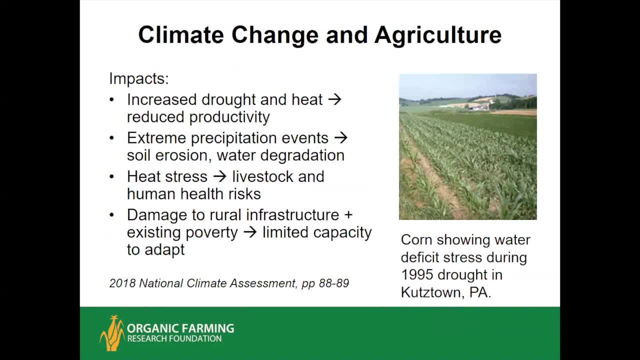 actually a very opportune time to engage the public and our leaders in the efforts that we will talk about here. Okay, so what is climate change? How does it impact agriculture? The most severe impacts seem to be currently around extremes of precipitation, prolonged severe drought. 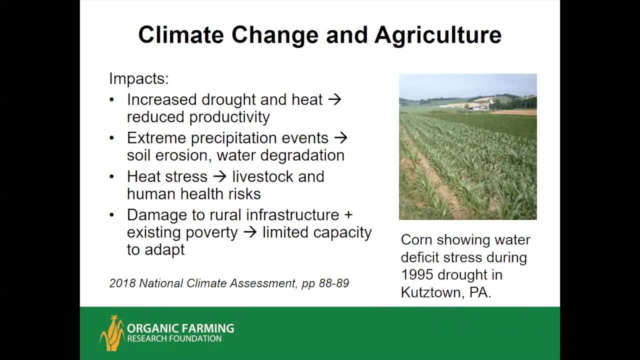 sometimes aggravated by heat or extremely heavy rainfalls, and all of the adverse effects on crop and soil that that can entail. Heat stress can impact livestock and the human health in rural communities, and there's also significant impact on the environment. So we're going to talk a little. 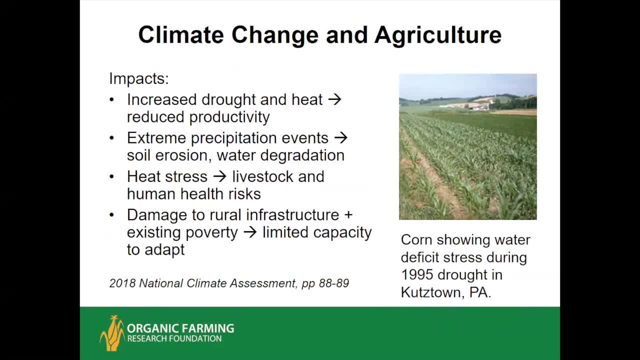 bit about what climate change is really and how it affects our economy. So let's start with the general picture here. The climate change and the impacts we're seeing in this year are significant and damage to rural infrastructure. This is an example here. Remember that photograph right there. 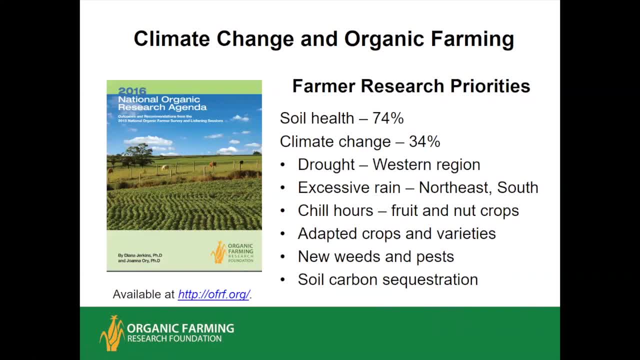 that's showing some pretty severely drought stressed corn. This will come up again in a few minutes. Okay, Before I go on, I wanted to mention that in California the State Department's Agricultural Secretary, Karen Ross. she noted something that was really important to mention and 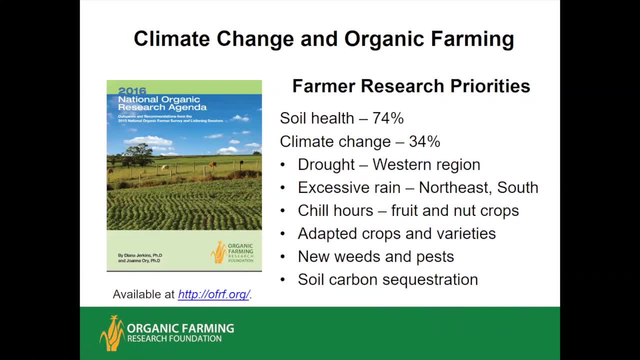 this is something that was really important in the state and it's something that was really important to mention. and it's something that was really important to mention. It was a really important point in the state and a lot of the some really significant impacts already in her state noted that up to half a million acres have. 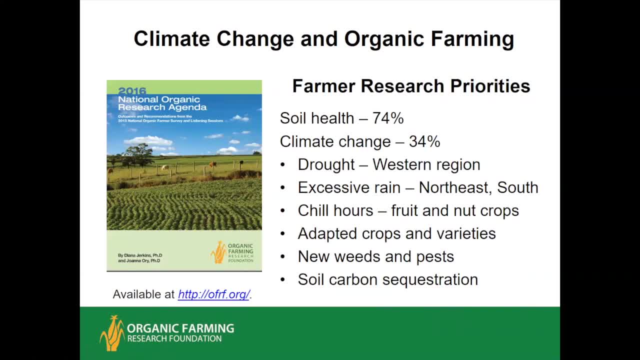 been fallowed some years because of drought over the past decade and also that disruption of normal chilling, normal cold periods in the winter has made it more difficult for orchard and vineyard crops to develop and mature normally. So this next slide we're looking at the results of a survey. 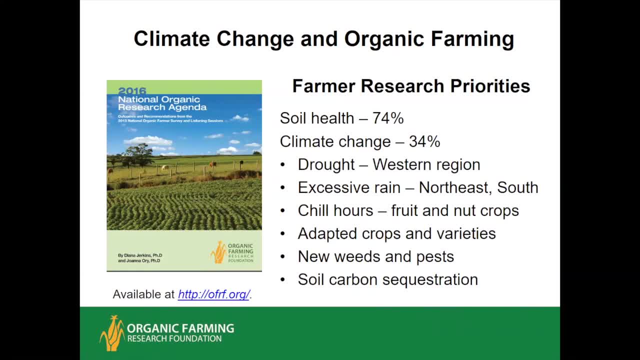 of farmer research priorities conducted by the Organic Farming Research Foundation. It's a survey of which 1,403 organic farmers across the United States participated, and the top research priority was soil health. Nearly three quarters of respondents considered that to be a high priority. 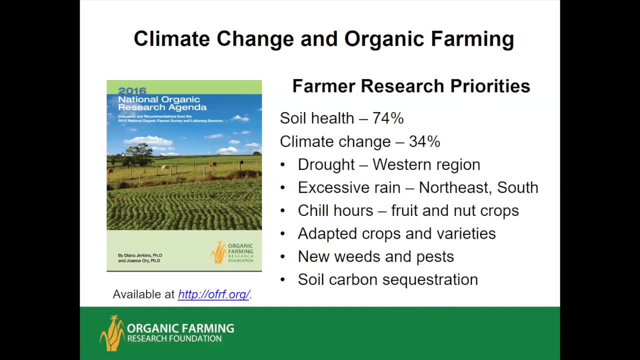 Now, climate change looks like not that high a priority from their viewpoint, because 34 percent rated it as high. However, an additional 42 percent rated it as a medium priority, and there were a few farmers that made comments such as- and this is a quote from the report that climate change is about to put me out. 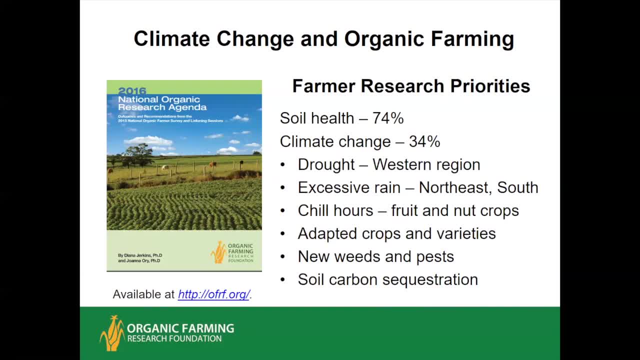 of business, So it's really beginning to impact some farmers. The leading impacts were drought in the western region, excessive rainfall in other regions, especially the northeast and the south, and now we're seeing some of it in the midwest with the flooding, The issue with chill hours and 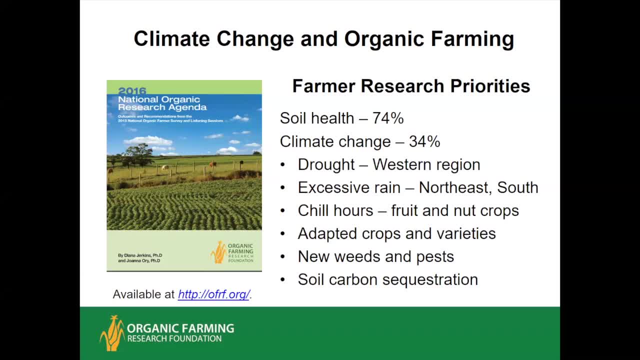 fruit and nut crops came up. Also, as the climate zones shift, the weeds will spread north, or new weeds or pests will crop up at a given location. In addition to researching these challenges and how to adapt to them, farmers are interested in identifying crops that are better adapted to the shifting conditions and organic 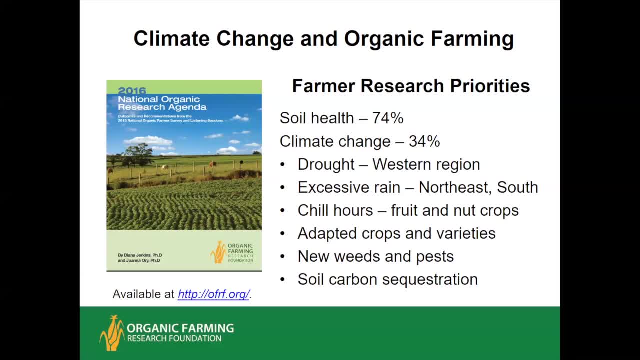 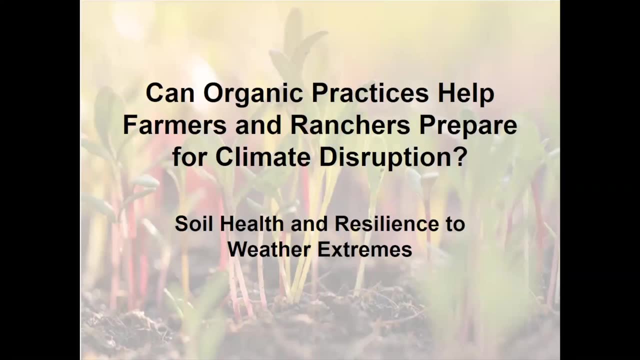 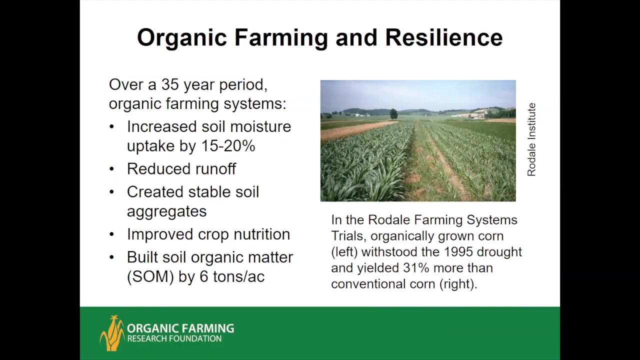 production systems. and also, can farmers actually receive some remuneration for the ecosystem service of soil carbon sequestration? Okay, so well. can organic practices help farmers and ranches prepare? How can it build resilience? Remember that picture? Well, that's this whole field, That's the whole story. On the left is one of. 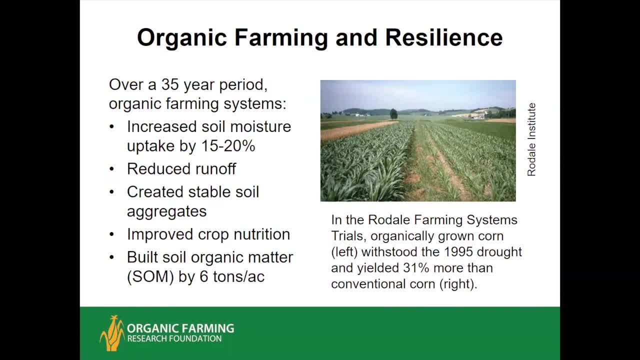 the two organic systems that the Rodale Long-Term Farming Systems trial is evaluating. On the right there's the R external organic system. The R external organic system is an independent system that now benefits the soil and carbon sequestration. So if you're in the field and your system is in a poor condition, knowing that your plants don't grow well, you 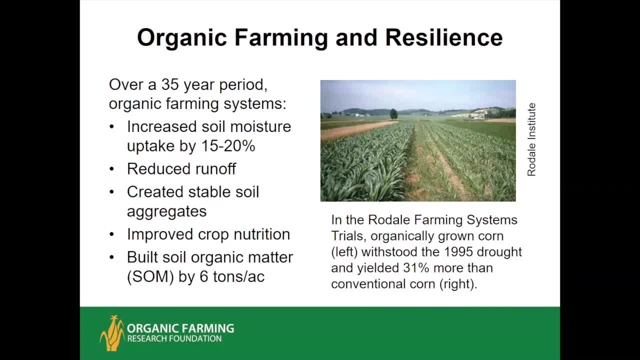 is a conventional corn-soy rotation with conventional inputs. On the left that corn is in a somewhat more complex and more integrated rotation with the use of legumes and or animal manure as the primary source of fertility. In most years the two systems have been giving. 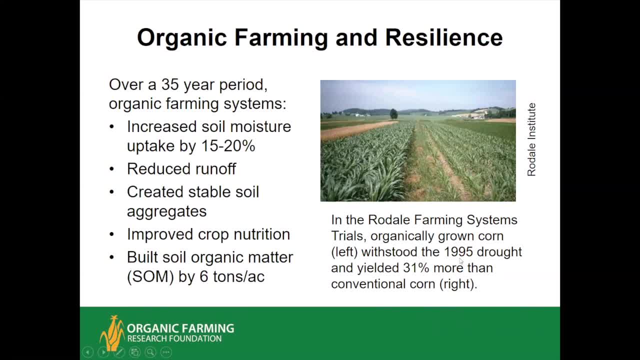 approximately equal yields, but during a moderately severe drought in 1995, at one point during the worst of the dry spell, we saw this difference in the appearance of the crop and at the end of the year the organic yield was 31% higher. The reasons for this were improved soil moisture. 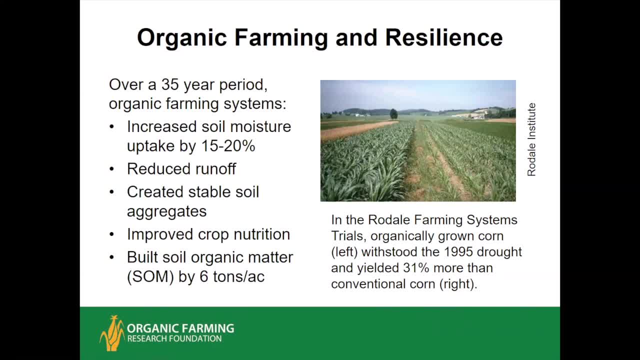 uptake. during a rainfall, This organically managed soil absorbed the water better, There was less runoff. It had more stable aggregates. Overall crop nutrition was better and over the course of about 20 years of this trial, organic matter increased by about six tons per acre, so half. 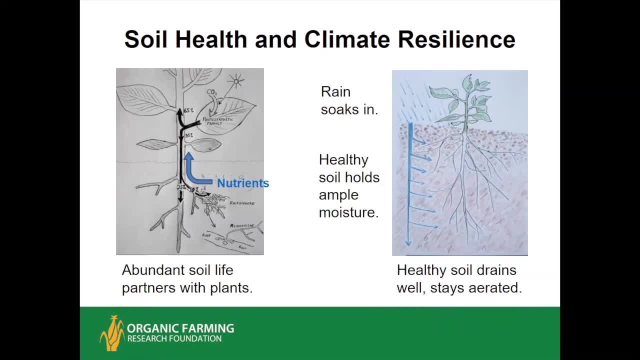 of that is carbon. That's three tons per acre of carbon that was accrued. Here's just some of the mechanisms by which really healthy soil will improve resilience to the weather extremes associated with climate shift. In a healthy soil you have an active partnership between the plant roots and various 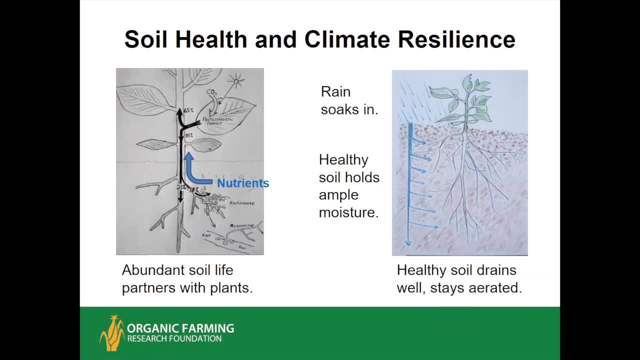 beneficial organisms living in the rhizosphere or close to the root, where all the goodies that the plant is releasing into the soil is nourishing That soil life, and especially organisms like mycorrhizal fungi and various bacteria that facilitate nitrogen metabolism and uptake, is helping the plant to get the nutrients it needs. Also, when you 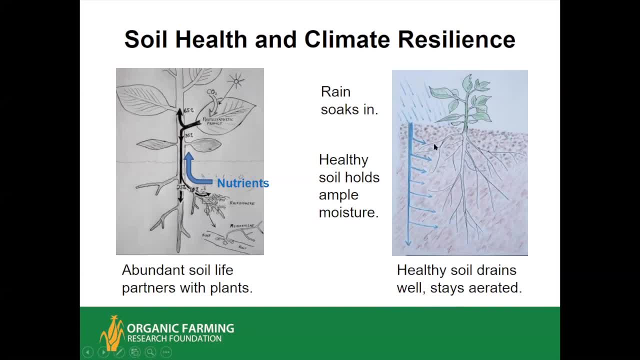 have a really healthy soil: an open profile, good structure. when the rain comes down excessively hard, it soaks in more easily, The soil drains out more quickly to restore aeration and the total plant availability is very, very high. So if you have a really healthy soil, you have a really 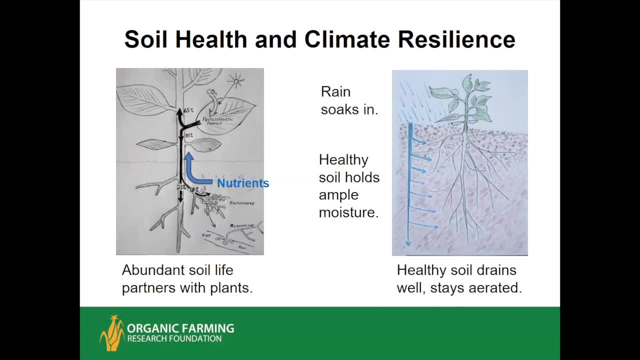 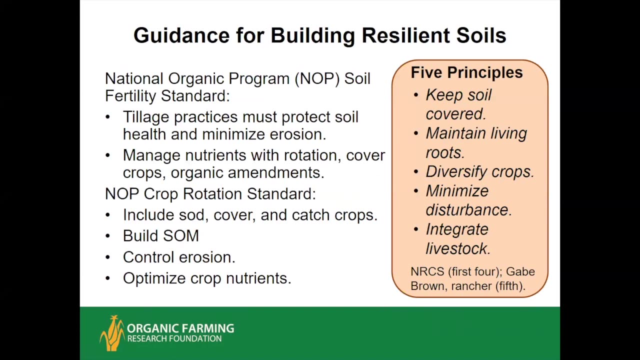 stable moisture holding capacity is better, so that when the dry spell hits the plant has more reserves And also in a healthy soil the plant is able to form a really extensive root system, which is an important part of resilience. So both the National Organic Program, which certifies organic growers, and the Natural 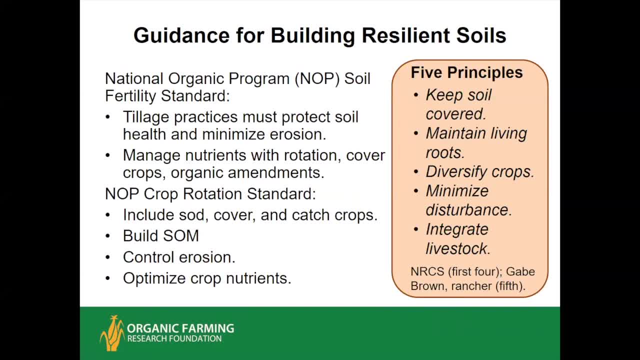 Resources Conservation Service have really offered some excellent guidelines for building resilient soil. So if you have a really healthy soil, you have a really extensive root system, which is an important part of resilience. So if you have a really healthy soil, you can definitely 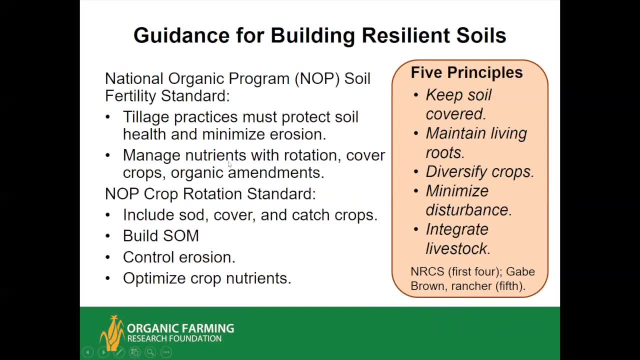 transition it when it gets trough the bottom of your contamination and getting rid of the rock, But making sure that you have the resources that are necessary to get rid of the rocks and to get rid of the zoys. the NOP requires that tillage practices have to. 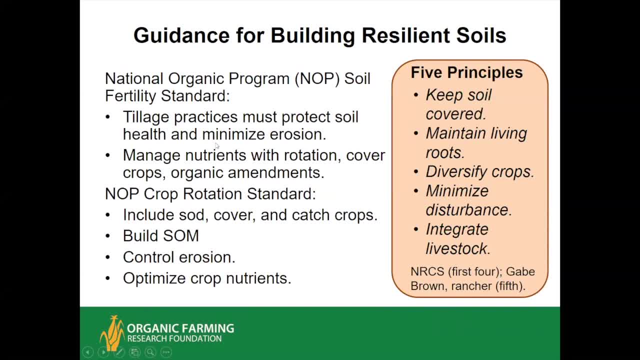 maintain- at least maintain- the current soil health and minimize erosion. nutrient management rotation cover crops and organic amendments. The crop rotation standard goes into some more details about how to build a truly sustainable rotation. I've listed five principles here. the first four, which we will go into in more depth later, were developed by the Actual Resources. 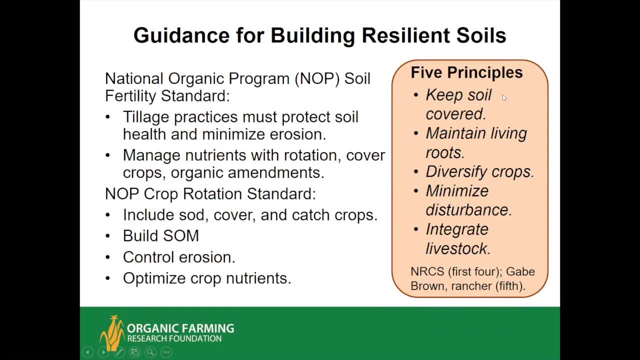 Conservation Service and the Nationalarest And the special program is built around higher allora so that all the crippling and interproys can get water solutions and most of the陰brom breathable later were developed by the Natural Resources Conservation Service. Five principles of soil: 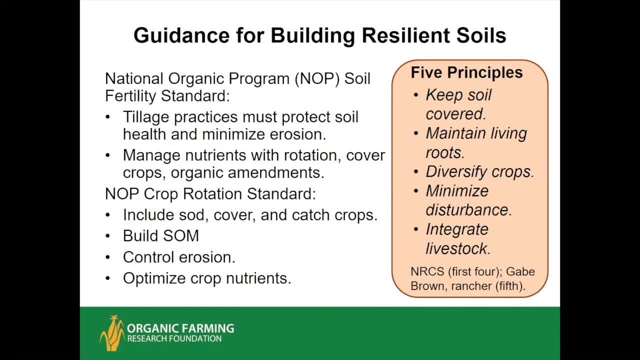 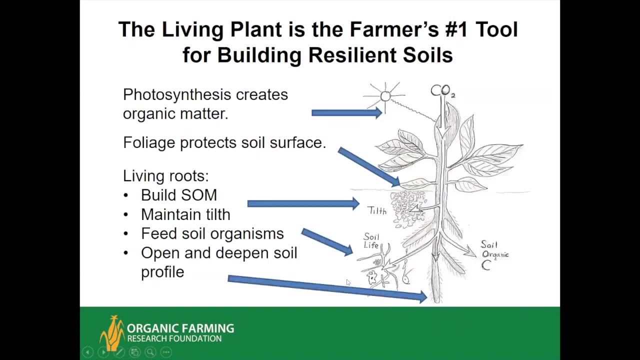 health, keeping the soil covered, maintaining living roots, diversifying crops and minimizing disturbance. And then North Dakota rancher Gabe Brown has added a fifth principle, which is to integrate livestock into the system, as this further improves both overall resilience and nutrient cycling and carbon sequestration. So I just wanted to point out that the living plant 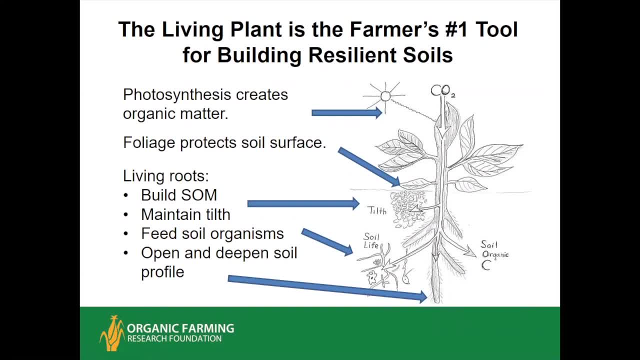 is really the number one tool for building soil resilience. This is how nature has done it since plants first evolved to make their life on the land and not just in the sea. The photosynthesis is the origin of all organic matter. essentially Living plant foliage protects. 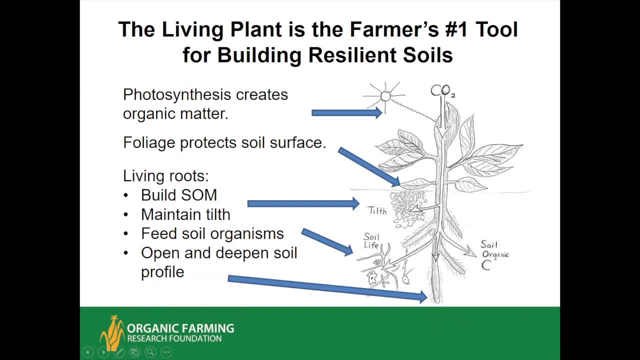 the soil surface and the content of the soil, So it's a very important tool for building soil resilience. And then North Dakota rancher Gabe Brown has added a fifth principle, which is to integrate livestock into the system, understanding living roots, diversifying crops and stimulating 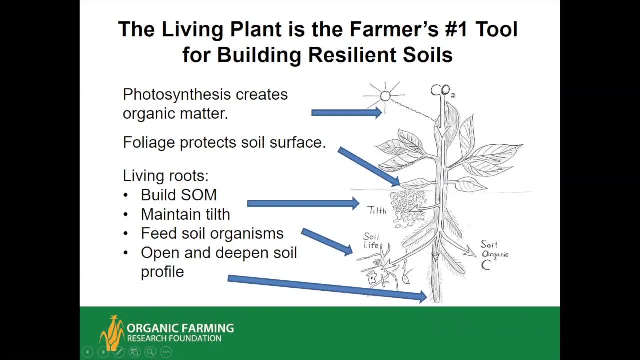 llevies and keeping them in theiroga dens. So those are the five principles of living, which is interacting with soil systems to help有 acre tulee and largely, thankfully, take on the into the subscale environment. So if you're interested in details about those late smile, 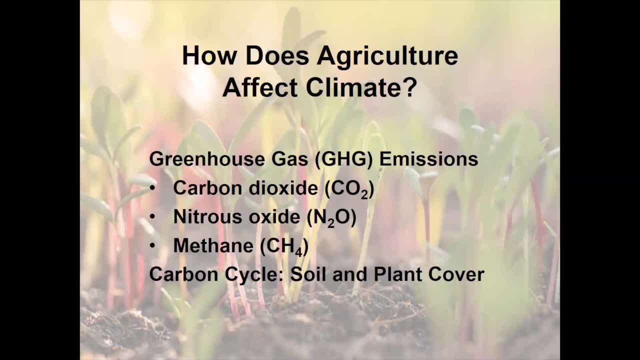 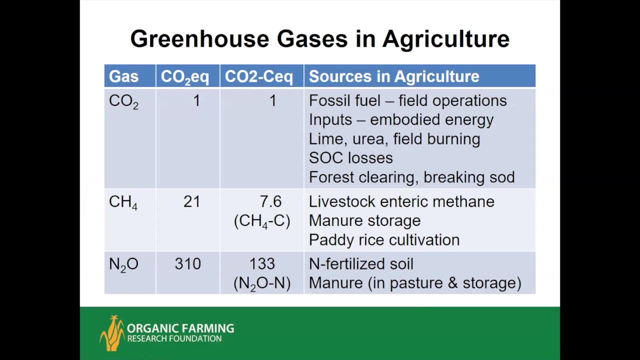 years at the region and the local level. you can very much click across here smiling to. Let's go to another slide. It's sort of a little fried down, doesn't ask you. It's much better over the roof. One thing to remember about the three main greenhouse gases in agriculture: 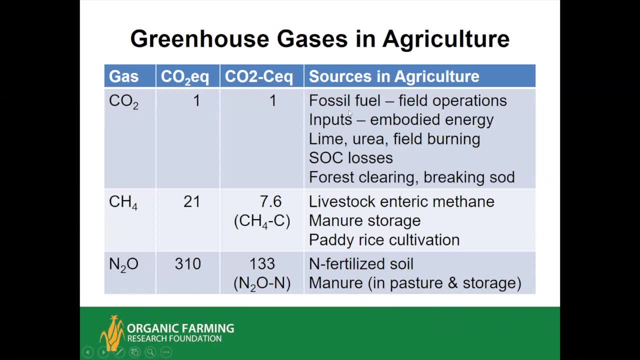 carbon dioxide. this is emitted during fossil fuel use and field operations, and the embodied energy and inputs. Small but significant contributions from application of lime. You put lime on an acidic soil. the carbonate turns to CO2, and that neutralizes acidity Urea. 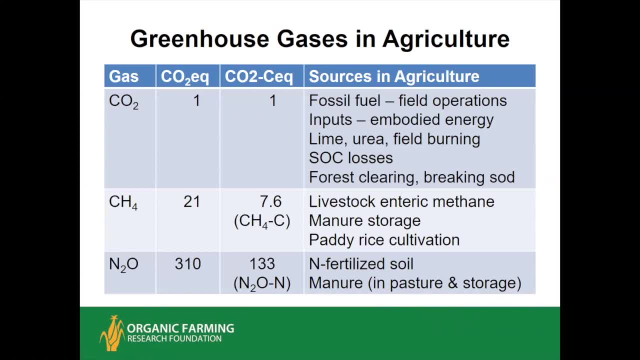 as the nitrogen is consumed, lets the liquid loose Field burning. of course, A big one is soil organic carbon losses. Now there's a net loss of organic matter- We'll get to that a little bit more later- And also whenever forest clearing or breaking of either native sod or pasture. 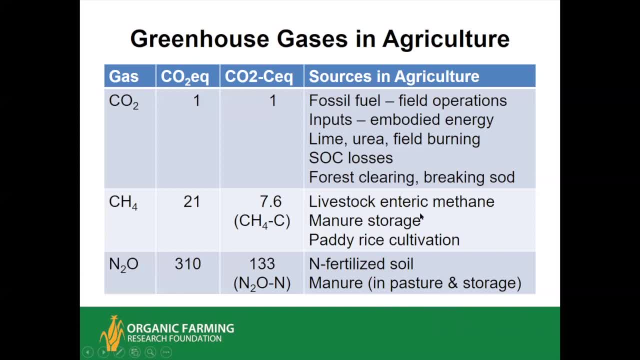 that will accelerate carbon losses. The other two gases are methane and nitrous oxide. Now the methane is about 21 times as potent as carbon dioxide in terms of 100-year global warming potential. Nitrous oxide is 310 times Now. when we look at this on an elemental basis- and I will be 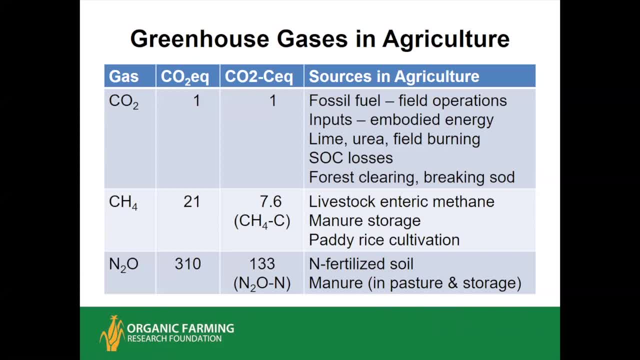 talking elemental basis, because we'll be talking about carbon sequestration rather than carbon dioxide per se. So, keeping carbon dioxide carbon as one, then every pound of carbon released as methane has 7.6 times the impact of that same atom of carbon released as carbon dioxide. 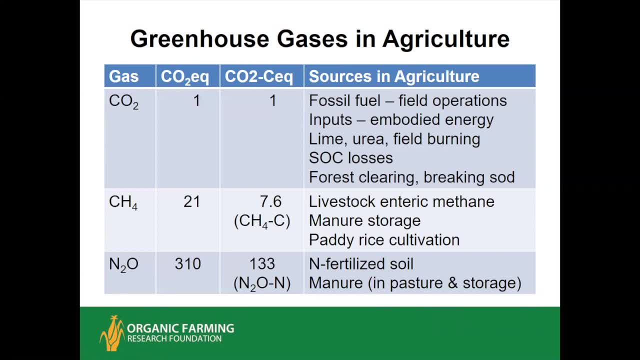 Every pound of nitrogen released as nitrous oxide has 133 times, So that is a very serious concern there, And the sources of nitrous oxide are primarily soil that has been fertilized with nitrogen, either synthetic nitrogen or organic sources. Manure during storage can also release nitrogen. 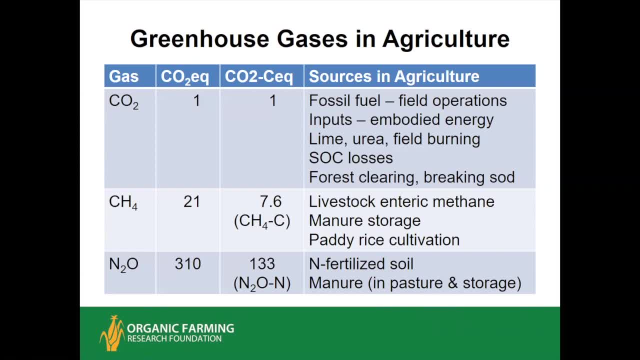 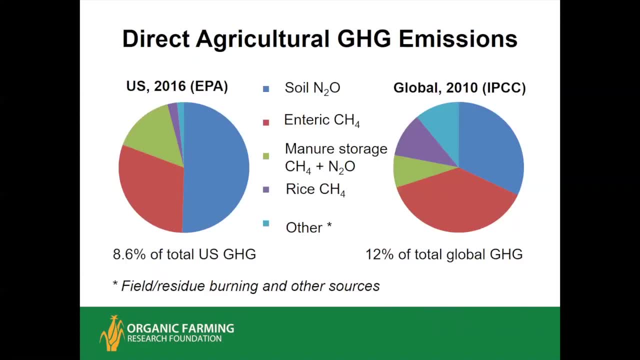 and also when it's deposited in pasture- Methane. one of the biggest ones is livestock enteric methane, manure storage and then patio. So we're going to start with what's called direct agricultural greenhouse gas emissions. This actually does not include the carbon dioxide that comes out of the tractor's tailpipe, or is. 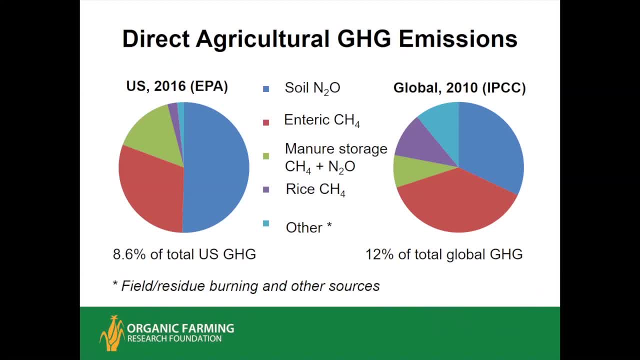 embodied in the nitrogen fertilizer and other inputs. Those are subsumed under other categories of emissions, ie transportation, energy consumption and industrial process Within the US in 2016,, the Environmental Protection Agency estimated that soil nitrous oxide accounted for. 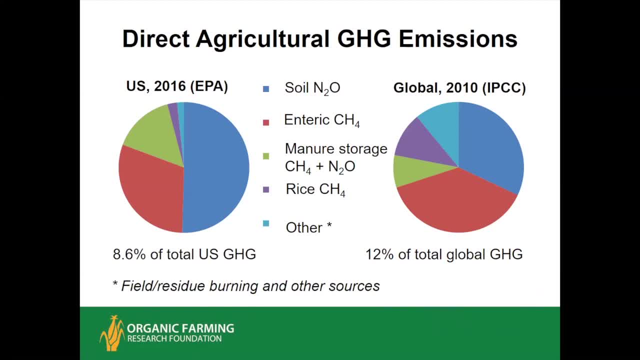 half of direct emissions. The second biggest slice was enteric methane emitted by the livestock on the land, and the third is manure storage, And this is 8.6% of the total US greenhouse gas footprint. So you say, oh well, agriculture is a relatively minor source. 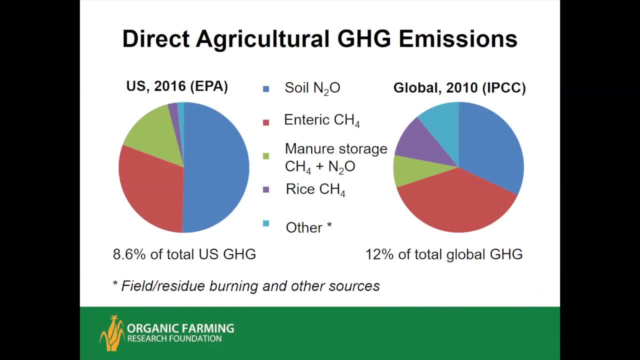 Yes in a way, but also we must remember if there's a way to make agriculture carbon neutral, that's 8.6% reduction in our emissions And that's a significant step to what we need to get. When you look globally, the soil nitrogen is not as large as a proportion. 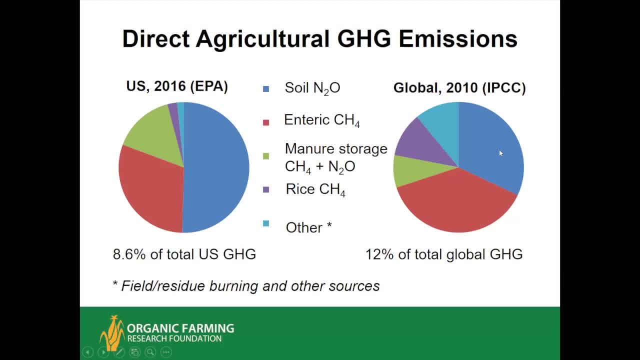 and that's because not as much fertilizer is used in developing countries as in the US. Rice is a much larger slice because it is a staple in the diet of most of Asia and other parts of the world, not so much in this country. Manure storage is less of a smaller part of the pie. 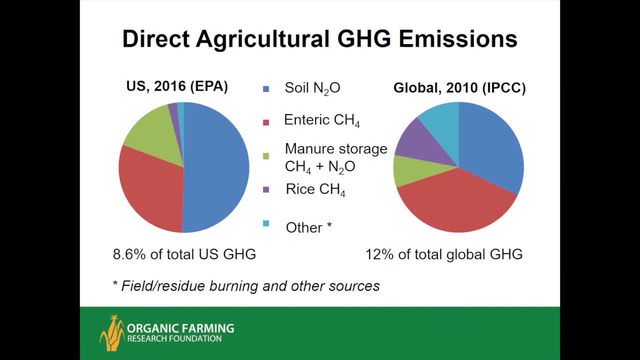 And then the enteric is relatively a little bit larger. it's because the soil nitrogen is less And globally agriculture direct is about 12% and that's mostly because other countries don't burn as much fossil fuel And that's because they don't use as much fossil fuel tooling around in their vehicles etc. as they do on average in the United States. 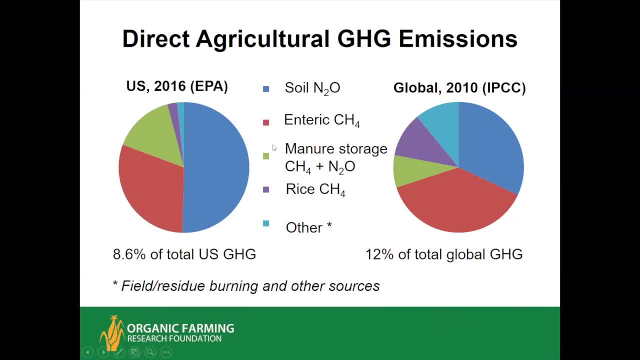 One thing to note is that this category- manure storage- and especially the methane part, has been going up in the United States because of the increased use of manure lagoons. liquid manure storage has gone up and that has been the main driver in a significant increase over the last 25 years in our direct agricultural emissions. 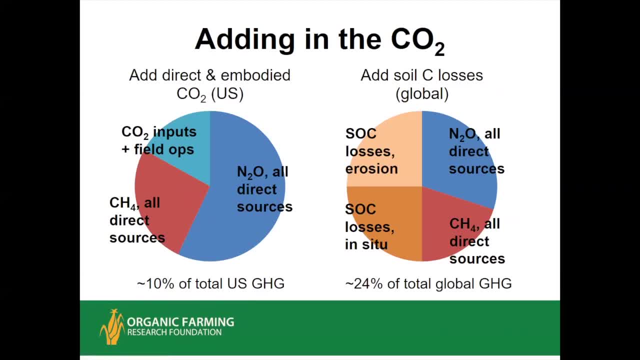 Okay, So let's add in the carbon dioxide. Well, with every time we talk about reducing greenhouse footprint of agriculture, the first thought that often comes to mind is: what about the CO2.? Interestingly enough, even though nitrogen fertilizer is very energy intensive to make, when we add the CO2 from inputs and from field operations, 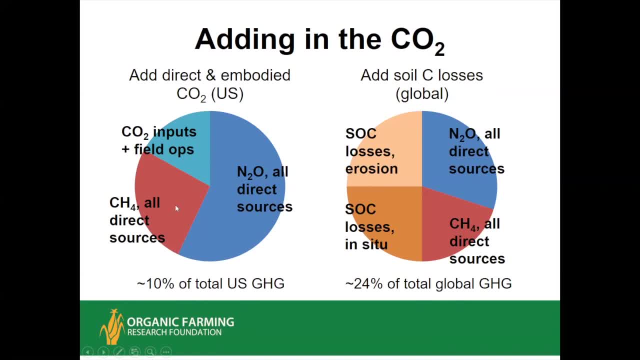 that's only 17% of the pie. The rest of it is all the sources, methane and all of the nitrous. and remember, most of this is from the soil, a little bit from manure and then, in a global analysis, when we add in all soil, 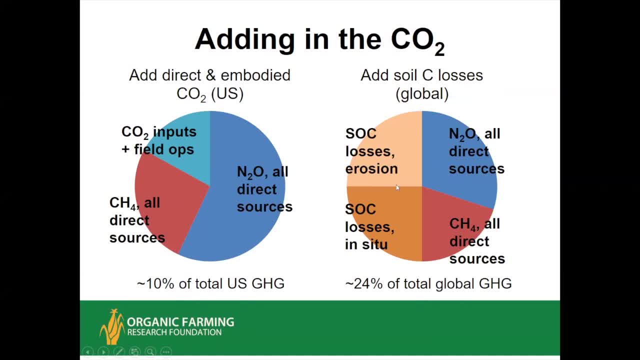 carbon losses. they make up just about half of the global agricultural footprint and of that half, 25% is directly related to erosion when the soil washes or blows away of organic matter. in other words, carbon is selectively removed. there's more car, is more organic matter and clay in eroded 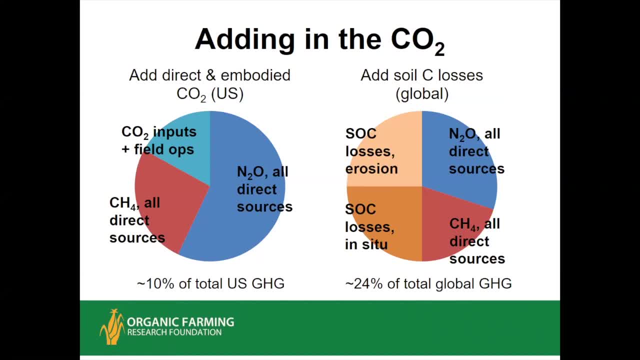 sediments and windblown dust and there is in the bulk soil. and as and when that carbon blows away, it either oxidizes or becomes submerged in the runoff- if it runs off into a river and that actually turns into methane at that organic water. and then there's also the long-term. 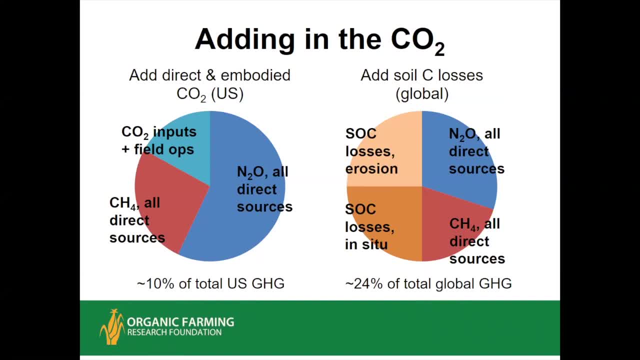 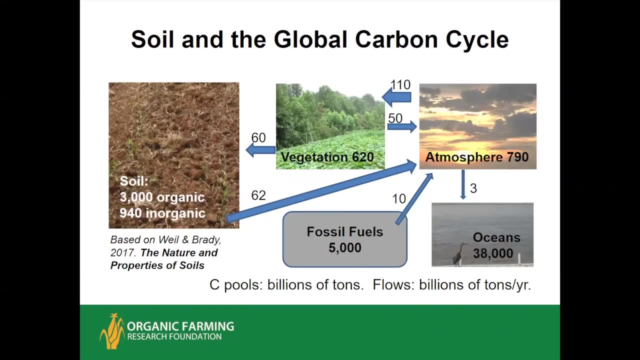 losses in situ. there is still a net loss in situ from soil organic matter degradation. when this is all added together, the total global agricultural footprint is close to one-quarter of the total human greenhouse gas footprint. okay, sorry about that. all right. some interesting thing to look at here is the 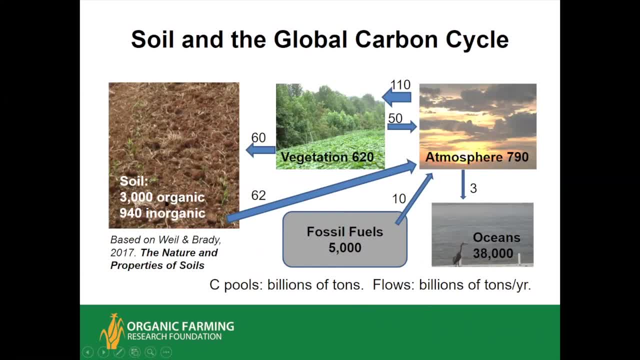 soils role in the global carbon cycle. most recent estimate is that the soil, the world soils, contain 3,000 million tons of organic carbon. excuse me, 3,000 billion tons or 3 trillion, however you want to cut it, but anyways it's 3,000 gigatons and another 940 gigatons of. 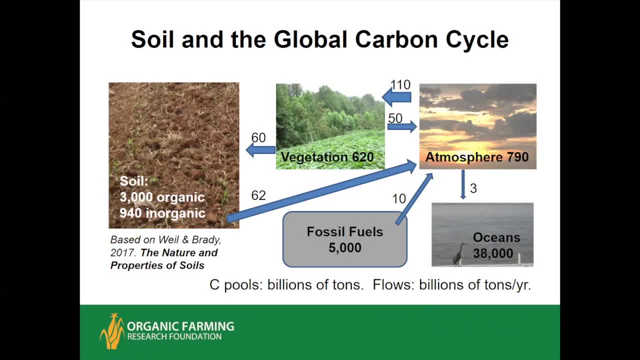 inorganic carbon or carbonate carbon compare that with the world's vegetable �� it's only 620 and in our atmosphere although this is a big concern has been going up it's still 790 which is less than what's in the soil so a few things to note about the dynamics across the big driver of climate change globally 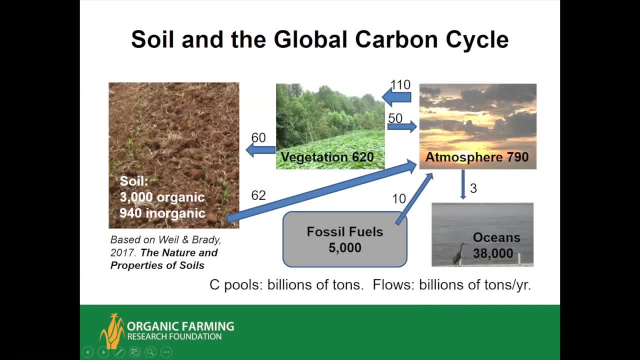 is its use of fossil fuels, putting ten units into the atmosphere, at which the oceans are maybe absorbing 3 billion tons per year. these are annual flows, whereas a vegetation takes 110 tons per year. whereas a vegetation takes 110 tons per year. Whether it's a record or matters, it's more than a record or a Arguaboy can't transfer as much carbon gas from a single source to another. um, as we move into the next slide, which is presently, we're looking at in-person buildings. we're looking at a lot of the climate change, of a climate change, and we also are interested in the environmental issues of class and nature and how we're able to. 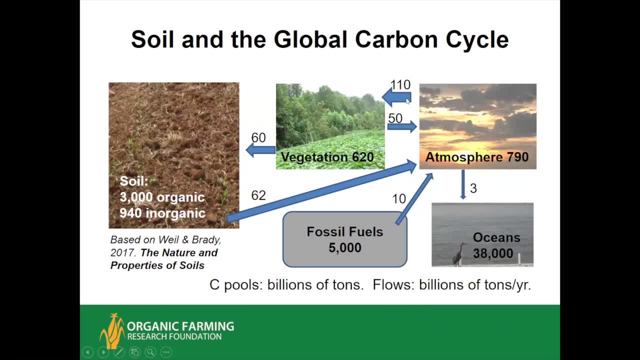 billion tons out of the atmosphere and respires about half of it back, puts half of it back in the soil And that imbalance, that half of the pie that was contributed by soil organic losses, that's represented here by the fact that this is about 60 gigatons and this is 62.. 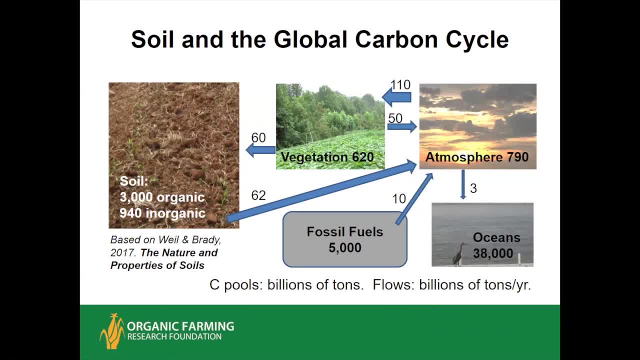 The soil is losing just a little bit more every year than it is taking back in. Okay, so what this shows us is that the most important practical means for humanity to get carbon out of the atmosphere is through photosynthesis and to try to get the soil 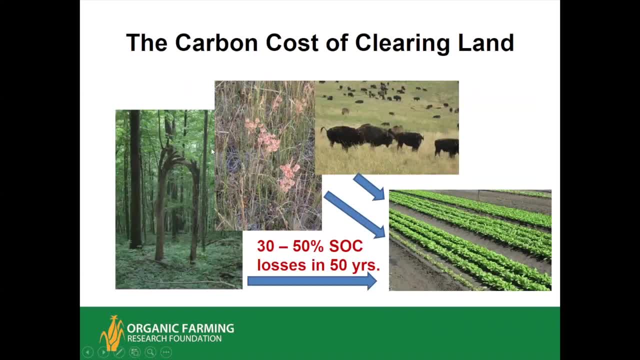 to be absorbing more than it is releasing. One thing to keep in mind is that clearing land has a terrible carbon cost. Typically, you turn a forest or a prairie into a forest and you're going to have a lot of carbon, And so if you're going to have a lot of 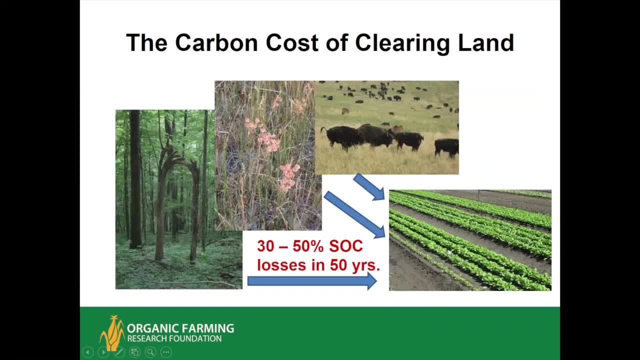 carbon, you're going to have a lot of carbon, And so if you're going to have a lot of carbon. even well-managed, organically managed cropland- if you're killing it once a year even you can expect a 30 to 50 percent loss of the soil organic carbon stock in the top soil. 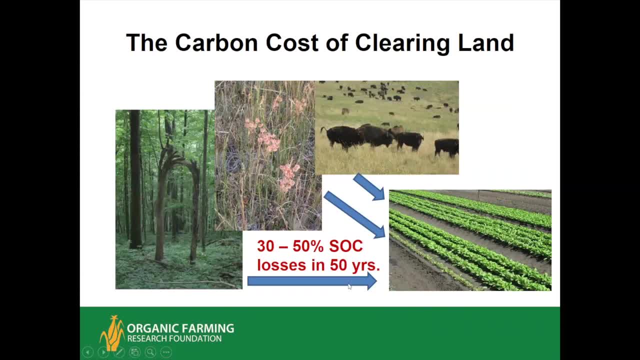 in the A horizon over about 50 years, And sometimes it can be much more severe than that. In fact, it's interesting to note that, historically, the clearing of land is responsible for about 30 percent of the excess human-caused greenhouse gas emissions, And so, if you're 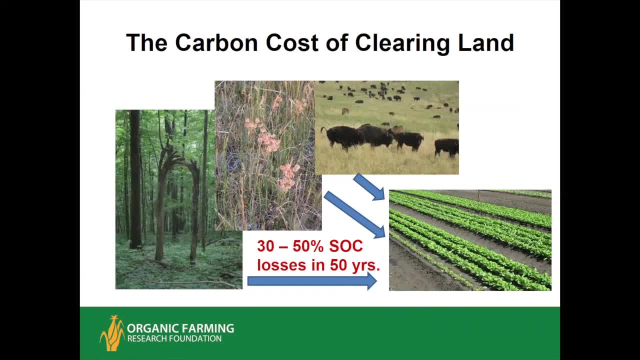 going to have a forest, you're going to have about 30 percent of the excess human-caused greenhouse gas emissions since 1750.. And since the dawn of agriculture, the loss of biomass and the loss of soil, organic carbon together represent about 500 billion tons of carbon that has been turned into CO2.. 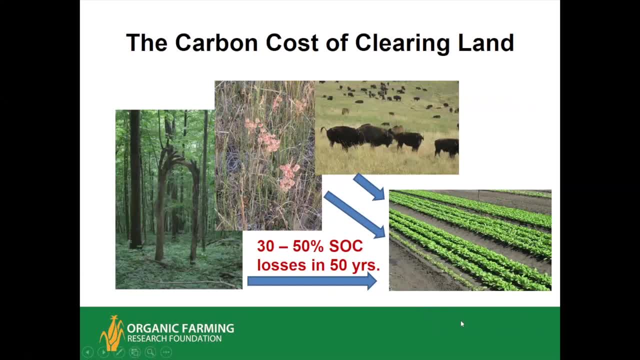 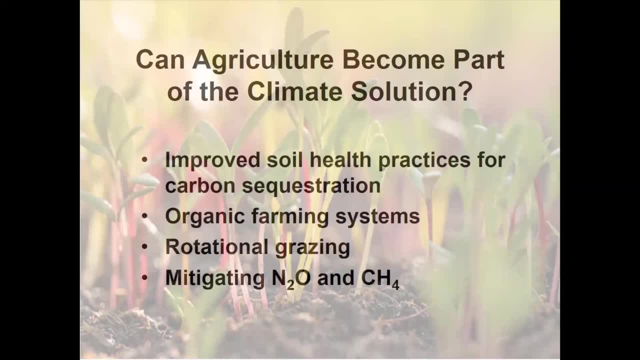 In other words, that's about 34 years worth of um CO2 emissions- greenhouse gas emissions- at today's rates. So how can agriculture become part of the solution? We'll look at three types of solutions. How can agriculture become part of the solution? We'll look at three types of solutions. One is if we're going to have a forest. 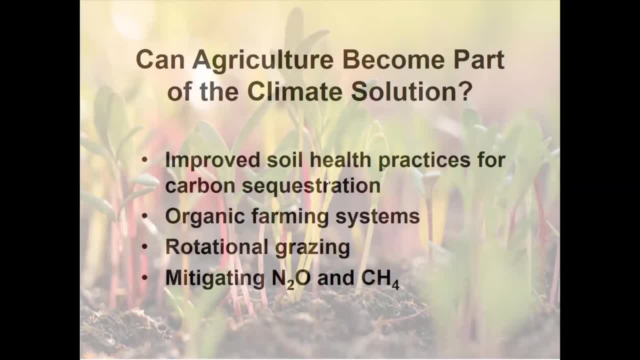 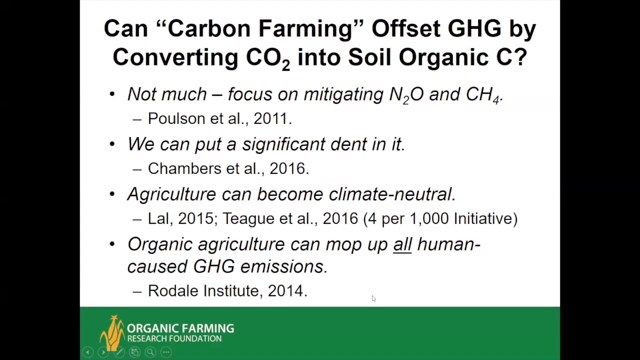 look at several ways that this can happen: Improved soil health, practices for carbon sequestration, organic farming systems, rotational grazing and strategies to mitigate the nitrous oxide and the methane. We've heard a lot about carbon farming. Can it really offset the greenhouse gas emissions that humanity is creating? 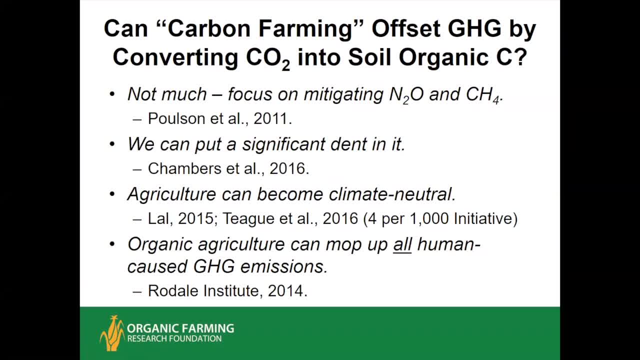 that is causing this climate crisis that we're facing. Can we convert some of this excess CO2 into soil organic carbon? Well, the research is very greatly in their opinions on this, And you'll find the details of these references in the presentation notes. 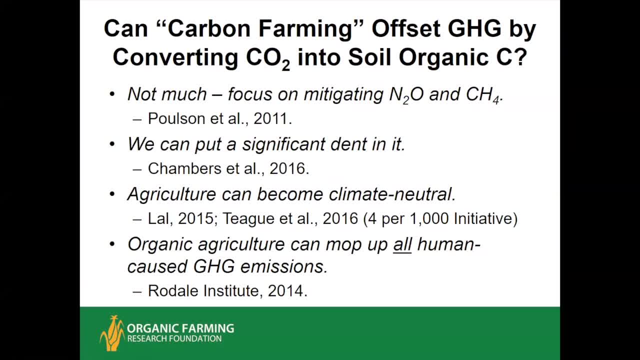 I won't have time to go into the great detail, but some scientists are saying we really can't get that much done in terms of direct sequestration. You better focus on mitigating this nitrous oxide and this methane Because, as you saw, 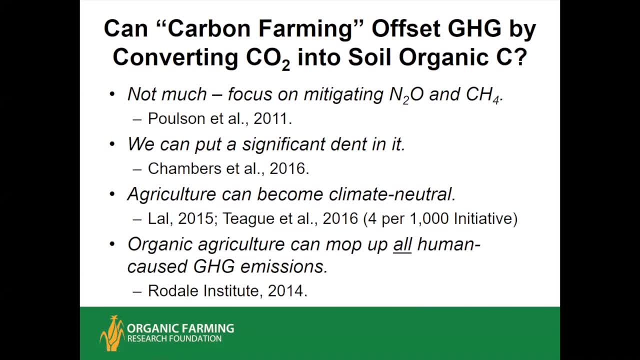 those are the two major sources of direct agricultural emissions. Others- this is based on the NRCS conservation practices and estimates of their capacity to sequester carbon. Basically, we could put a significant dent in agricultural emissions, maybe even offset most of the direct emissions. 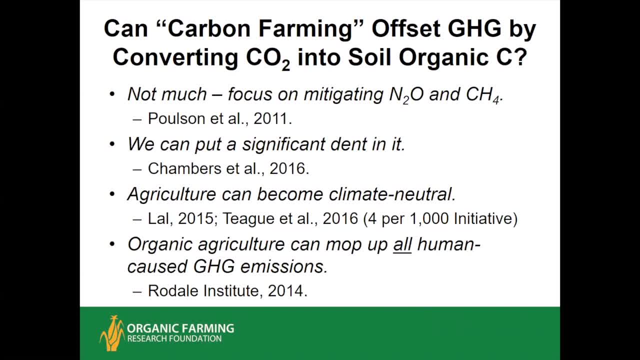 There are others who have been a little bit more: Dr Ratan Lal, who's one of the leaders in in agriculture and climate and soil health, is at Ohio State University, I believe, and Dr Richard Teagan at Texas A&M. 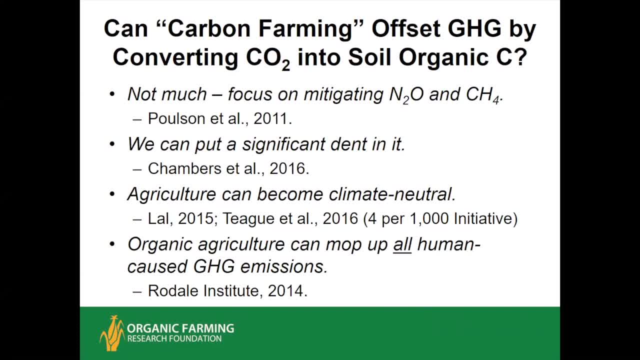 They have published a number of articles in the Journal of Soil and Water Conservation that suggests that if we implement best organic or sustainable practices on all of the world's agricultural lands, we could probably make agriculture fully agriculture, climate neutral. And in fact, at the December 2015 Paris meeting of the Conference of Parties, 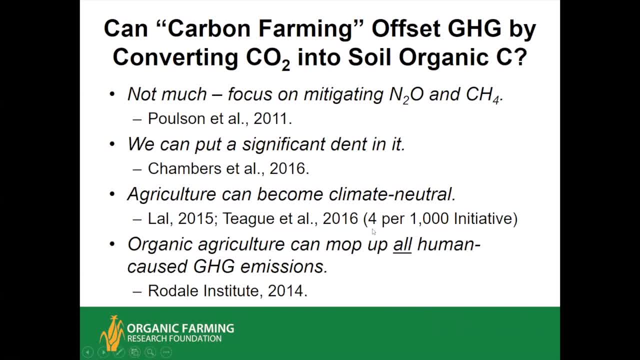 this is related to the climate agreement. there was a four per thousand initiative launched And the idea was to increase the world's total soil organic carbon in the top 16 inches of the soil profile by about 0.4% per year. So you're taking that probably about half of that 3,000,. 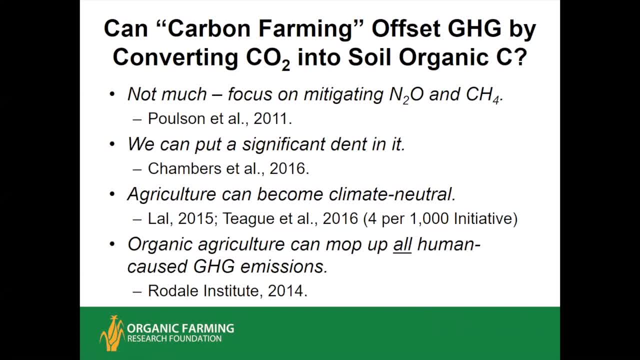 gigatons and then adding increasing it by 0.4% per year at that level will just about achieve this degree of mitigation. And there have been some other researchers who have been really excited about the results of organic systems over conventional, as the Rodale Institute has conducted a long term farming systems trial. 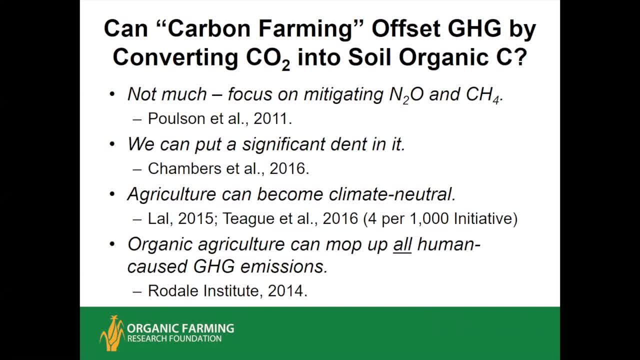 And they have somehow concluded that if we apply management, rotational management tests of rotational grazing to all the grazing lands and organic, integrated organic production systems of all cropland, that we could pretty much clean up the whole human greenhouse gas footprint. So that's the range of opinions. 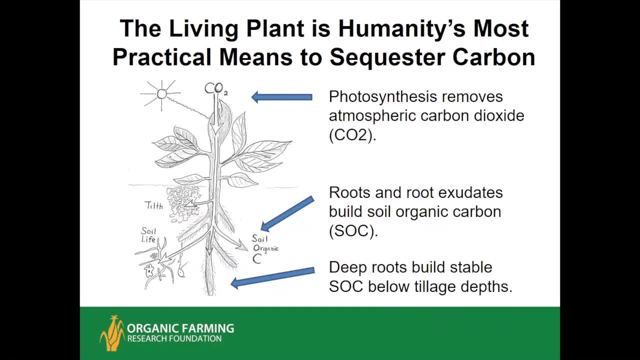 Yet I'm back to the living plant. I think it's the best thing that we've ever been given on this planet, because it is the way that carbon moves out of the atmosphere back into the Earth. That's how the fossil fuels got there the first time, and plants are different today, so we may not do it exactly the same way it did today, but that's the way it has become the way it has become. 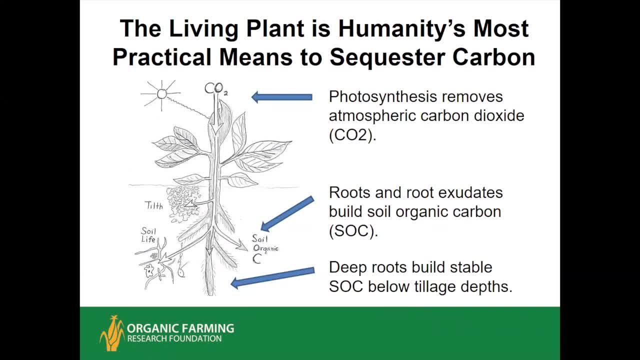 So we're pretty much back to the fossil fuel point. So we're pretty much back to the fossil fuel point. So we're pretty much back to the fossil fuel point, the same way. but we can certainly facilitate getting a lot of carbon down back into the soil. 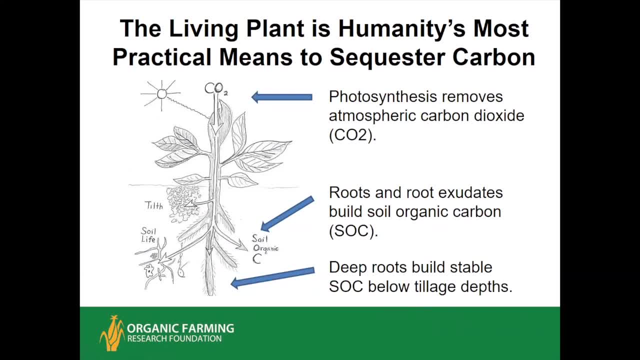 And two things are happening. One is that this constant biological process that I've talked about earlier between the roots and the soil life is continually building and rebuilding soil, organic carbon near the topsoil, And the other thing is that the deeper roots are putting soil 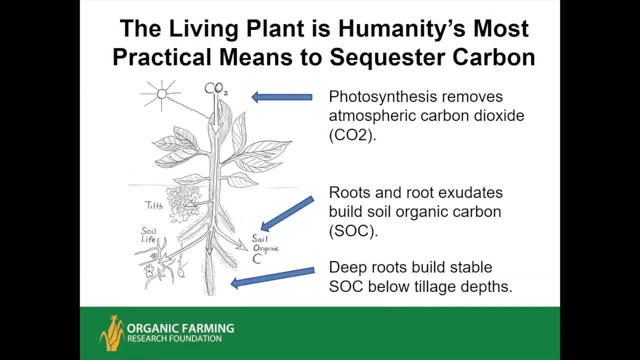 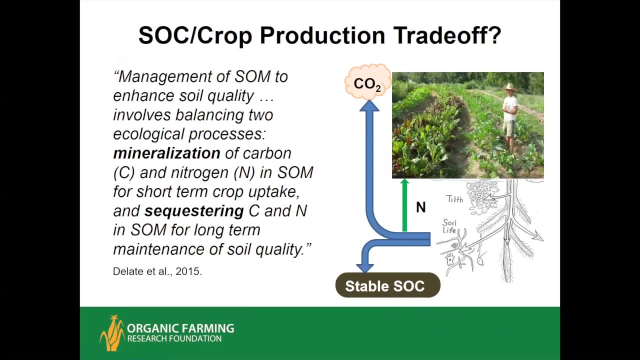 organic building soil, organic carbon below the depth that even the deepest turnplow is going to reach. So this deep carbon is not as prone to loss from a tillage event. Okay, and then I'm sure some of the farmers on the call are wondering: well, what about the trade-off? I have to mobilize. 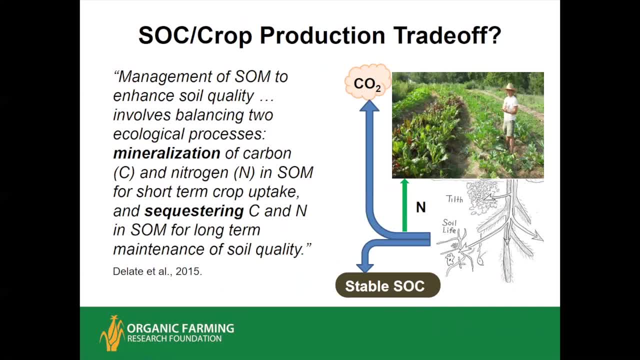 organic matter to nourish the crop. The process by which the soil life feeds the crop does entail burning some organic matter, some of the either the fresh residues or the active organic matter. to release it Is carbon dioxide, releasing nitrogen and other nutrients directly to the plants right there in. 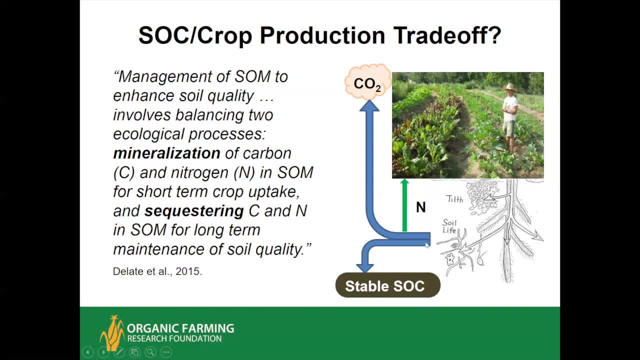 the root zone. Yes, that's happening, And at the same time, some of the fresh organic residues are being converted to stable organic matter by those same organisms. For example, when organisms die, their remains often adhere tightly to the surface of clay and silt particles in the soil. 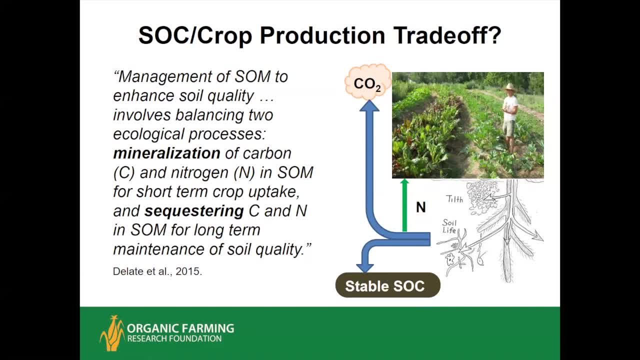 And that is a very stable form of soil, organic carbon. It used to be called the clay complex. In any case, sustainable agriculture depends on both of these processes. You got to have mineralization to feed your crops. You got to have good crop yields to stay in business. 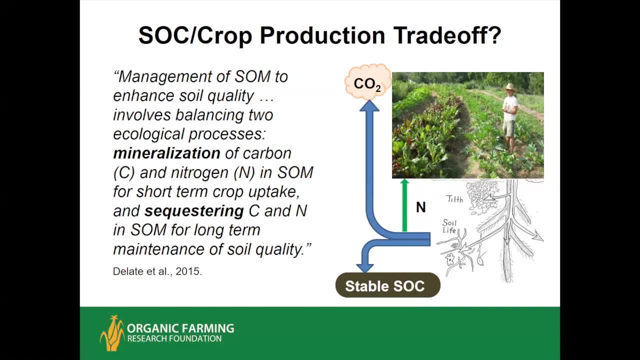 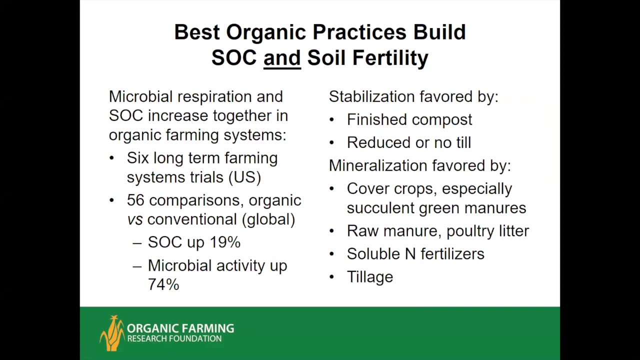 And we need agriculture, not only to feed ourselves but to keep the soil healthy, And, at the same time, we need to have those long-term soil carbon sequestration. Okay, so what are some best organic practices to build Soil, organic carbon and soil fertility? Well, the good news is that it's not as severe a trade-off. 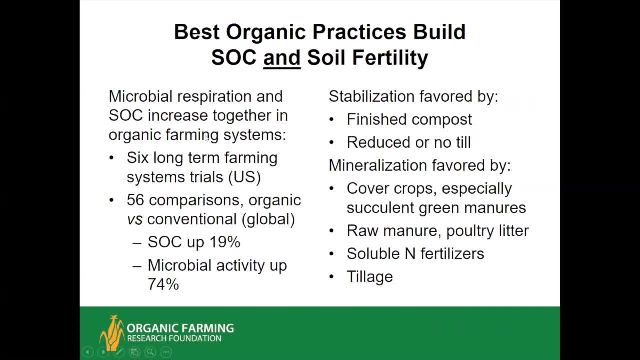 as it sounds like, because the processes and practices that tend to build up microbial respiration and microbial activity also do tend to increase long-term soil organic carbon. There's a number of meta-analyses or a review of multiple studies that have shown that these processes are not as severe as it sounds like, because the processes and practices that tend to build up microbial respiration and microbial activity also do tend to increase long-term soil organic carbon. 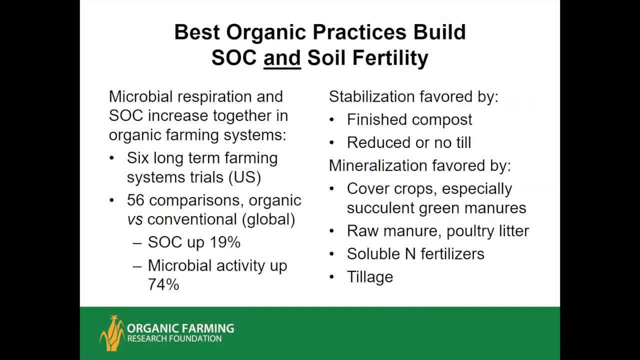 There's a number of meta-analyses or a review of multiple studies that have shown that these processes do tend to increase long-term soil organic carbon. There was one analysis that did 56 different studies across the world. On average, the soil organic carbon was up 19% of the organic citizens, while microbial activity increased by some 74%. 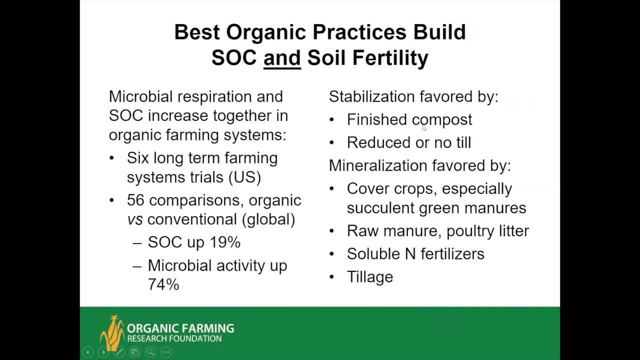 Now there are some processes that favor stabilization. Finished compost helps to anchor carbon, as does biochar, which is an amendment that's become popular these days. There are some concerns also with biochar manufacturers, so I'm not going to be emphasizing that in this talk. 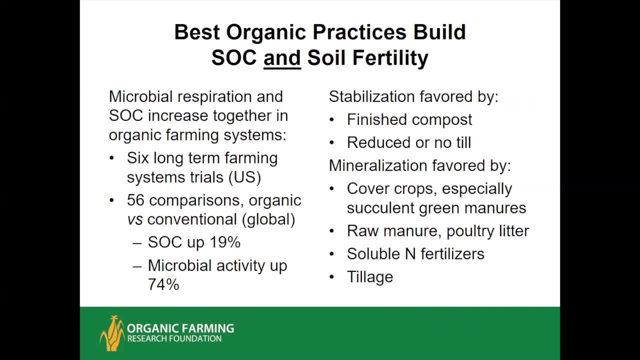 or reduced or no tillage. the less you till, the more the organic matter tends to remain stable. Mineralization, which is the process by which crops are fed, are favored by succulent green manure, like a young cover crop that's tilled into the soil. 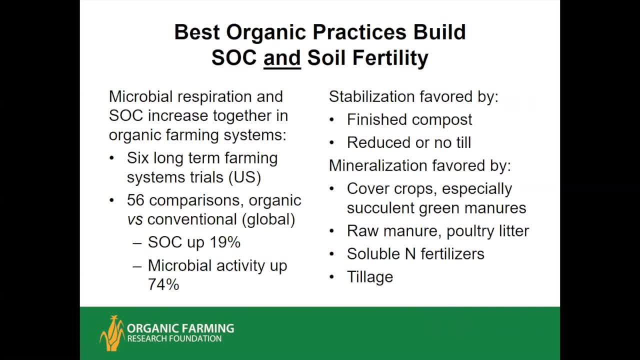 Raw manure poultry litter. soluble nitrogen fertilizers. inorganic solids are in the middle of the crop. soluble nitrogen fertilizers, such as ammonium nitrate, will actually burn up soil organic matter. They're not adding any and they're promoting more rapid microbial metabolism and 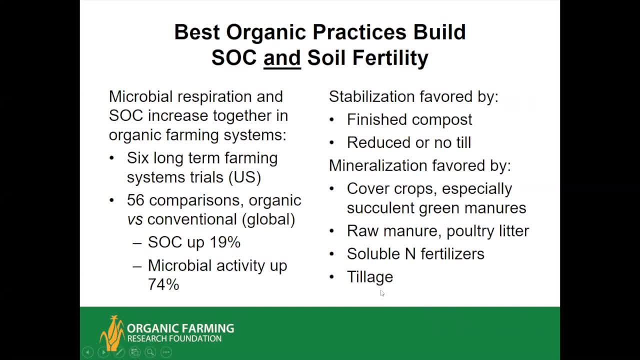 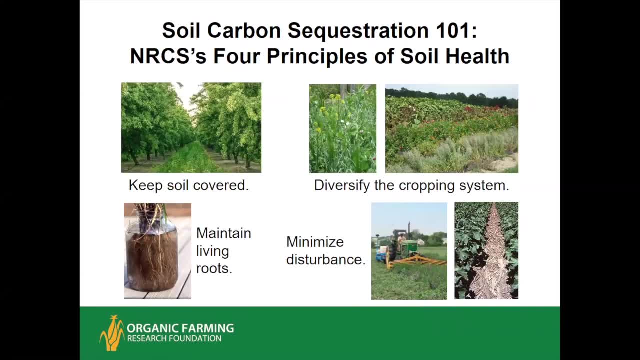 breakdown And, of course, tillage. we all know that that will tend to stimulate microbial breakdown of soil carbon. Okay, this is what I call soil carbon sequestration 101.. I also call it your tax dollars at work. in the best possible way. I do believe that by establishing these, 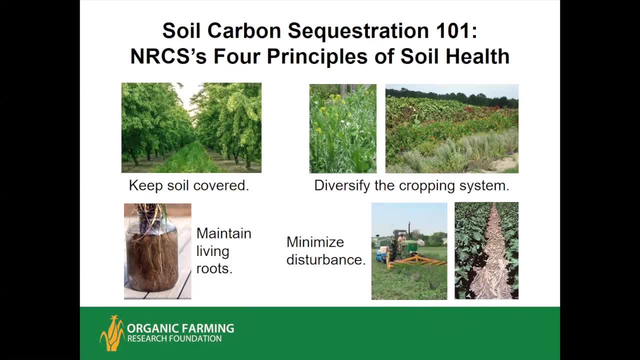 four principles of soil health. the Natural Resources Conservation Service has created at least some of the vital roadmap to agricultural carbon sequestration and climate mitigation: Keeping the soil covered, best of all in living vegetation, at the very least keeping it covered in residues. Here's an example of an orchard with a very 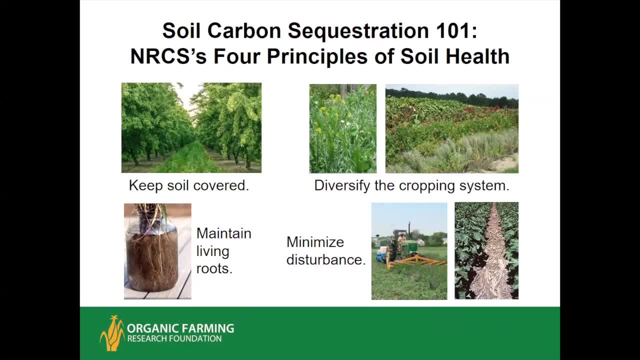 very rich cover in the alley and probably a lower cover. It's hard to tell right there actually that right under the trees that may be bare. The ideal is to have some kind of low growing cover or mulch. In any case, keeping the soil, the orchard floor, covered results in twice the organic matter, as you. 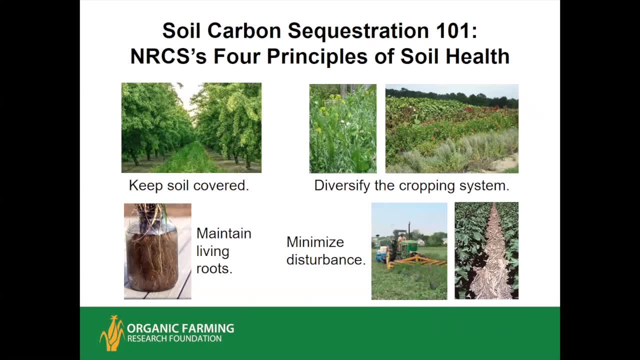 would have if that were a bare orchard floor maintained either by tillage or by herbicides, without tillage. Diversifying the cropping system. this is just a market garden, Showing a wide diversity of crops that look like everything from pole beans to herbs to cut flowers. 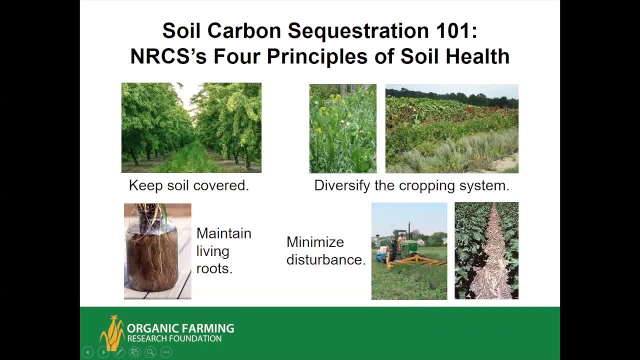 And here's a multi-species cover: crop Living roots are vital. We'll get into more of that that more later. but maintaining living roots as much of the year as possible makes a huge difference in how much carbon is entering the soil and how well it is staying there And minimizing 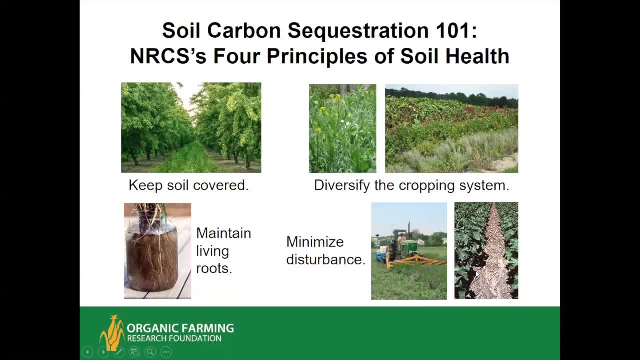 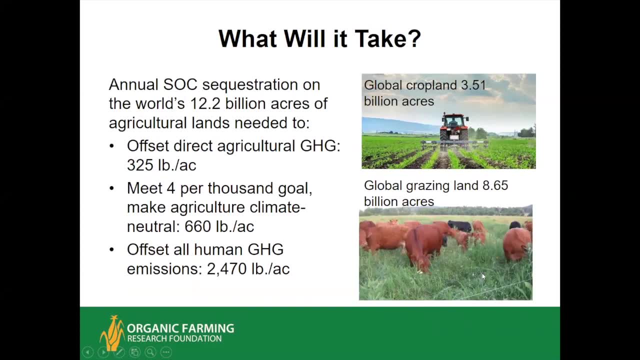 disturbance. Here's a roll crimper taking a cover crop down and here is a no-till planting of a vegetable crop. Disturbance can also include chemical disturbances, like high levels of soluble nitrogen from either chemical fertilizers or very concentrated organic fertilizers such as poultry litter. 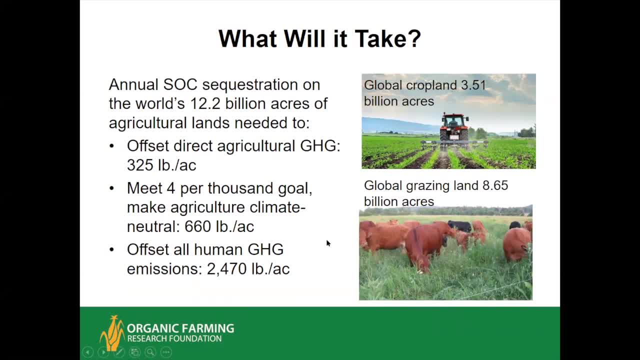 when used at high rates. So what will it take to really say meet the four per thousand of a global objective? The world has about three and a half billion, eight or twenty acres of crop land and another 8.65 billion acres of grazing lands. So let's take that. 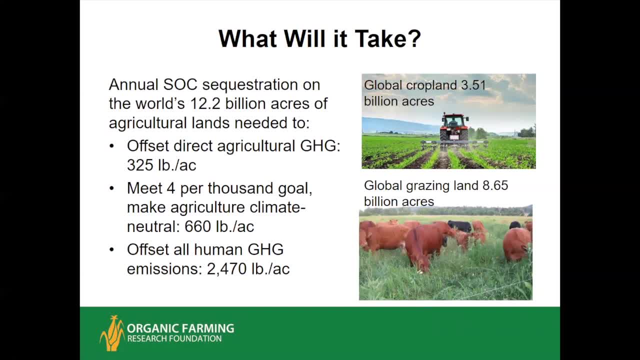 whole acreage and say: well, how much do we have to… how much carbon do we have to put in the soil every year to achieve different goals? To offset the direct agricultural greenhouse gas emissions, we need about 325 pounds per acre per year. To meet this four per thousand goal, we need about 660. 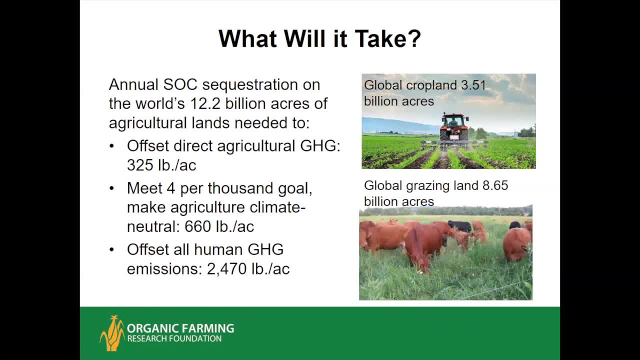 to offset all of human greenhouse gas emissions. we're looking at over a ton- 2470.. But keep those figures in mind as we look at the levels of carbon sequestration that have been documented for various conservation and organic practices. Okay, 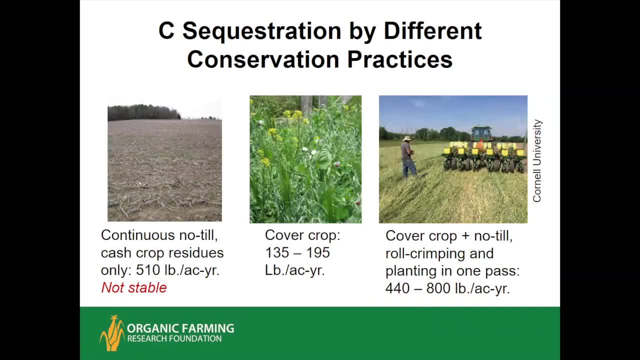 Okay, continuous no-till will sequester about 500 pounds per acre per year. You say, oh good, that's almost all the way to four per thousand just by itself. And then we add cover crops. If you're gonna till in the cover crop? 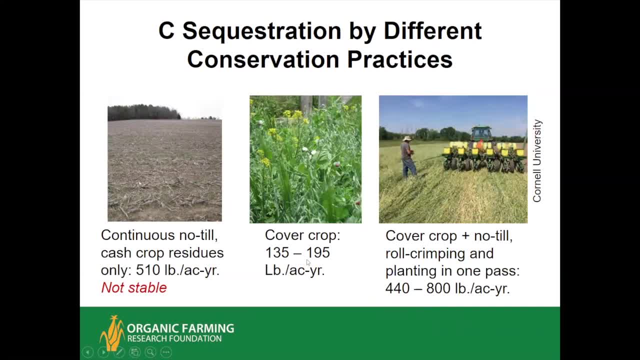 you're not gonna get a huge amount, maybe one to 200. But if you combine cover cropping with no-till by roll crimping the cover crop and planting in one pass, you can get up in the range where we're looking at the four per thousand. 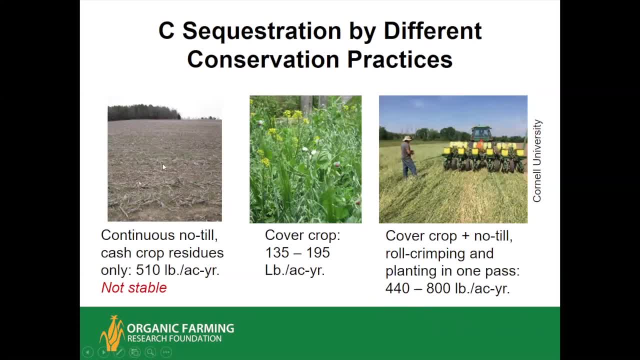 One caveat, though, is that, especially when you're not including cover crops and increased overall rotation intensity, keeping the ground covered just no-till by itself, just leaving the dead residue on the surface, That is not a very stable form of sequestration. 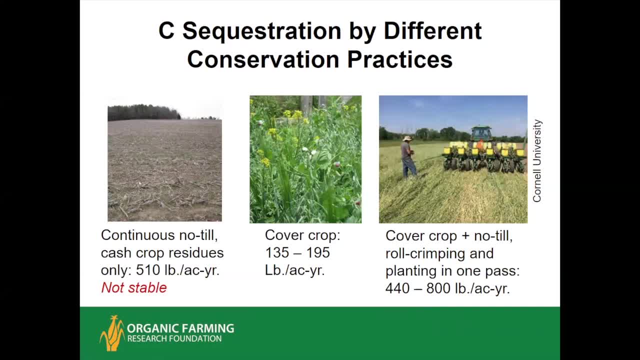 cause. most of the added carbon is physically protected in aggregates very close to the soil surface And you can see a little bit of weed growth there, even though this farmer habit using herbicides, So eventually you're gonna get a herbicide resistant weed. 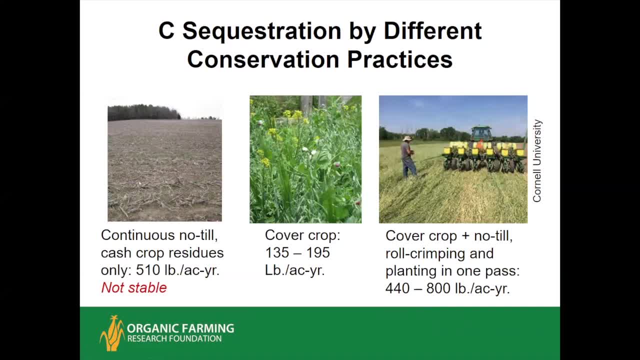 You're gonna get a perennial weed, get some compaction and you're going to have to get out there and do some tillage And even a relatively light tillage pass. let's say you decided you need to take. you know that that's. 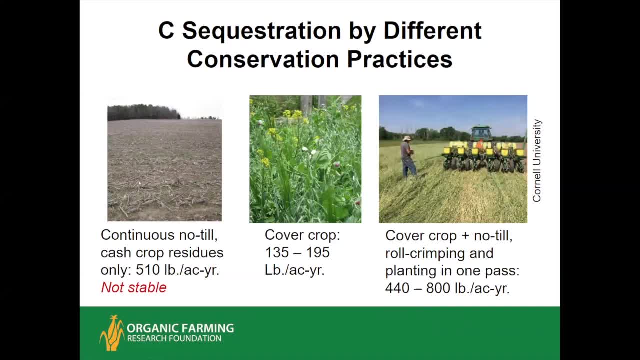 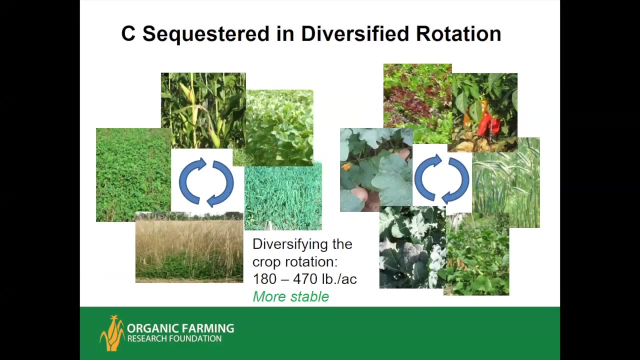 herbicide resistant, that weed grows you got to go out there with a harrow. Well, that can cause a lot of this crude carbon to break down very quickly. So it's so close to the surface not really anchored the way some of the stable organic carbon is Okay. diversifying the crop rotation. 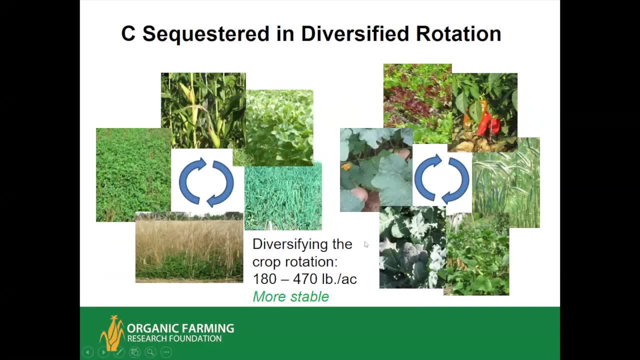 Anytime you increase the diversity of crops, you're increasing the diversity below ground, you're improving the function of the soil food web. And especially if you take what had been like a corn-soy rotation and you add a perennial phase- let's say you had a corn-soy cereal grain- 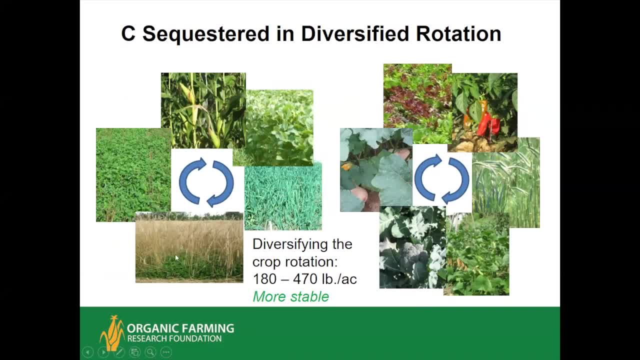 rotation. you had those three already and you just under seed it with a legume. you let that legume grow for a year. that is greatly increasing the root biomass and increasing the duration of living cover, And this will just diversifying even. 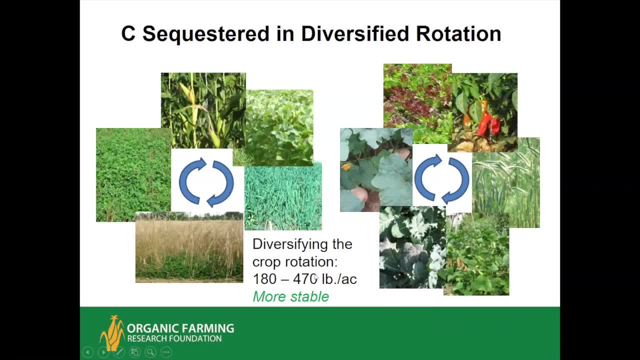 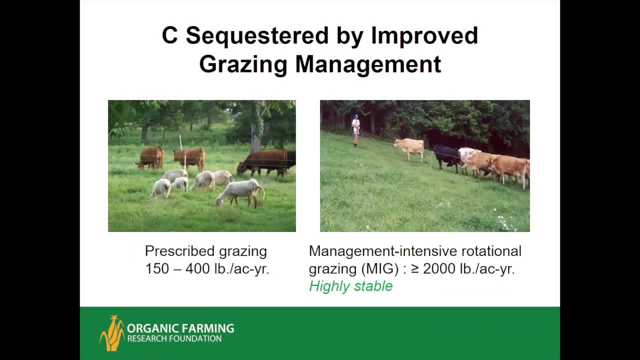 without intensifying particularly, will build up some more organic carbon And it's more stable than that. that's a crude no-till alone. Okay, grazing management, The NRCS practice called prescribed grazing, which is basically making common sense improvements to your grazing. 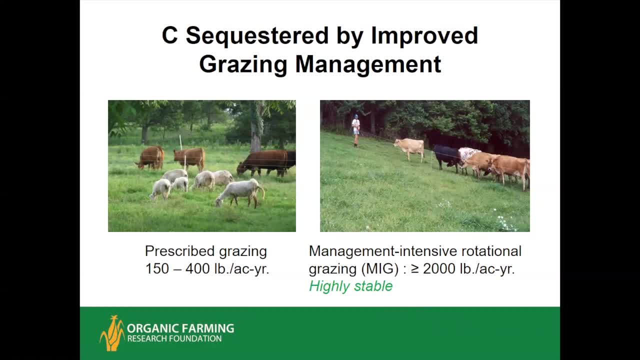 system like going from a continuous graze, which can be very destructive to the soil, to some kind of a rotational system where you graze an area for a while and then let it rest. take some other measures to maintain forage quality. The Chambers reference estimated that as accruing only 150 to 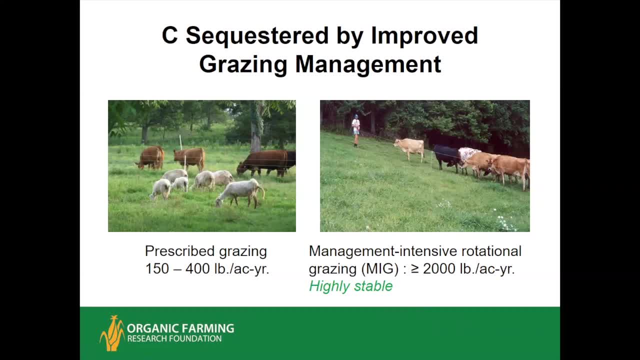 400 pounds per acre per year, perhaps getting close to making offsetting direct and emissions. However, management intensive rotational grazing systems. a number of studies around the country have shown that, when done properly- like you're moving the cattle every day or two and 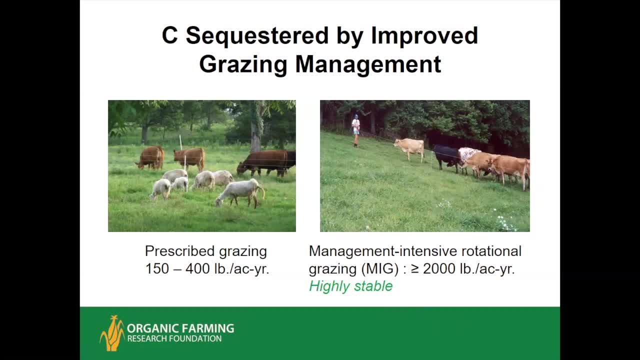 you're leaving them there until they intensively graze, but not to the point where the ability of the forage to recover has been injured. Then you move them off and you leave a long recovery period. This has been shown to build a ton or more of carbon per acre every year. 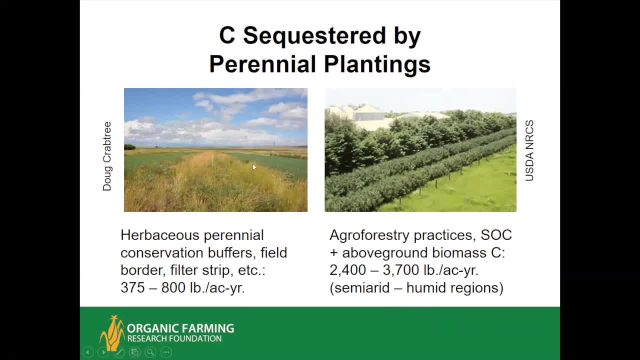 So now let's look at perennial plantings. Remember before I said how destructive it was to remove perennial cover. You lose soil, organic matter, you lose biomass, carbon. you get a tremendous net emissions. On the flip side is, if you take some sensitive land- some, perhaps some. 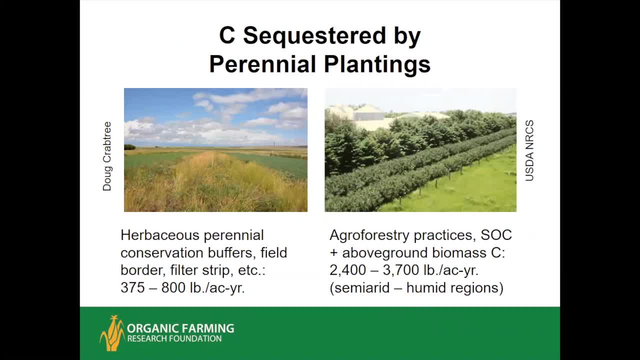 steep or marginal cropland, you say, oh, you're going to put this in perennials. You really are returning a lot of carbon to the soil. You're ceasing tillage and you're providing year-round living roots and year-round plant cover, Going to pervasive. 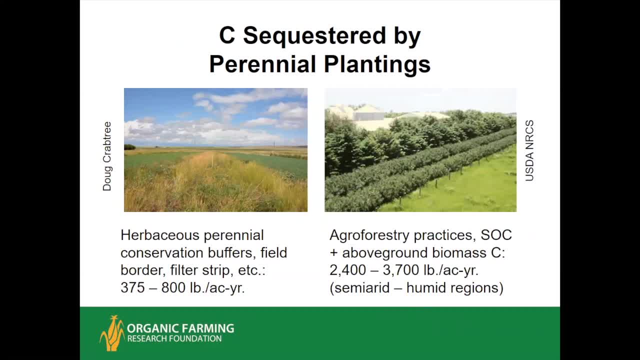 perennial conservation buffers, things like field border filter strip. This is an example of Doug Crabb theory of Villicus Farms in Montana has an excellent system there for organic dryland grain production And here is a conservation buffer strip that is going through the field. 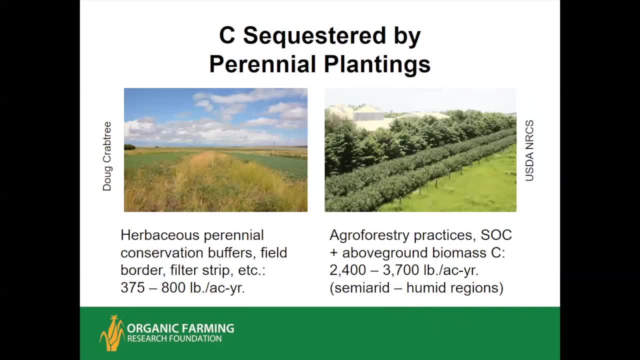 He has these regularly through the fields to provide habitat for beneficial insects And it also is increasing the carbon sequestration in that strip. Another example is over here. This is a hedgerow, a multi-purpose, multi-species hedgerow, this entire area under permanent. 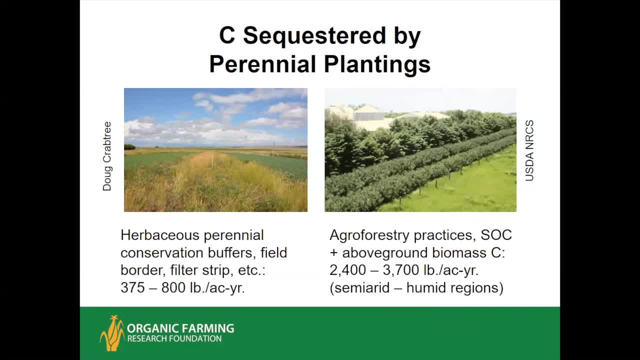 perennial woody vegetation. There was a study by Feliciano and Associates of Agroforestry Practices that these perennial plantings will typically sequester one to two tons per acre every year, some as soil organic carbon, some as above ground biomass. 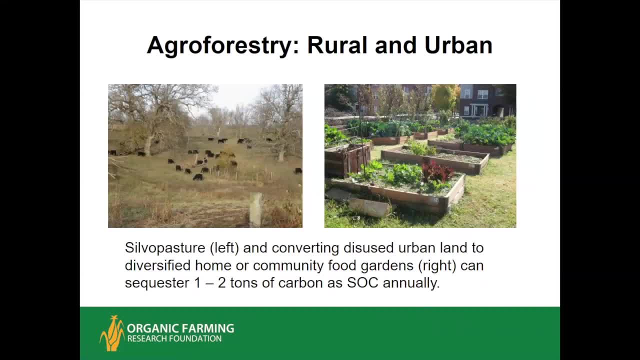 Two practices in that review that emerged as especially effective are: silvopasture, where you have grazing animals on pasture which has an open stand of woody trees or other woody perennials- Somehow that comes. The combination of the rotational grazing and of the pasture and of the woody perennials. sequesters. 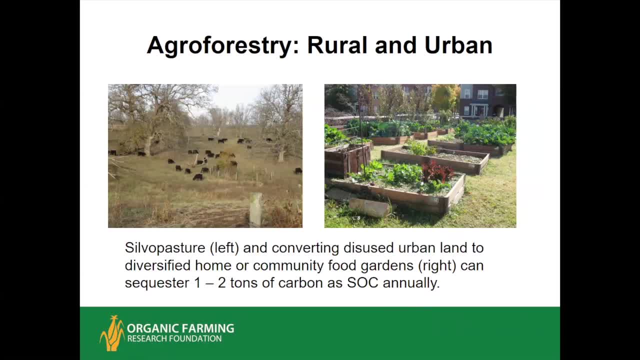 one to two tons of carbon in the soil every year, plus whatever the trees are accruing. Also, if you take an abandoned lot in an urban area, this is disused land, it's not growing anything, it's dead, and you start a community garden that's going to be similarly, building up a large amount of carbon. 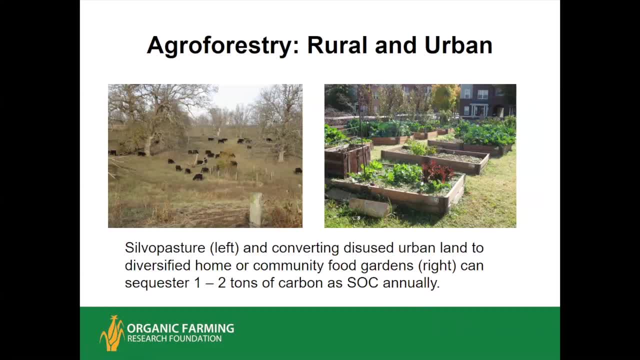 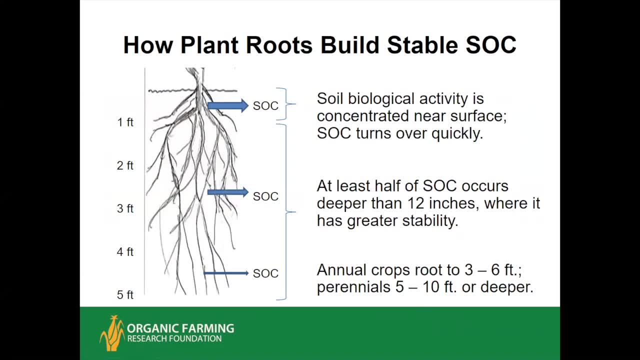 So something to be said- It's not just for urban agriculture, in addition to all of its socio-economic benefits. So how do plant roots build stable soil organic carbon? Most of the biological activity and the highest concentrations of soil organic carbon, and therefore the darkest, richest looking soil, occur within the top 6 to 12 inches. 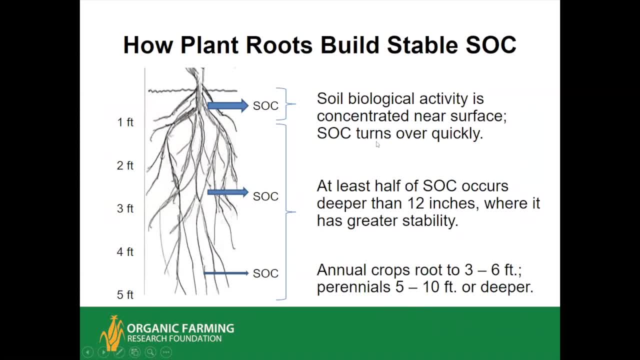 However, this does turn over quickly. This is where the mineralization and the nutrient release is concentrated. But at least half of all soil organic carbon occurs below 12 inches, And down here it has greater stability because you're not plowing that deep, you don't have as much oxygen. biological activity is slower. 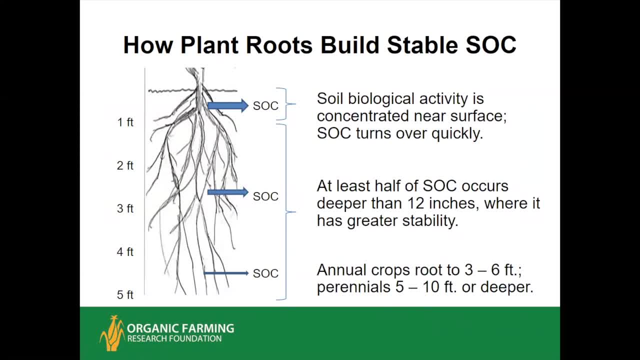 so the carbon tends to remain where it is. Annual crops typically root to three feet, sometimes to six, and perennials tend to go five to 10 or more feet deep into the profile. So there is always the potential for plants to deposit carbon down here. 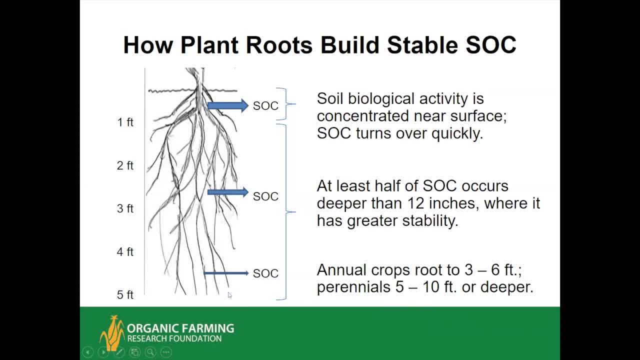 So there is always the potential for plants to deposit carbon down here here, and it has a much longer residence time, much longer turnover time, and therefore it makes a significant contribution to sequestration, And this is a contribution that will not necessarily. 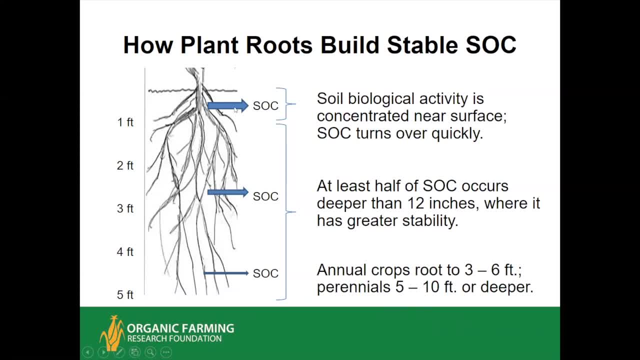 be measured in studies that focus on this top foot And, granted, it's pretty hard, it's pretty labor-intensive and cost-intensive to do studies that go all the way down. So a lot of our sequestration studies have been done in that topsoil. Okay, big caveat: We cannot expect. 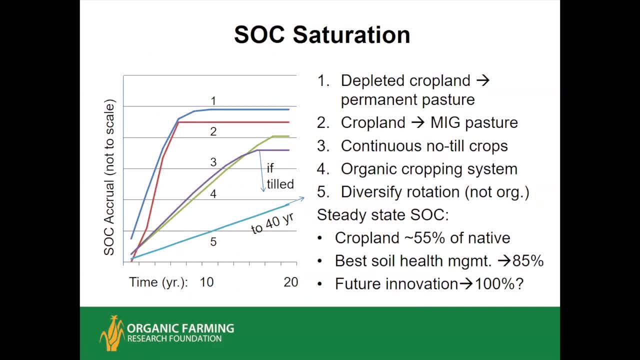 agriculture to go on sequestering carbon. Not the best organic, sustainable or conservation agriculture system is going to continue to remove carbon indefinitely. So we can't say, oh well, we can still drive our SUVs because agriculture is going to soak it all up. 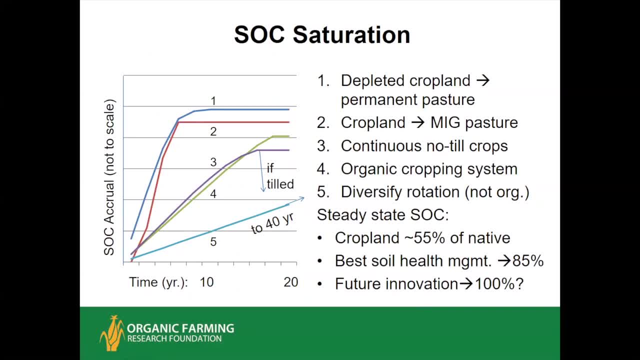 What agriculture will do is help us during the transition period toward a carbon-neutral society and economy and technological system. It'll give us a little bit of extra time to make the important transition to zero emissions by mid-century. But here are a few examples of what happens after you improve practices Now. 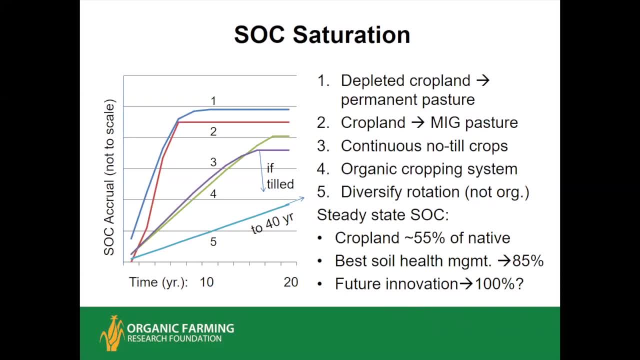 these are not all to scale. Just be aware of that. The two on top are the largest accruals, but by drawing them to scale these curse. So the first example is a study in Portugal where they converted some depleted cropland. 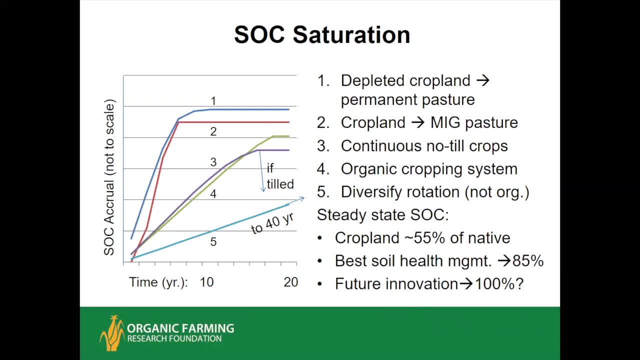 to permanent pasture For about six years. there's a very rapid increase in soil organic carbon. The soil organic matter went from 0.87 up to 3%, So that's a gain of perhaps that would be over 2% of organic matter, over 1% organic carbon, So more than 10 tons. 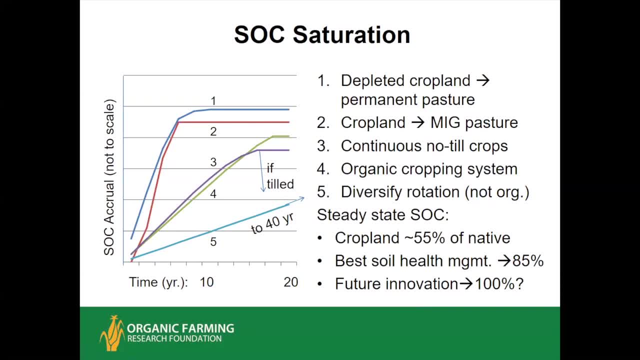 But then again it leveled off once that pasture reached a new steady state of healthier soil. but then the soil- organic carbon- levels off. Similarly in South Carolina, converting filled cropland to a management-intensively grazed pasture. there was a couple years lag. 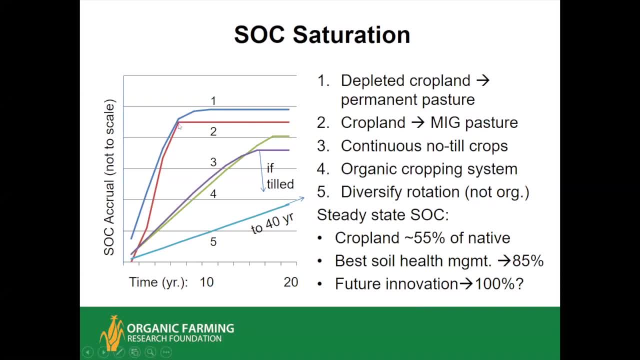 and then there was a tremendous rapid burst for about four to six years of accruing carbon, as much as 25,000 or 30,000 pounds per acre over that four-year period. Then it leveled off Again in the Rodale Farming Systems Trial, that's curve four. there was a steady increase in organic 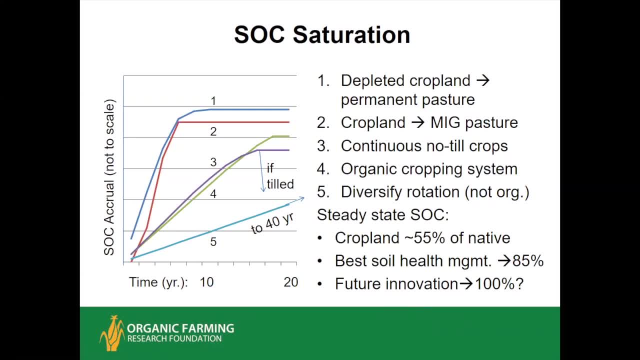 carbon for about 20 years And then it leveled off. the soil organic matter number went from 3.5 up to 4.2, and then it leveled off. That was about 7,000 pounds, about three and a half tons. 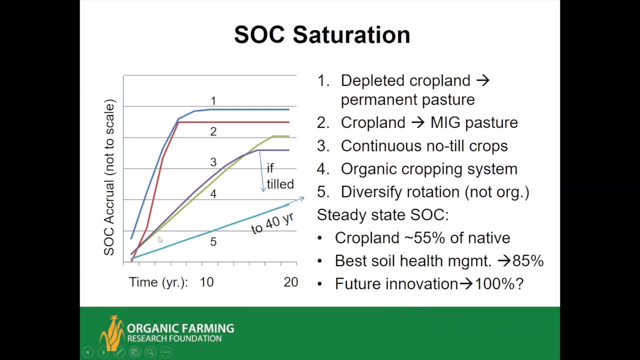 of carbon. Similarly, the paper that discussed, on which I based that: 500 pounds per acre per year for continuous no-till, that's by West and Post 2002, they estimated that it would continue at that rate for about 10 years, then gradually level off, with a big caveat that if you have to till even once to 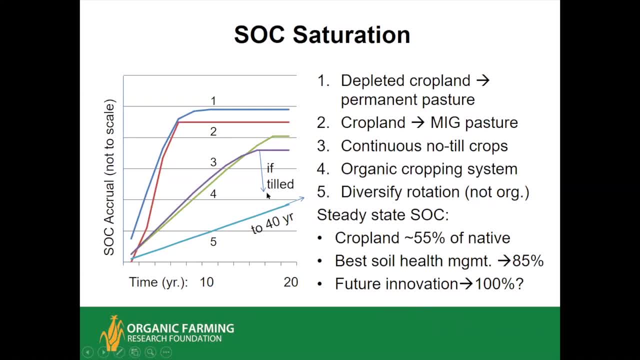 deal with a compaction or a weed problem, you'll get a sharp drop, very rapid drop in that soil carbon. In the same review, the same authors found that simply diversifying a low diversity rotation. say you had corn-soy, you went to corn-soy wheat or corn-soy with winter cover crops. 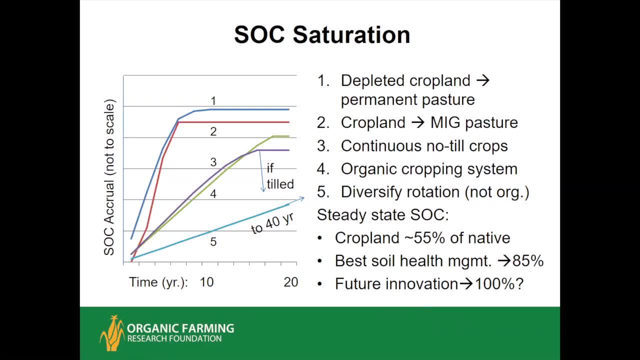 simply adding that extra crop, you get a slow, steady increase in soil organic carbon. that takes 40 years, but it continues and it eventually reaches that same ballpark of three to four tons of net gain per acre. They say, okay, how big an impact can this be? Well, let's remember that. 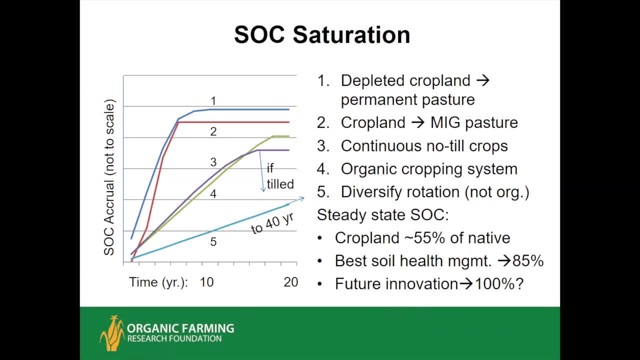 in native agricultural, native plant ecosystems there is a steady state level of soil organic carbon and let's call that 100%. That's what it was before agriculture. That's when the soil organic carbon pool was at its maximum. Cropland on average is about 55% of that native level. 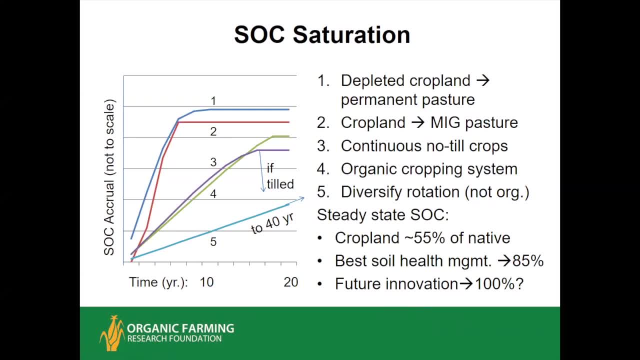 but it's been estimated that best soil health management practices, such as we discussed here and such as there's done under good organic management, will easily get that up to 80 to 85% and that future innovations could bring us up to 100%. 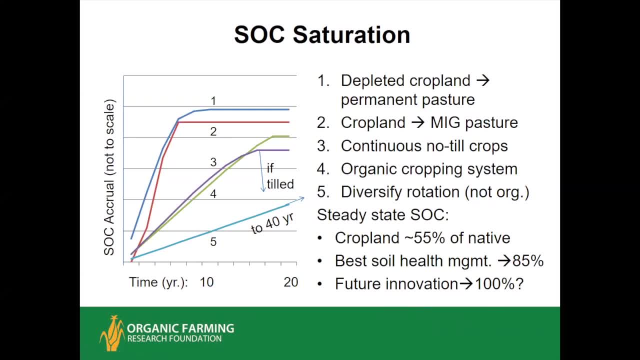 And what does that mean in terms of helping us get over the hump towards stabilizing the climate? That will absorb this. 85% would absorb somewhere. if applied to the whole world's agricultural lands, would absorb somewhere between three and eight years' worth. 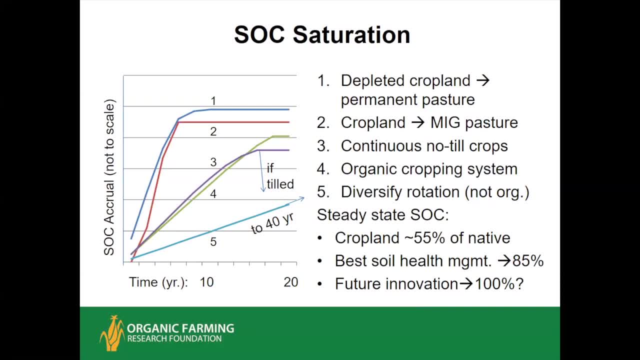 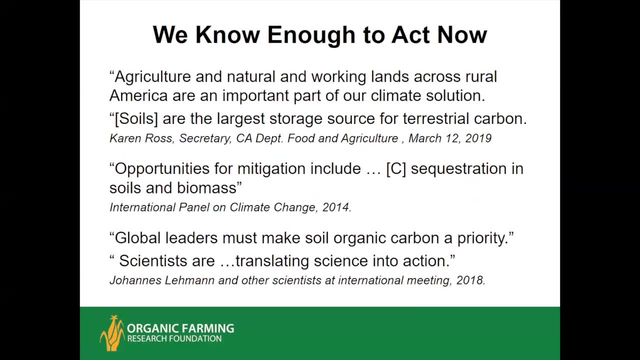 of human greenhouse gas emissions Doesn't solve the problem, but it is quite significant. So basically, in short, more and more leaders are saying we know enough to act now. The California Department of Food and Agriculture Secretary, Karen Ross, says here: agriculture. 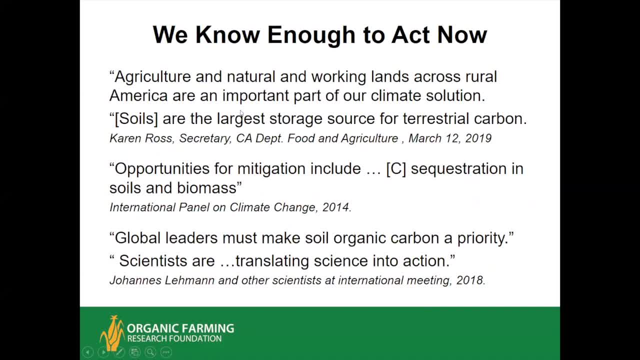 natural and working lands are an important part of our solution because soil is the largest storage source of terrestrial carbon, as shown in that carbon cycle slide I showed earlier. International Prop Panel on Climate Change and our 2014 report realized this is an important factor in helping the 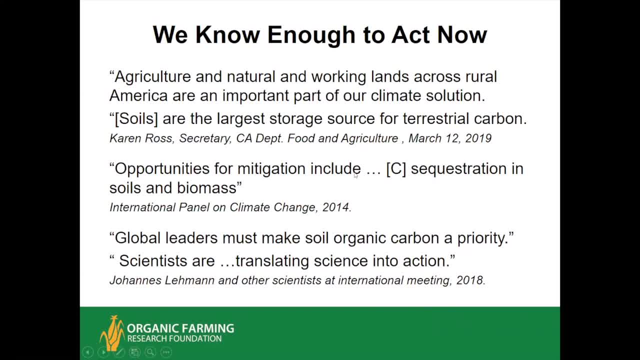 report emphasized sequestration in soils and biomass as a mitigation strategy And more recently, last fall, there was a meeting of scientists in London, and Johannes Lehman is at Cornell University. He basically said global leaders must make soil organic carbon a priority, And it was noted also that scientists are already 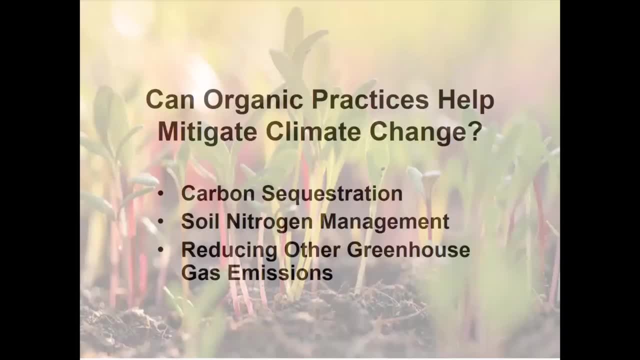 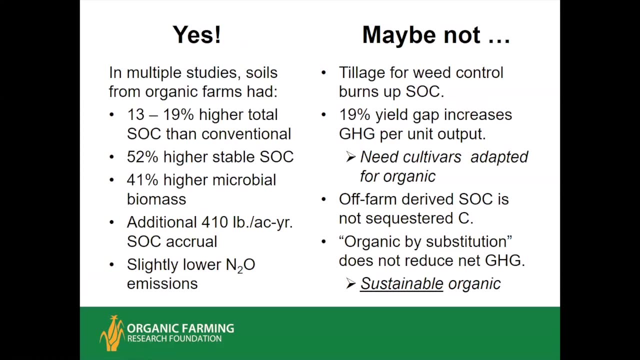 translating science into action. Okay, So how can organic help? There's been a debate, actually. Some say: yes, organic will definitely sequester more carbon. In fact, some of those meta-analyses show that organic soils have 13 to 19 percent more. 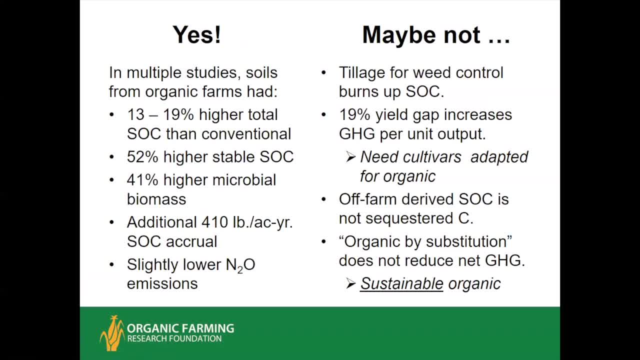 soil organic carbon on average. It's not a huge jump but it's significant. And the stable organic carbon is. In the US study of about 700 organic fields and 700 conventional fields it was 50% higher, So that's quite interesting. Again, the higher microbial biomass. 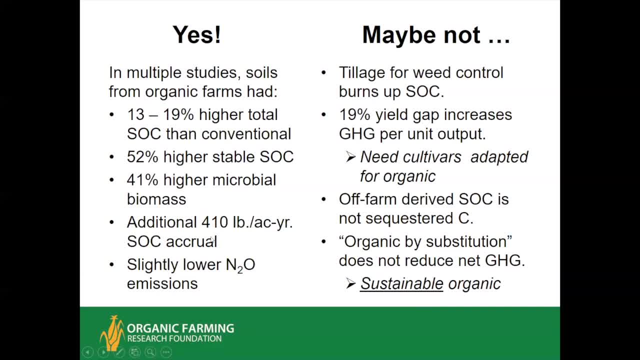 And organic systems have been shown to accrue about 410 pounds of carbon per acre per year And a generally slightly lower nitrous oxide concentration. We'll get to more of that later. There are some who question whether organic can be part of the solution. The most challenging issue is tillage for weed control. 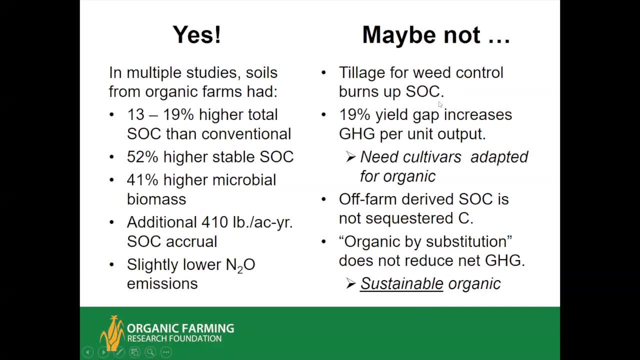 Yes, that can burn off soil organic carbon. I will refer you all to one of the guides on soil health at the Organic Farming Research Foundation addresses practical means to reduce tillage in organic systems. It's not a black and white issue. You can till with care and 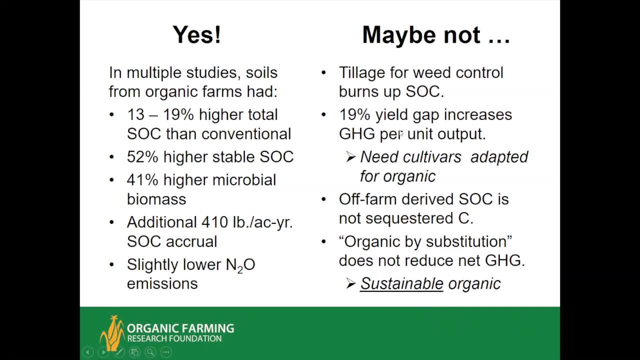 minimize this impact. Another criticism is that, on average, organic farms yield 19% less than conventional. Well, we need cultivars that are adapted to organic systems. In this meta-analysis that showed that organic systems sequester another 410 pounds over conventional. about 60% of that was. 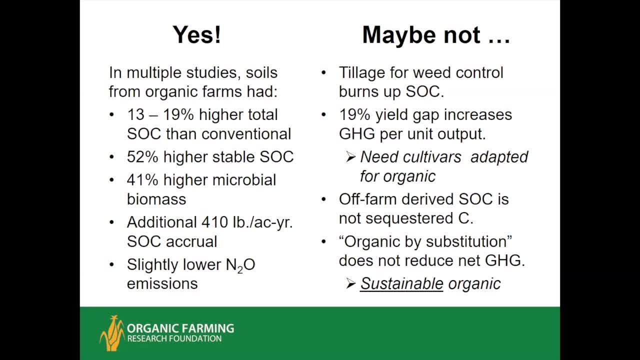 indeed sequestered, and the other 40% was imported. And there was one other study that thought that well, adoption of organic agriculture is not leading to a reduction in the agricultural greenhouse gas footprint. And the point here really is just that organic by substitution, just by 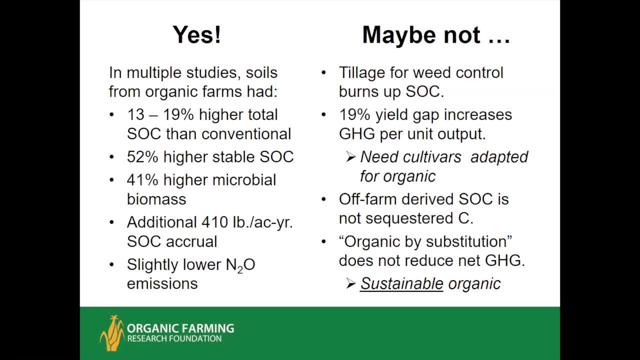 following the NOP rules for what you can and can't use is not going to change your carbon footprint. It has to be sustainable, organic, And it's basically combining organic practices with all what we talked about before, which really are organic practices when you look at the standards. 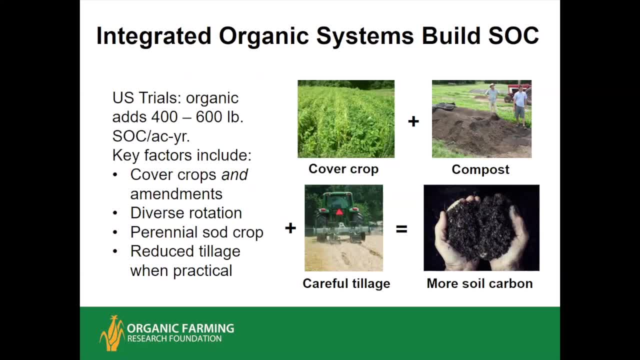 Okay, can you advance that one? Okay, great, All right. so this is at the point. Several trials across the United States indicate that organic systems that do use some tillage will accrue 400 to 600 pounds per acre per year compared to the conventional system, And in some cases that advantage. 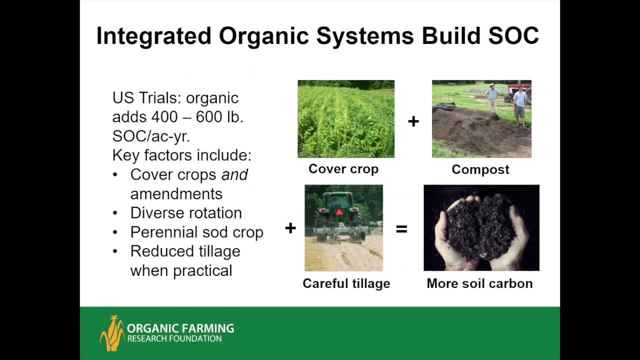 actually applies to organic versus a conventional no-till system. The key factors what makes a good farming system build organic carbon are the cover crops and amendments. They work together in complementary ways to build stable organic matter. Diversifying the rotation, as I mentioned, having a perennial 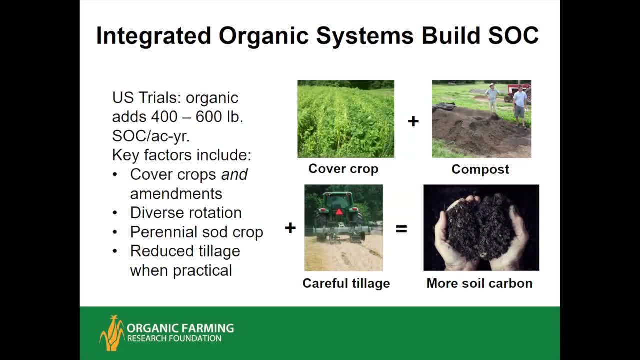 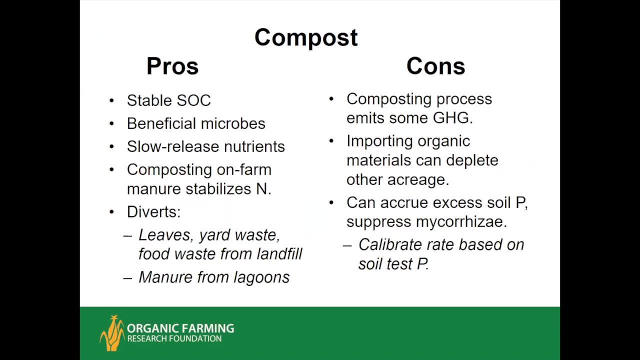 sod crop gives you that duration and depth of root growth and reducing tillage to the extent practical. Okay, go ahead and advance it. It seems like it's denied me access. Okay, so compost. This is pros and cons. It's a very valuable material for building stable. 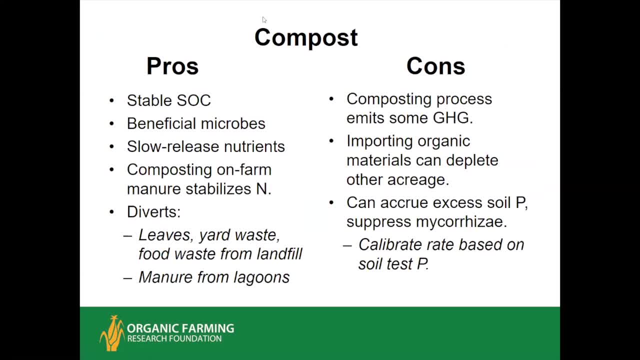 organic matter, providing beneficial microbes, slow-release nutrients and also if you use composting process for on-farm manure and other wastes, it really stabilizes our nutrients. And another thing is if you're importing materials but you're diverting them from. 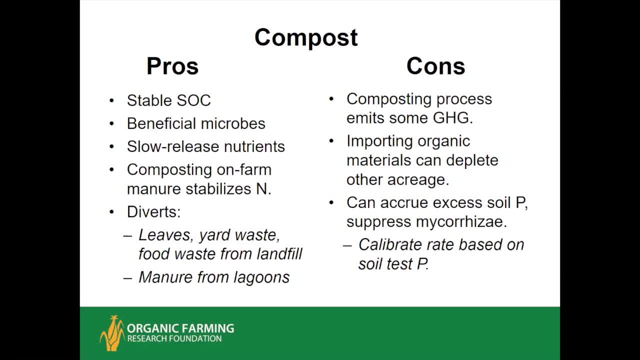 the landfill or taking manure that would otherwise go into a lagoon, you're reducing the greenhouse gas emissions from these organic materials. Okay, The cons are that composting process does emit some greenhouse gases, but far less than landfilling or lagoons. If you're importing organic matters from other acreages, you're. 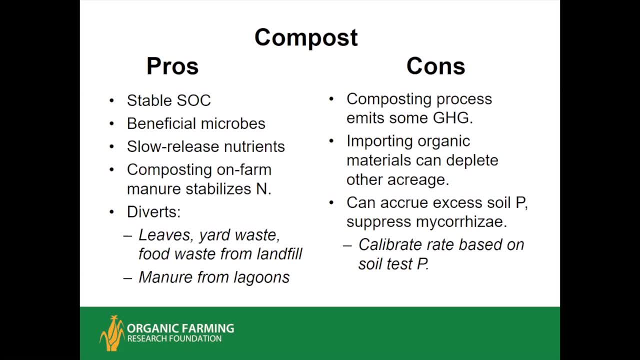 cutting hay from one field to make compost for another farm, you are withdrawing carbon from other fields. That's not so sustainable. The other big caution is that, using compost as your major source of nitrogen and organic matter, you can rapidly build up excess of. 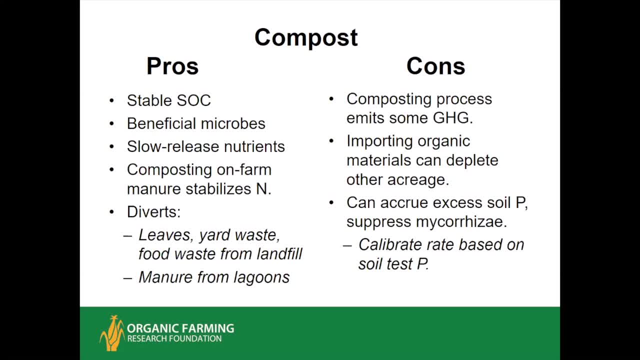 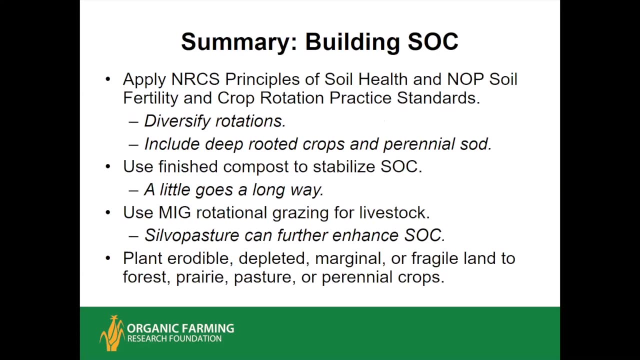 soil phosphorus. That phosphorus suppresses mycorrhizal fungi, so it's important to calibrate your compost use to maintain moderate phosphorus levels. Okay, go ahead, Dan. Thank you Okay. so just a summary: the NRCS principles and the NOP standards: diversifying rotations. 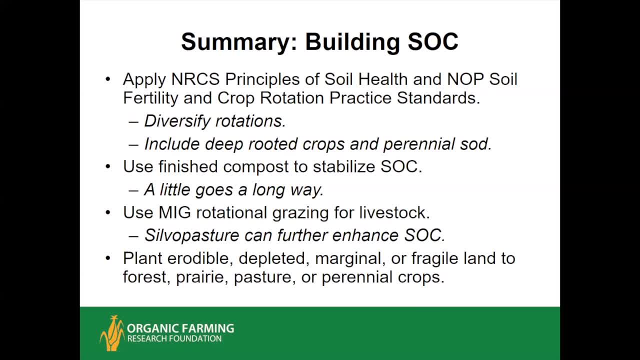 including deep-rooted crops and perennial sod, using a little finished compost to stabilize that carbon. the management and test of rotational grazing, And then any erodible, depleted or fragile land, getting that back into perennial crops or forest or prairie- those are the leading ways that farming can build carbon. 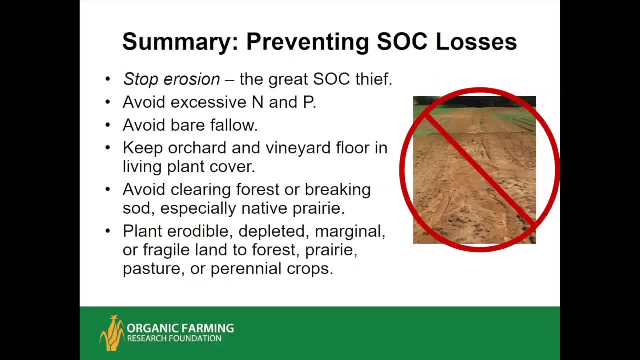 Okay on So preventing some losses. Erosion is the great soil: organic carbon thief. As we saw, that's responsible for one quarter of total agricultural greenhouse gas footprint. Avoiding excessive nitrogen and phosphorus to enhance the carbon footprint of the crop And then 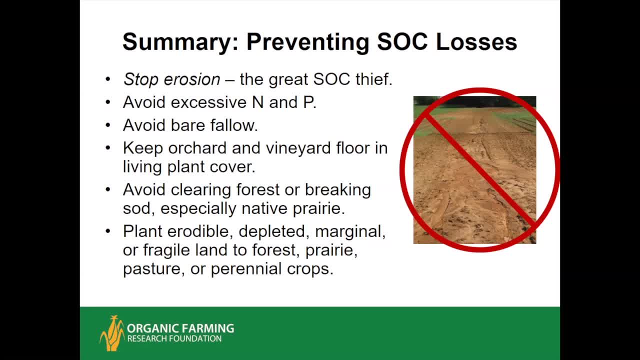 as I said, maintaining a substance of some of the potable vegetables, including their particulate matter, and maintaining the Tulsa, which is the third most valuable natural plant that we have in terms of tone supplies, fertilizer and otherfar-referencing� can. 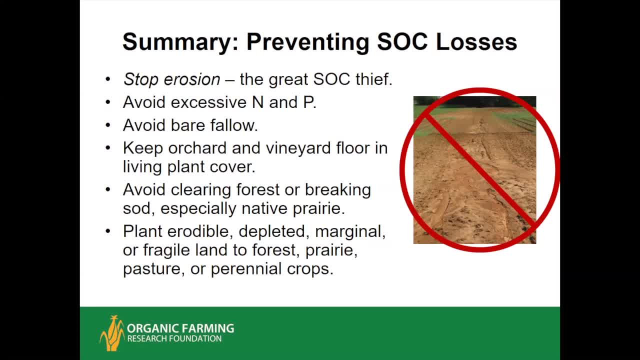 ensure a decent chance that plant-roots microbial partnership. Avoid bare fallow. Bare fallow is worse than tillage in my opinion, based on a lot of view of a lot of research. Keeping the orchard and vineyard floor in living color cover. Avoid clearing forest or breaking. 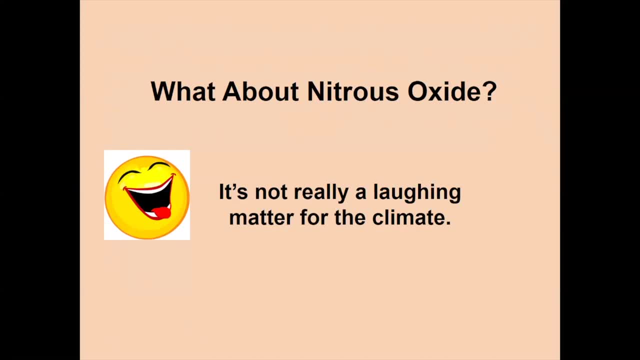 sod, especially any native plant communities, if you can. And then again, restoring those, Yeah, nitrous oxide. We're getting a little short on time. We're going to have to go through this one a little bit quicker, Okay, next. 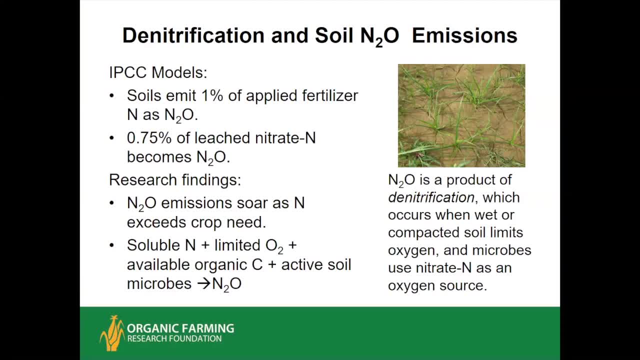 So where is the nitrous oxide? comes from the soil when denitrification occurs, or it's nitrate nitrogen in the soil, or ammonium nitrogen and its way being transformed into nitrate. All of these changes are mediated by soil life, And the denitrification and the formation of the nitrous oxide tends to occur when the soil is very wet but not completely anaerobic. You have limited oxygen but not completely devoid. 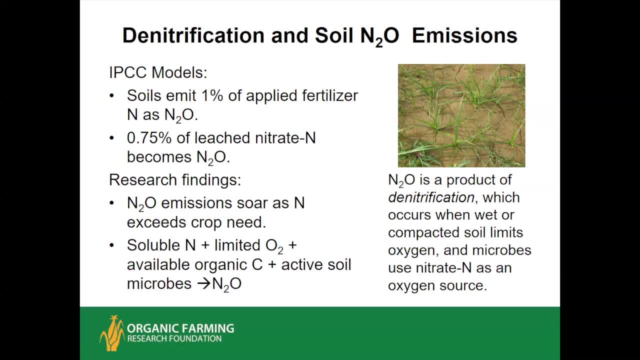 Now the International Planet of Climate Change has estimated that soils emit about 1% of applied fertilizer nitrogen as N2O and then, above whatever nitrogen leaches, three quarters of 1% eventually becomes nitrogen oxide again. And So, just as an example, if you've got a corn crop and you put 200 pounds per acre of nitrogen, which is often done, 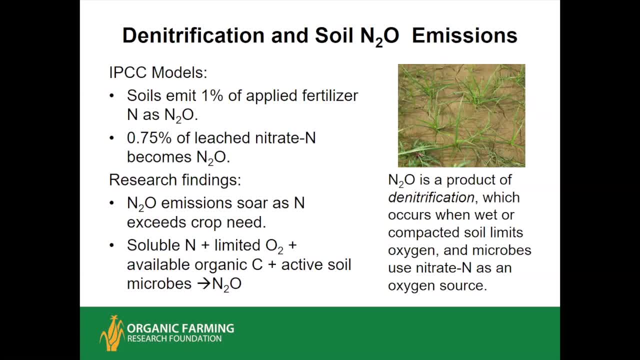 And then let's say, half of that leaches because you've got a pretty high rainfall climate. So of the 200 pounds, two pounds goes off as N2O, and of the leached 100, another three quarters of a pound. That two and three quarters pounds will offset 366 pounds per acre of carbon sequestration. 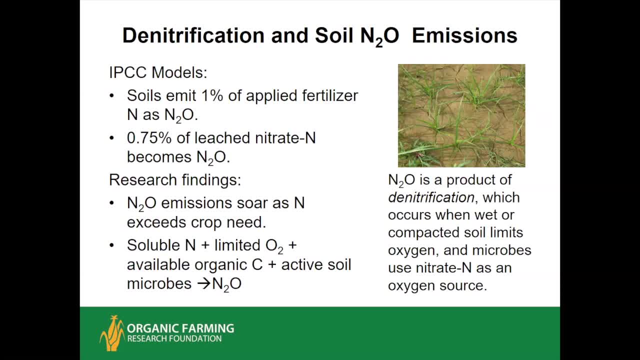 So if your corn residue returned enough carbon to raise your soil by that much, then it's been zeroed out. So some research findings related to this, that the nitrogen emissions- nitrous oxide emissions- soar when the nitrogen applied exceeds crop need. And it's the combination of soluble nitrogen, limited oxygen and N2O. 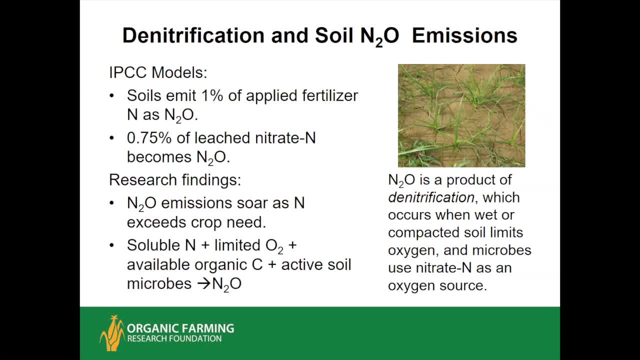 Plenty of available organic carbon. So in this case, when you have high organic matter, high active organic matter and lots of active soil microbes, you get more nitrous oxide. An interesting, a couple of interesting data here to consider. When the soil is below field capacity, which means field capacity is the soil moisture level, when all of the 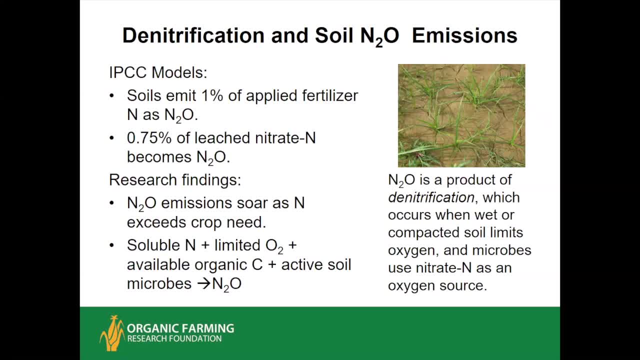 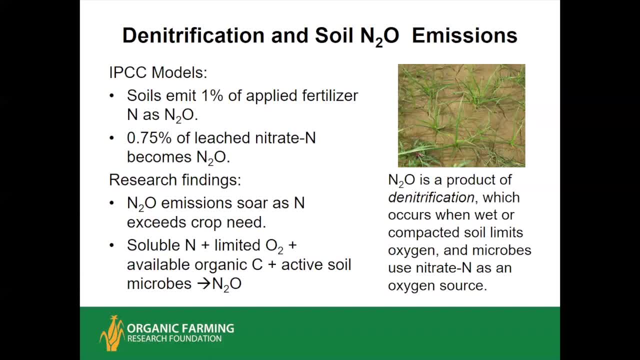 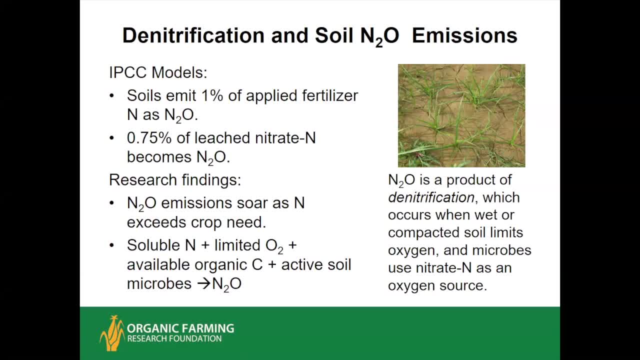 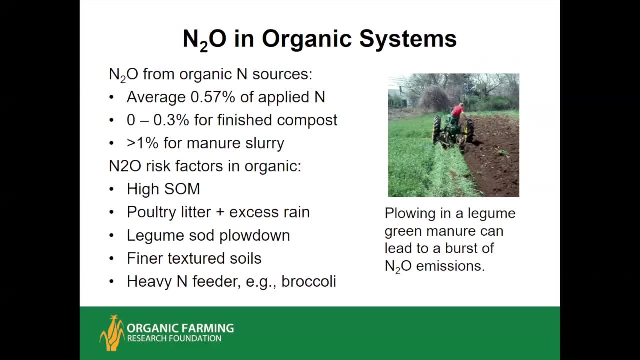 You will basically get no nitrous oxide. Next Okay, inorganic systems. A meta analysis- organic fertilizer- suggested that that emissions factor is not 1% but only a little over half a percent. But it's very variable. You got very stable sources like a good finish compost based products. 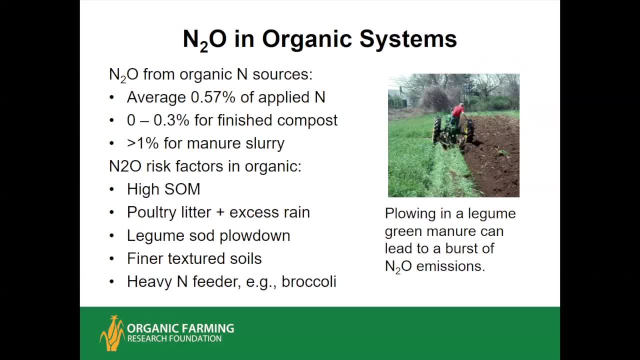 But you got very variable. You got very stable sources like a good finish, compost based products, compost- it can be close to zero. If you're applying manure slurry, it can be above one percent because you've got the soluble nitrogen and also soluble carbon at the same time. 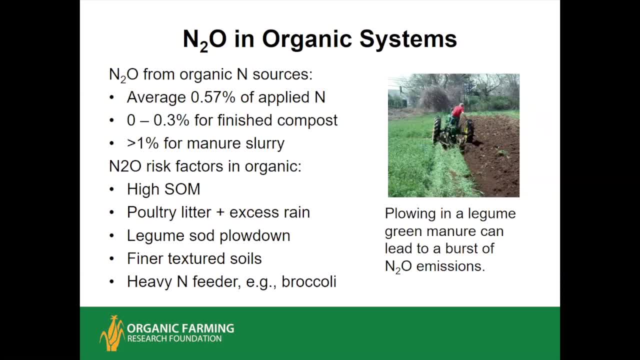 So some risk factors in organic high soil organic matter. it's been estimated that every increase in one percent soil organic matter may increase emissions by about 25 percent. Combination of poultry litter as your main nutrient source, organic fertilizer and high rainfall, that can create very large bursts of nitrous oxide emissions Whenever you plow down. 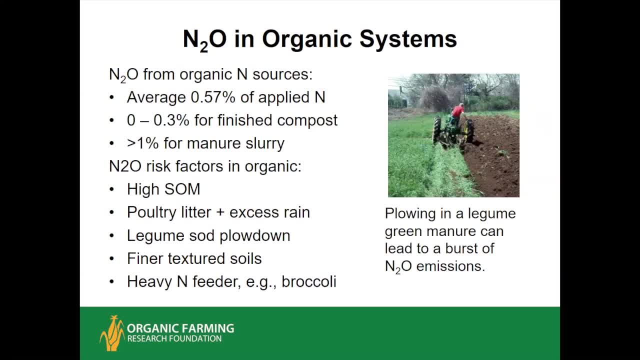 a sod, a legume or even an annual legume cover crop like here, you're putting all that succulent, high nitrogen material into moist soil and you're likely to get a nitrous oxide burst. Generally heavier soil, silt loam, clay loam will have higher emissions than sandy loam because 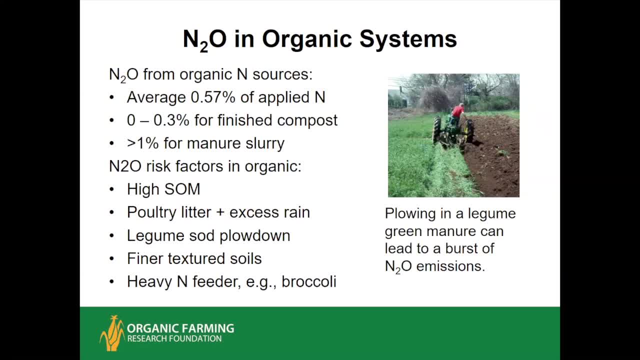 it's a little harder for oxygen to diffuse in. And here's a really extreme example: Broccoli is such a heavy feeder that it gives an economically viable response to added organic nitrogen, as in feather meal, up to 220 pounds of nitrogen per acre. 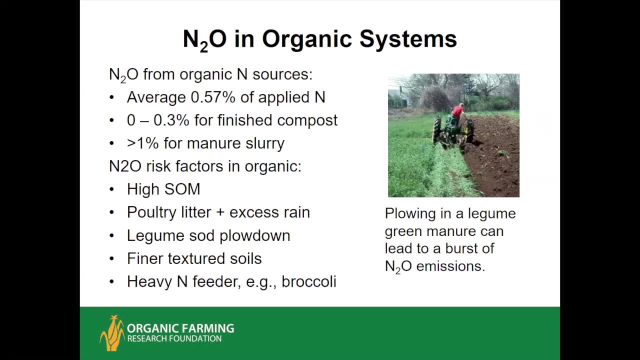 Now that gives the best economic return because of the yield response. but it also has been estimated to release as much as 11 to 27 pounds of that nitrogen as nitrous oxide. This is in a study in California, either under irrigation or during the wet season. but 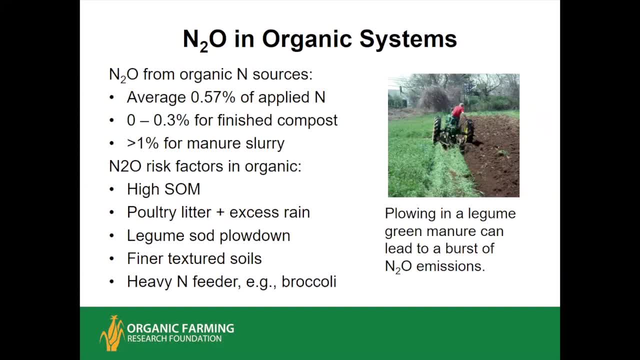 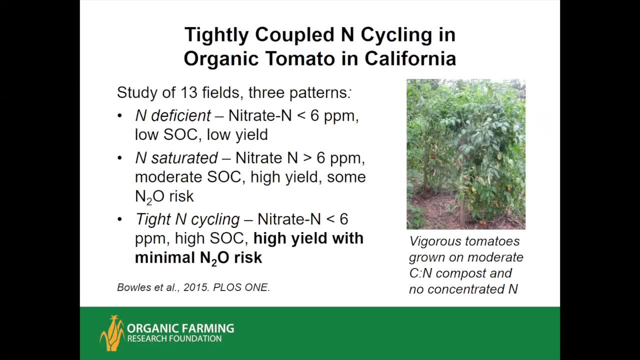 in any case, it's a very good example. It was kind of a perfect storm and that offset more than a ton of carbon sequestration. Next, On the POS side, another study in California looked at 13 different fields. where they were. 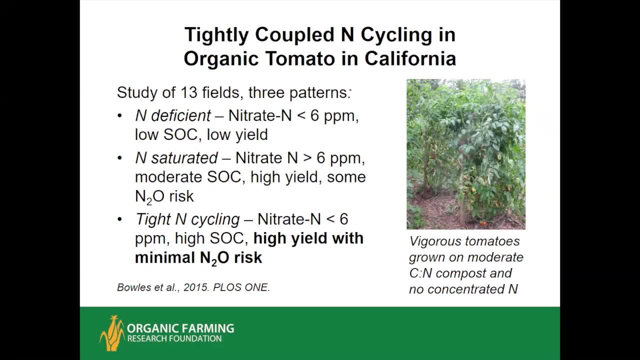 growing organic processing tomatoes and they found three different, distinct patterns. One is nitrogen deficient. The soil nitrate was below six parts per million. but the organic matter was also kind of low and the crop was even lower. So it was kind of a perfect storm. 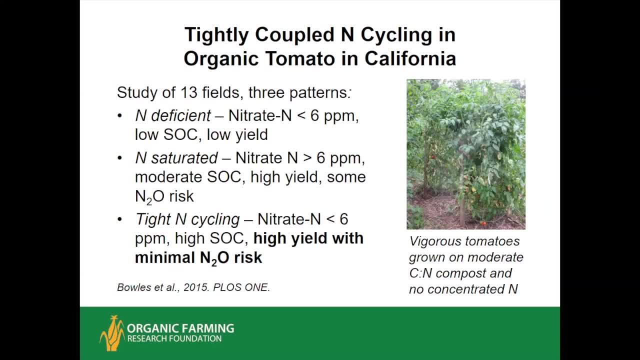 Nitrogen: was nitrogen limited in its yield? Nitrogen saturated: There were some high concentrated organic fertilizers such as guano or poultry litter. Nitrate levels were above six parts per million, quite a bit higher sometimes, and there was some risk of nitrous oxide. 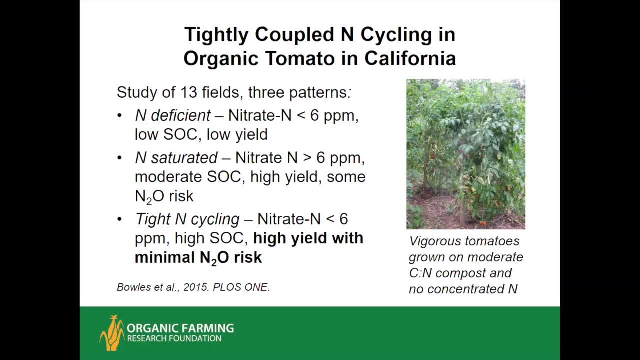 And then tight nitrogen cycling. There were four fields where they used a lot of compost, finished compost which has a very low level of soluble nitrogen, and then a very small amount in the row Of either Chilean sodium nitrate or poultry litter or other concentrated nitrogen, and that 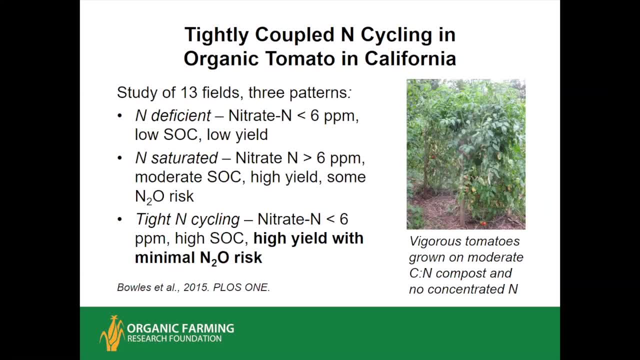 maintained a bulk soil nitrogen level less than six percent. These were fields that were what we call mature organic fields: high levels of soil organic carbon, high levels of beneficial microbial activity, and we had the combination of high yield and minimal risk of nitrous oxide losses. 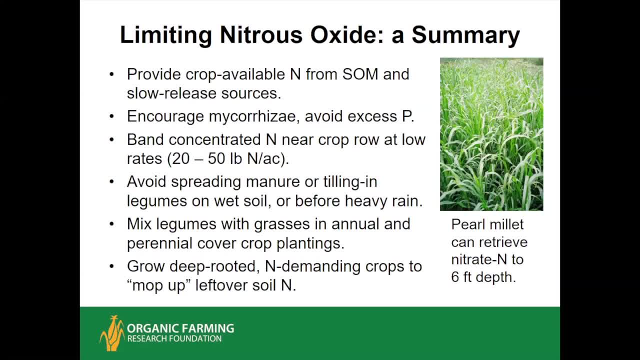 Next. Okay, just a summary of practices Organic and other farmers can use to limit nitrous oxide losses. A lot of research needs to be done in this area. This is not a definitive, but these are some guidelines based on what we know now. 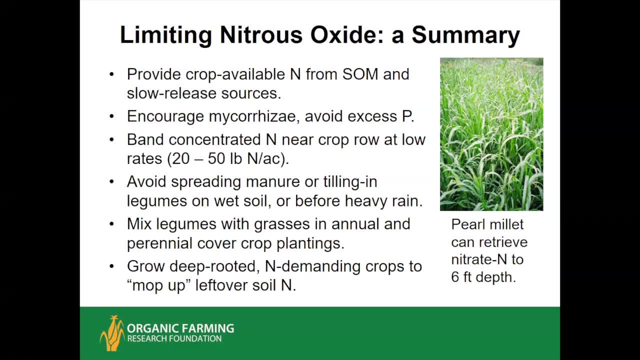 Definitely encourage mycorrhizae. avoid excess phosphorus. Mycorrhizae themselves have been shown to reduce nitrous oxide evolution from the soil. Rely on your soil organic matter and really slow release sources as much as possible for nitrogen. 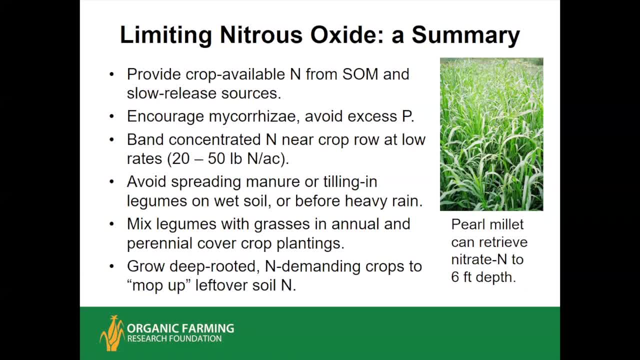 Your crop. if you need a little bit of concentrated nitrogen, band it near the crop row. There was one study with a liquid fertilizer application on organic lettuce in Colorado and, when done properly and at these low rates, there was almost no nitrous oxide. 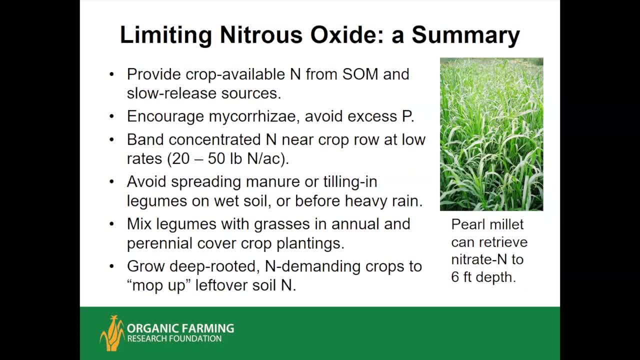 And avoid spreading manure or tilling in legume when you're likely to have wet soil. If you're going to have a cover crop- either a perennial sod or annual cover crop- mix grasses with your legumes And then really deep-rooted nitrogen-demanding crop like this pearl millet can send its roots down six feet. 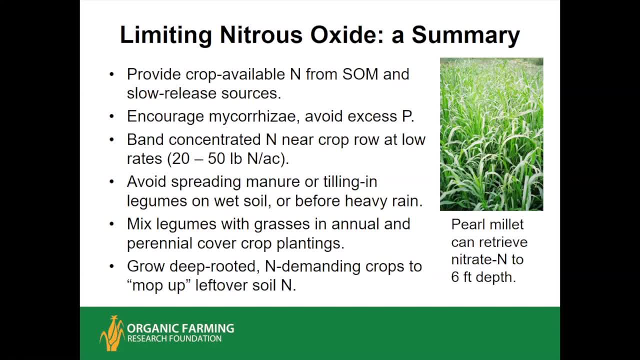 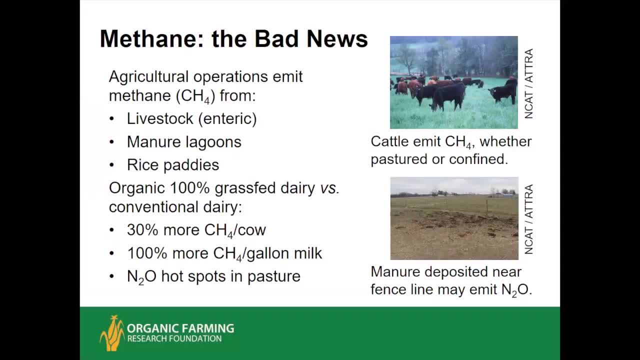 to mop up leftover soil. nitrogen Next, Okay, methane Next. we'll have to go quickly here. The bad news is that cattle emit methane whether they're pastured or confined, And in fact, when they're pastured, on kind of low-quality. 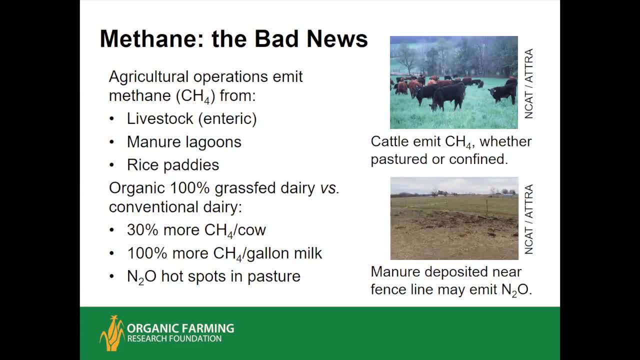 forage like very coarse grass, their emissions go up somewhat. Other sources of methane are manure legumes and rice paddies. Another thing that can happen is when you have pasture where the cattle are a long time and you have that manure accumulation by the fence. that can be a source of nitrous oxide. 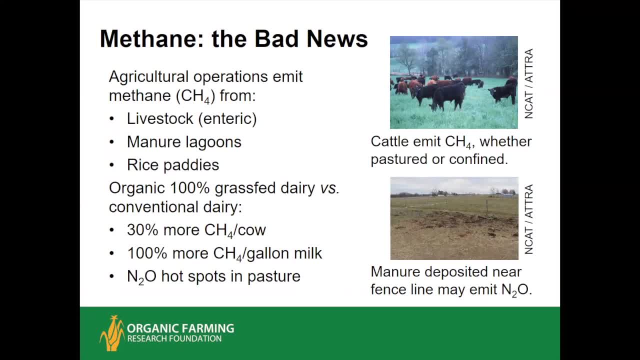 One study made organic 100% grass-fed dairy look kind of bad. It was emitting 30% more methane per cow and it went only up to 100% more per gallon of milk because production was a bit lower. And then there were not nitrogen. 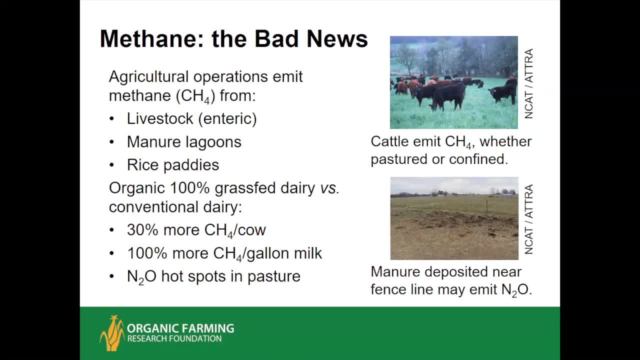 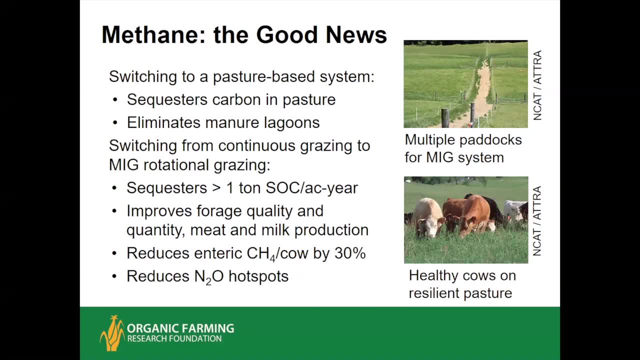 nitrous oxide hotspots in the pasture. Next slide Now. the good news is simply switching to a pasture-based system does two things right away: It sequesters carbon in the pasture and eliminates manure legumes. And when those two factors are taken into account by that very same study that made organic milk look so bad. 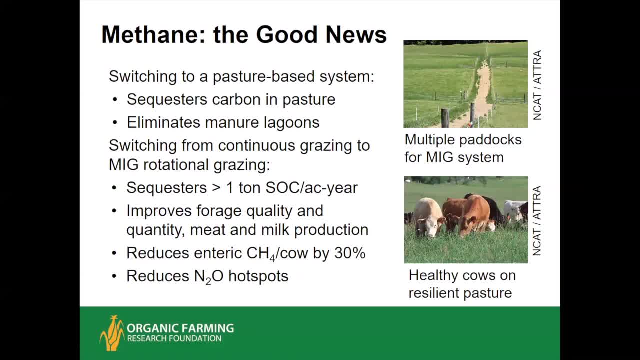 all of a sudden doesn't look so bad. Its greenhouse gas footprint drops to 80% that of a confinement dairy. And if you then transition from just a basic pasture system, from continuous grazing, to management-intensive rotational grazing, you have these multiple paddocks and you move the cattle from one to the next every couple of days, so they're always in really good quality pasture. 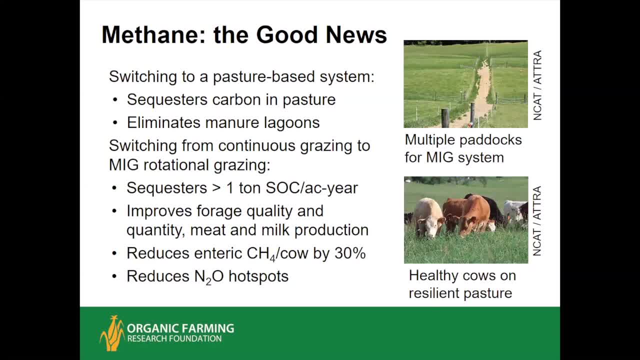 Several things happen. Your land is sequestering lots more carbon. Your production is improved because of better forage quality And because they're eating more balanced forage with more protein, their enteric carbon methane drops back down to where they would be if they were being fed grain supplements. 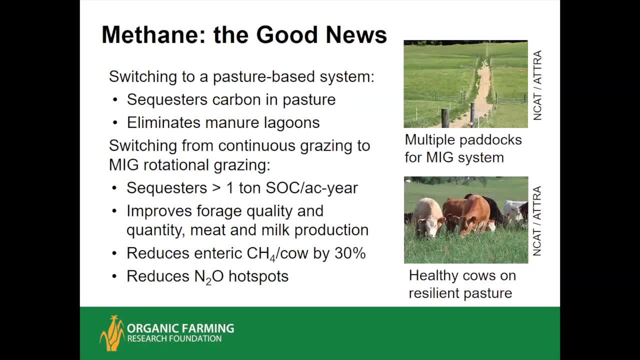 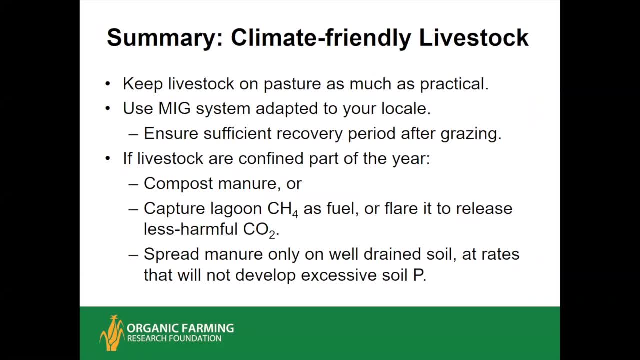 And then by the good rotational grazing, you don't have so much of those nitrous hotspots Next. So keeping a livestock and pasture as much as possible using the management-intensive system as adapted to your locale. There's many variants on it. 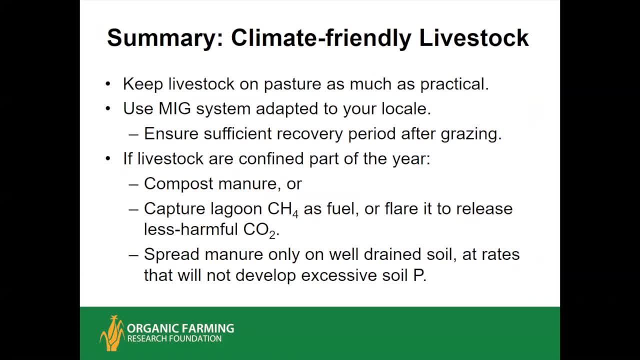 But it has worked everywhere across the country. If you do have confinement for part of the year, like you're in a cold climate, either compost the manure or, if you've got to keep it in a lagoon, install something so that you can capture that methane. 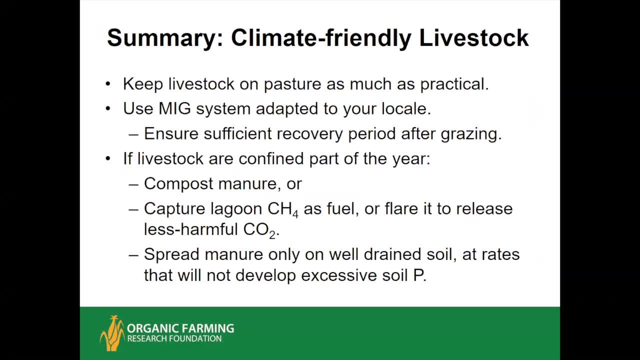 Have it completely enclosed to use as fuel. or even if you can't market it as fuel, if you flare it as carbon dioxide, you're reducing its impact by seven-eighths. And then be sure to spread manure at rates that don't build up excessive soil. phosphorus. 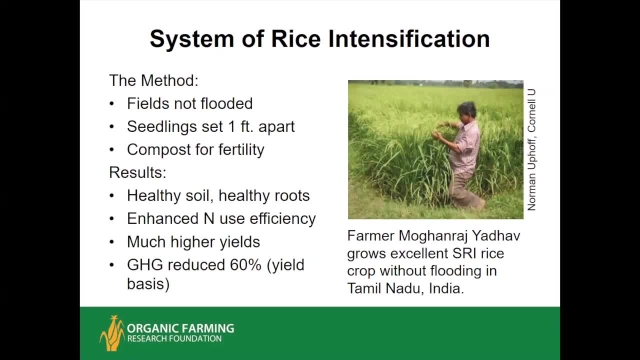 And only on well-drained soil. Next, System of rice intensification. We're pretty much out of time. I just wanted to say that this is a non-flooded method of rice production that greatly improves crop health, soil health and it pretty much very much reduces the methane emissions, slightly increases nitrous emissions because the soil is very wet but it's not flooded. 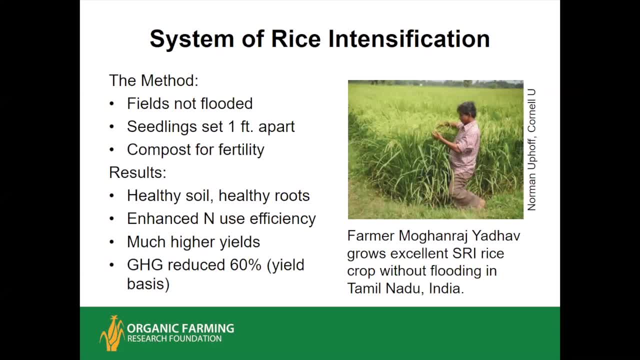 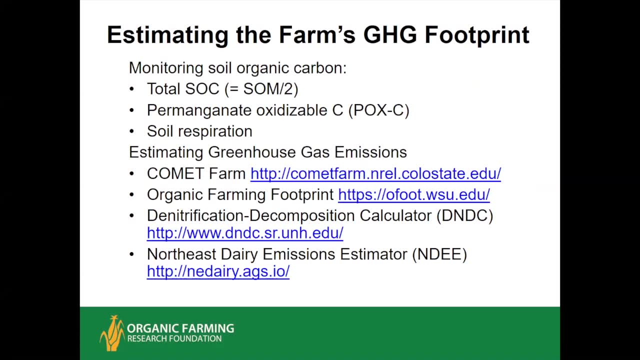 But overall the greenhouse gas emissions per ton of rice Next. So I haven't spent much time on this aspect of it, but there are some models out there that will help either a whole farmer or particularly a dairy farm to estimate their greenhouse gas emissions and to look at waste strategies to reduce it. 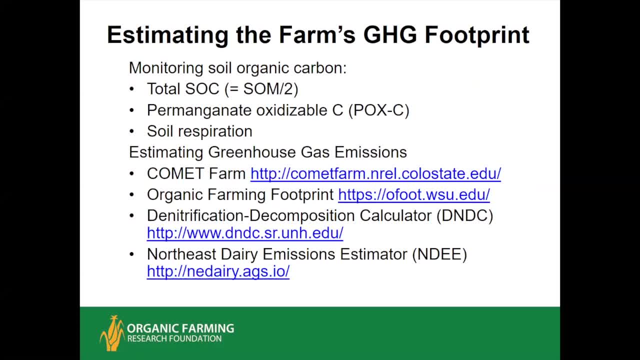 These are also some parameters that are useful for monitoring soil organic carbon. Total soil organic carbon is a good measure, but it Changes very slowly, so it's not responsive short-term. This one, the permanganate oxidizable carbon, which is becoming more available to farmers, is also a source, a way to monitor microbial activity and especially microbial carbon sequestration activities. 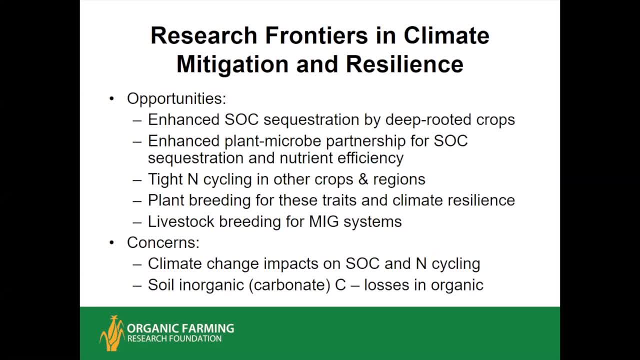 Next The research frontiers opportunities. carbon sequestration by deep-rooted crop- That's really exciting To me. enhanced plant-micro partnership, again for sequestration and nutrient efficiency. This tight nitrogen cycling: there's evidence that that's not limited to tomatoes in California but could be realized in many crops in many regions. 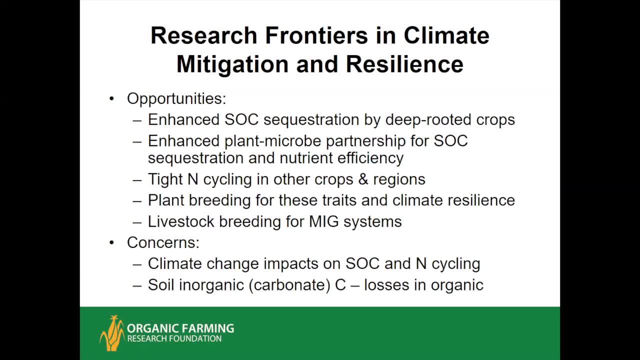 I think there's an important frontier in breeding plants for all of these traits: Deep, extensive root systems, excellent association of microbes and tighter nutrient cycling, Developing livestock that are better. They're adapted to the management-intensive grazing systems. A couple of concerns. 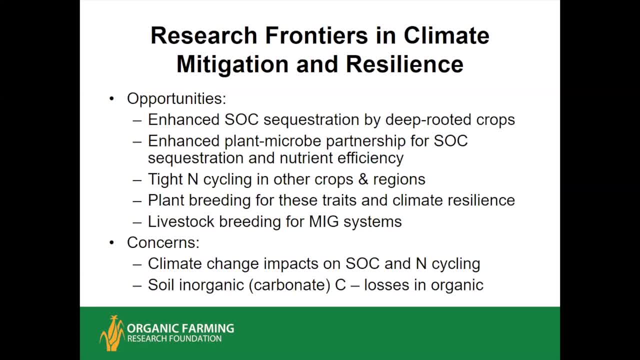 One is climate change itself will make it harder to store organic carbon and will somewhat accelerate nitrous oxide emissions as climates and soils get warmer. So that is a concern. Another one is we don't know the dynamics of the soil inorganic carbon or the carbonate carbon, which is 25% of total soil carbon. 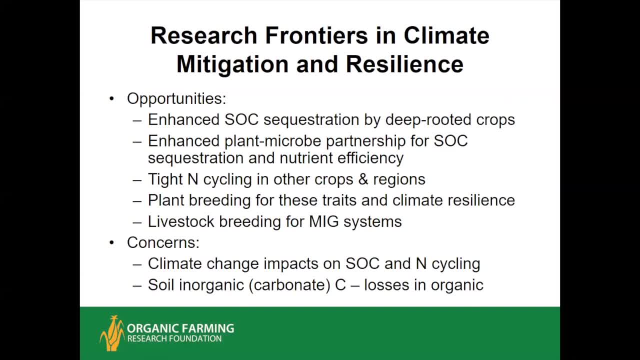 Now, if you have a field, Now this occurs. This carbonate is an important part of soil- carbon in semi-arid climates. So when you get on the soil and the pH is 8, you say, well, I need to lower the pH to 7.. 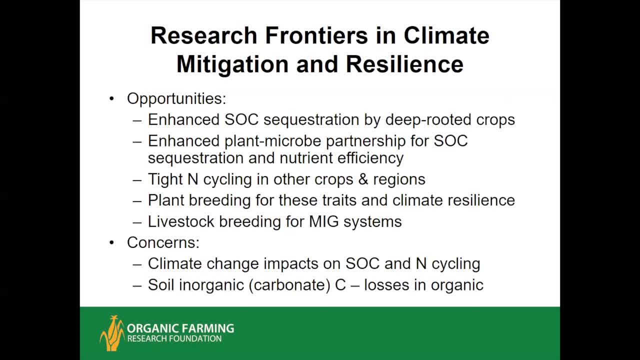 Well, what's going to happen? You lower it to pH to 7, all of that carbonate is going to turn to carbon dioxide. And there were seven studies of organic versus conventional in high carbonate soils. Three of those showed significant losses under the organic system, probably because the soil health building practices. 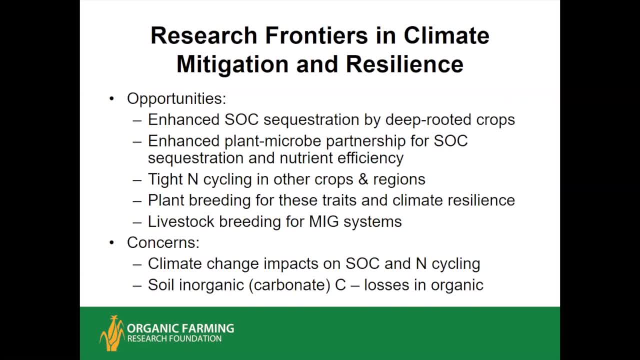 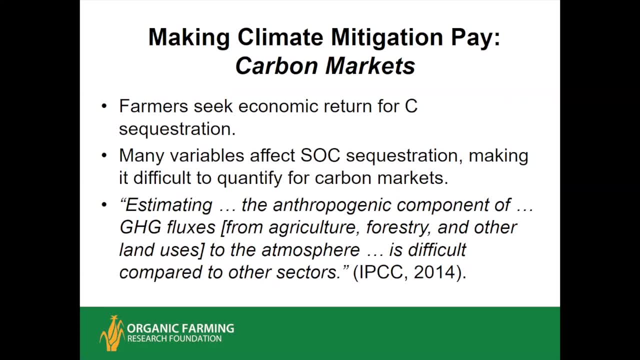 also modified pH and modified carbonate cycles, So this is an area that we need to look into. Okay, next Making: climate mitigation pay Carbon markets. The constraint here is that it's hard to predict exactly how much carbon you're actually putting away in the soil. 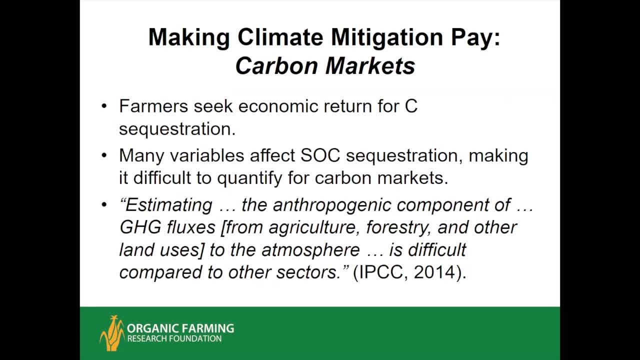 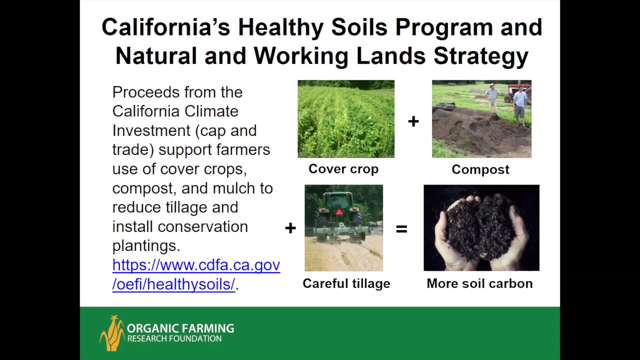 So it's very hard to connect that to a market. It's acknowledged by national and it's hard to quantify precisely. Next, In California there is a healthy soils program and now more recently announced by the Secretary of Agriculture in California. 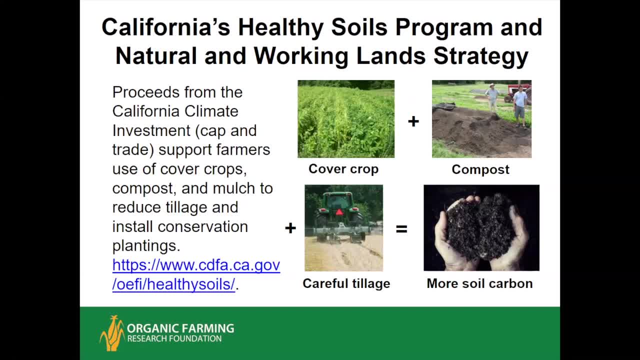 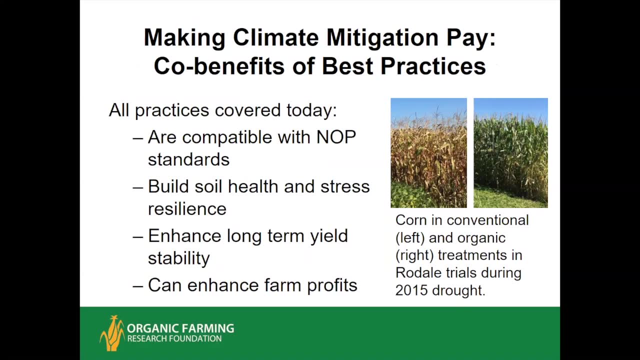 the Natural and Working Land Strategy. This is providing indirectly through a carbon market is providing funds to support farmers to adopt organic practices that will enhance both resilience and sequestration. Next, Well, you can't. even if you can't earn directly carbon credits, it really pays to adopt a lot of these practices that are compatible with organic standards. 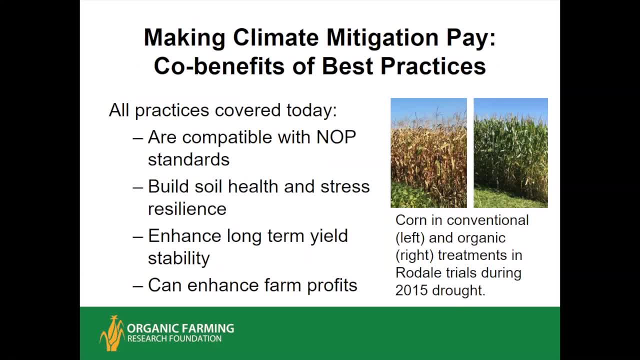 They build soil health. they build resilience to stresses. Another- this is another example from the Rodale trials: a different drought year. Again, the conventional crop burned out a lot faster and yielded about 30% less. You have this long-term yield stability. 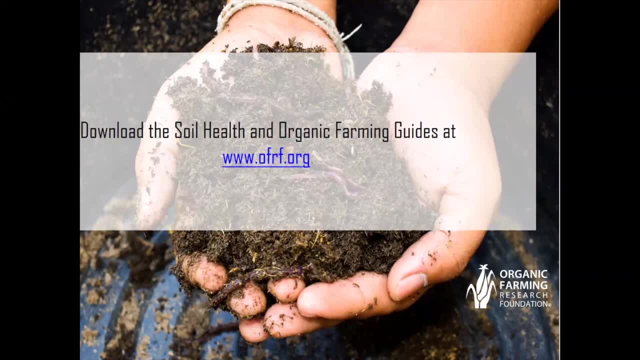 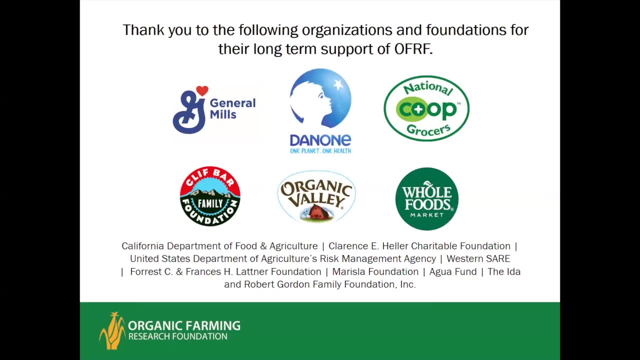 And okay, So the soil health guides are available through OFRForg. And then next, I want to thank all of the people that have made this wonderful work by OFRF possible. Here are the sponsors, And I'm sorry I did run a little over, but I'm certainly open to questions. 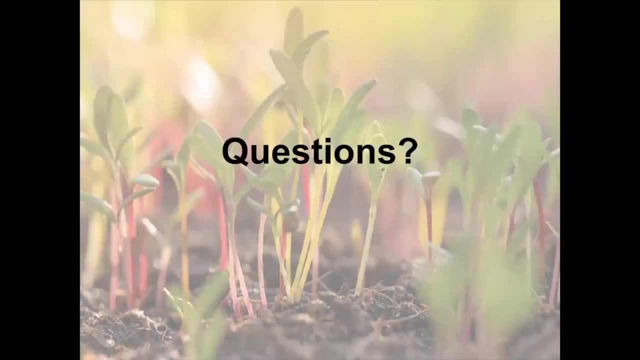 Okay, Thank you, Mark. We will probably run a little bit over time on the questions too. in case there's a lot of questions, I want to give people a chance, Otherwise we'll end a little early. If you have a question, you can type it into the Q&A box on your screen and we will read the questions out loud until we run out of time. 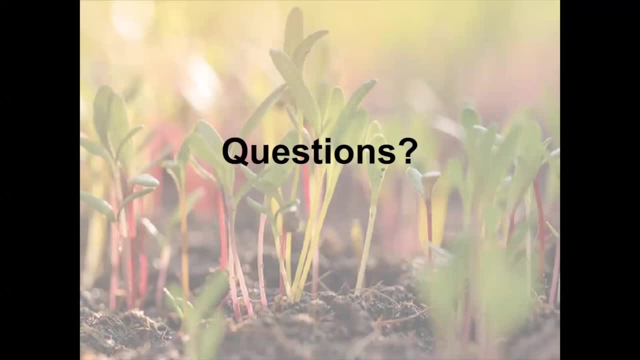 If you don't see the Q&A box or the chat box, there should be a bar with some controls. if you hover over the screen And if you click on the Q&A one, that should pull it up. I also want to mention that this presentation was recorded. 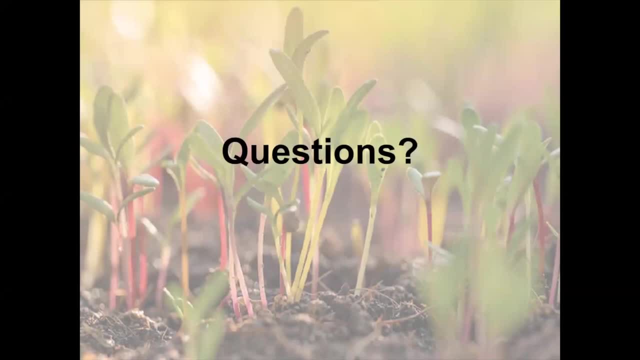 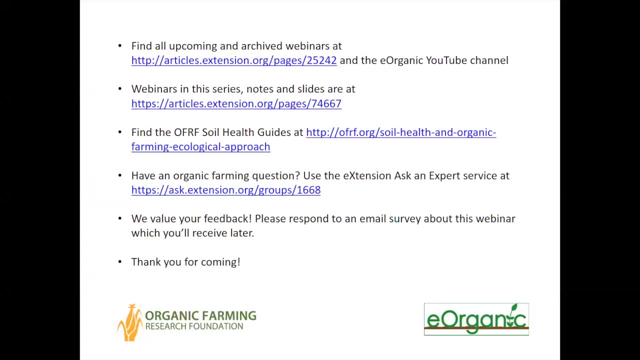 So if you missed the beginning or if you want to watch it again, you'll be able to find the recording. Okay, Okay, Okay. So we've had about a week on the eOrganic YouTube channel And I'm just going to pull up a slide with a link to where you can find the presentation notes, a PDF handout of the slides and all the recordings of the webinars in this organic farming and soil health series. 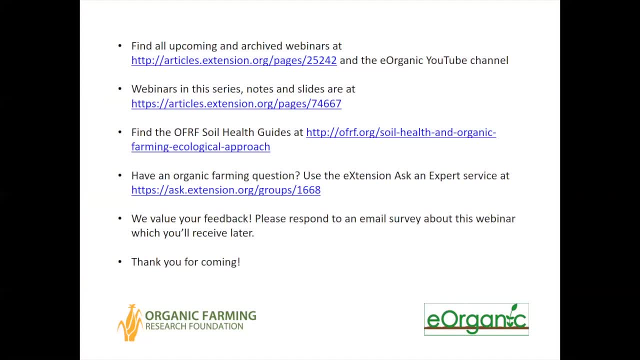 So, moving on to the questions, Let's see The first one. you may have answered already in the slide about carbon saturation, But I'll just ask it again because it's free. raised a little differently, The ton of carbon sequestered through MIG grazing will only happen. 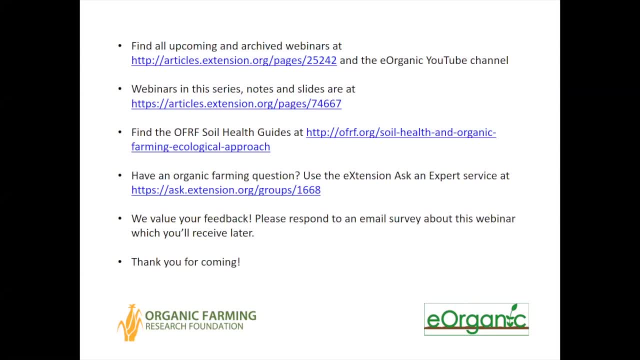 up to a point where the soil reaches maximum carbon. Is that correct? Yes, that is correct. One thing to remember, though, is that the benefits of resilience are ongoing. They don't end with that initial, with that initial initial increase, So and? 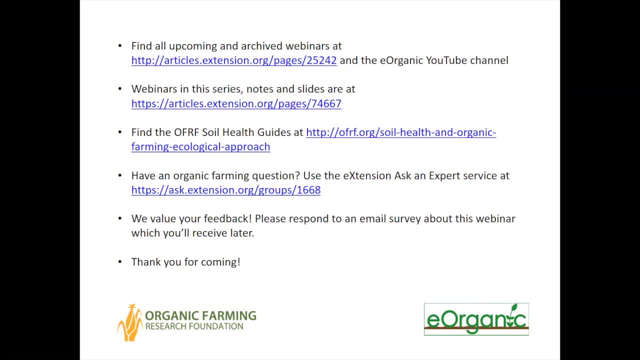 it's. it's not clear, one of the things about some of these studies. you can't study the whole soil profile that intensively, so there may be some deep carbon sequestration that goes on for longer, but it is true that there will be. 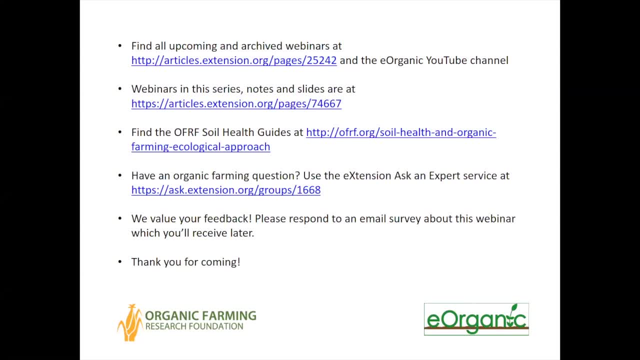 that saturation curve. Okay, here's a question about whether you know of any growers who are successfully practicing organic no-till production on a scale larger than more than a hundred acres, besides Rodale- Oh, that is a good question. Probably not organic. 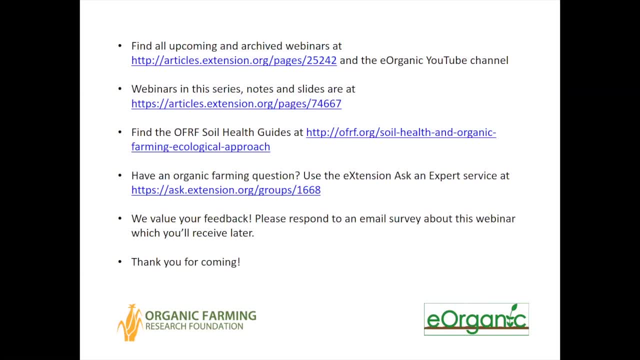 continuous no-till. There certainly are some advances in minimum tillage. One example I can think of that's been applied in semi-arid regions and I know that's a good question. but I know that's a good question- Probably not organic continuous no-till. There certainly are some advances in minimum tillage. One example I can think of that's been applied in semi-arid regions and I know. 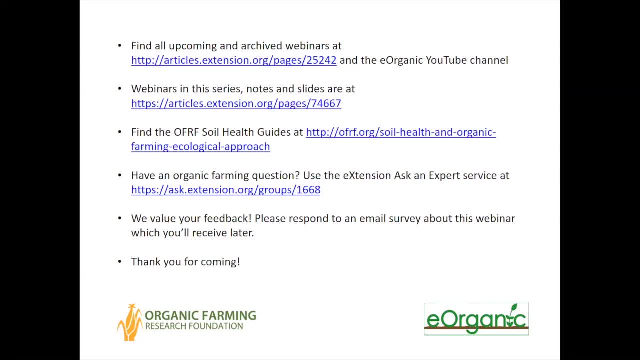 at least one ranch is doing one farm that's doing it at 7,000 acre scale. that's Villica's Farms Doug and Anna Crabtree. they use a sweep plow undercutter to terminate cover crops and knock out small weeds ahead of planting. 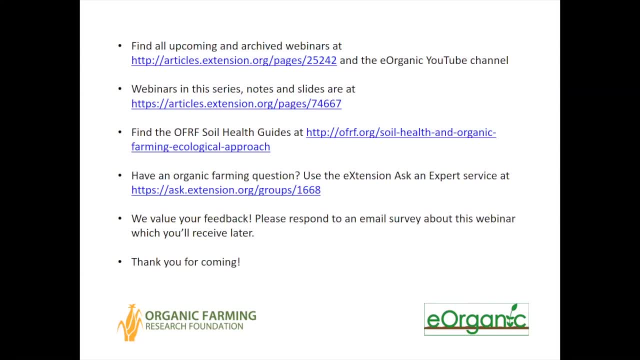 They never. they never turn plow that soil. So and then Gabe Brown is not fully organic but has continually phased down the amount of chemical inputs to where it's really vanishingly small. Now, this is not useful if you want to. 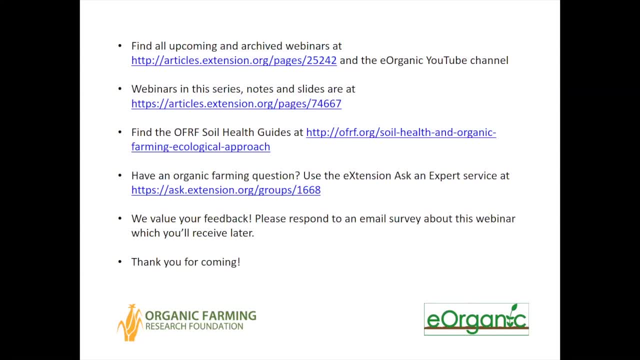 be certified organic. but he has completely eliminated tillage and has phased way down the synthetic inputs, Very rare to use as an herbicide or a pesticide or fertilizer. I see two basic approaches to this. The ideal is organic, continuous no-till and probably the only way you can really get there is. 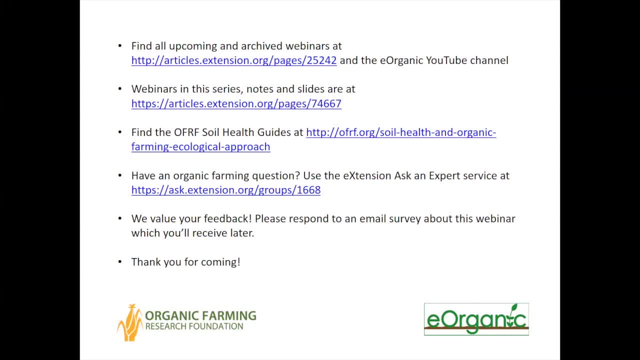 through a permaculture, perennial based system. If you're growing orchard, you can grow apple trees for a hundred years without ever tilling, if you do it right. So but we have two. we have two approaches to this idea. One is organic. 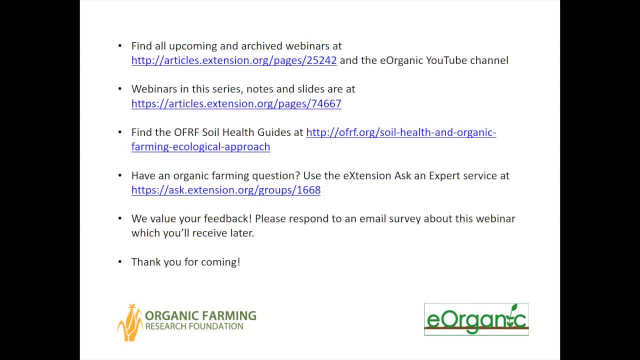 which is no chemicals till, as little as possible and as much as necessary. And the exciting thing is that there are more and more tools and techniques for minimizing that disturbance. Something like a sweep plow undercutter or for preparing a seedbed or rotary harrow only disturbs a couple inches of soil, so 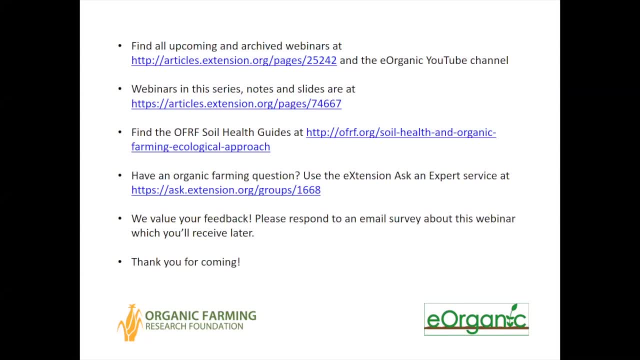 you're leaving most of the soil爱 soil- undisturbed, allowing those roots to break down naturally. The other thing about the best sustainable organic systems and conservation agriculture. and in conservation agriculture they swear off all tillage and allow judicious use of chemicals And the best conservation. 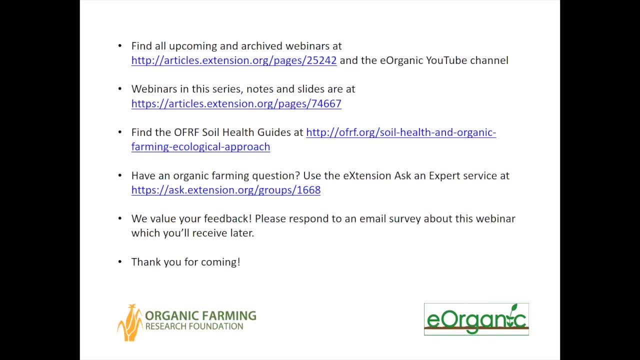 agriculture, farmers use very, very little of the chemical inputs. So that's a very good question. That's a challenge. These are the two approaches to it. Okay, Let's see Long-term cropping systems research at the Russell Ranch Sustainable Ag Facility at UC Davis, which is in a Mediterranean. 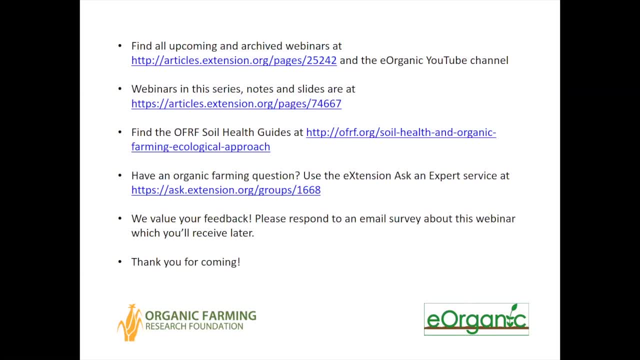 climate shows that cover crops do not increase long-term carbon storage in the soil, but compost does. As with many things in agriculture, it is hard to generalize when it comes to long-term carbon sequestration. That's a good question. That is very true. The figures that I quoted in those earlier are just broad estimates. 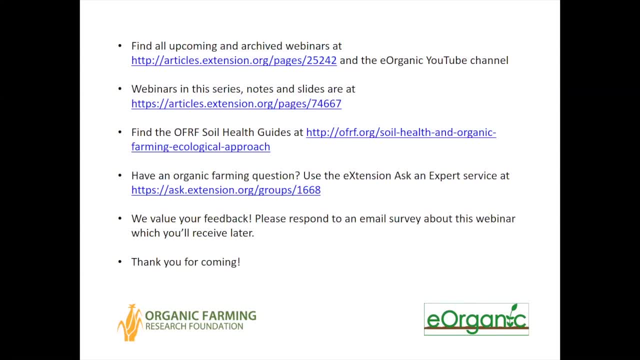 often based on multiple studies. Now it depends. I would want to look at that study. If those cover crops are being grown to a fairly young stage and then terminated, especially terminated by tillage, then, yes, probably nearly all of that will go into. 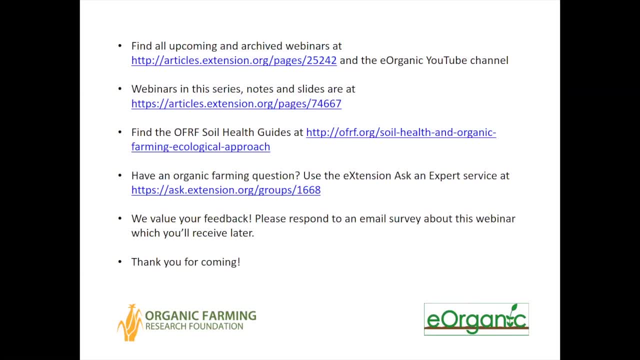 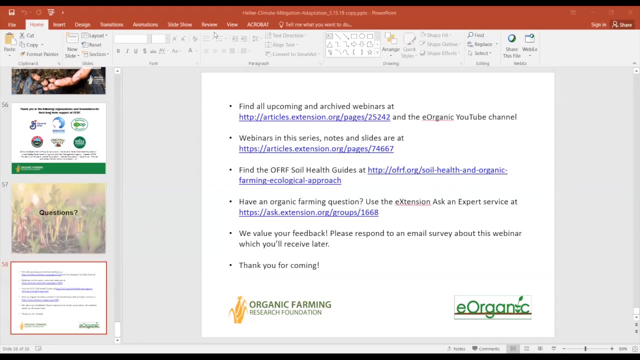 mineralization rather than stabilization. In fact, one of the studies- I've one of the meta-analysis. it covered several individual studies, some of which showed that the cover crop by itself will not build organic matter. Let me just ask you: do you know of any good practices in potato rotations to increase? soil health and soil organic matter. Good question: Potato rotations. Well, from my viewpoint down here in Floyd Virginia, potato harvest typically happens in July or August and that allows plenty of time to get a late summer cover crop. In fact, once we had a situation where timely cover cropping by one of my neighbors. in our little community garden we dug our potato crop and he got the sorghum seed and planted the next day And by mid-September this crop was four feet tall. And then we had a biblical rainstorm that caused the river to rush over that garden. and it basically roll crimped the cover crop, But because it was four feet of sorghum to then, we didn't lose a single shovel full of soil. Had that potato field been left fallow, we probably would have three foot gully. that would still be there. So I don't know. 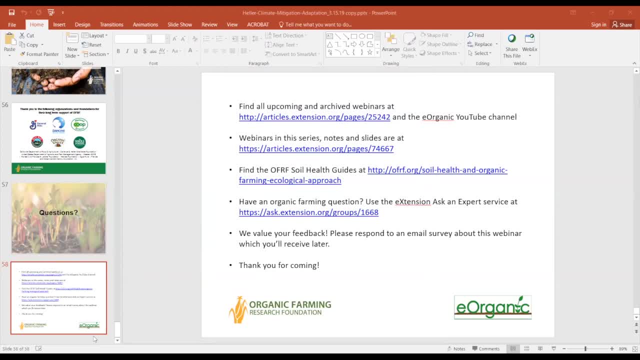 Follow the potatoes. You could follow it with a wheat crop undersown with a clover. Okay, Okay, Here's a question: Does the NRCS provide any funding to growers who want to put in place any of the conservation practices you highlighted here? 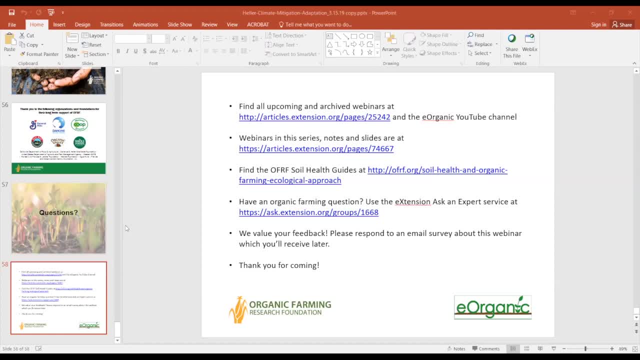 maybe to get a special kind of machine to avoid tillage or to plant lots of buffers. And before Mark talks about that, I know that we've had webinars in the past on the EQIP program, E-Q-I-P, which provides funding to farmers for conservation practices, So you might want to. 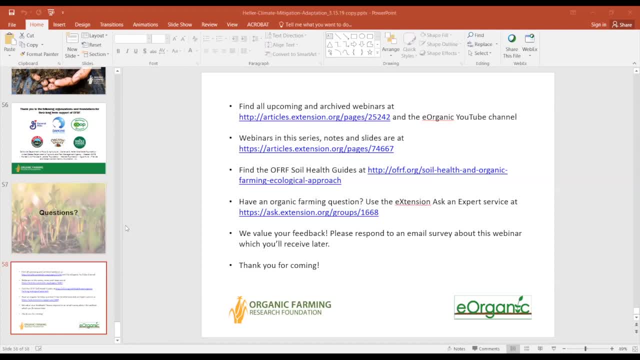 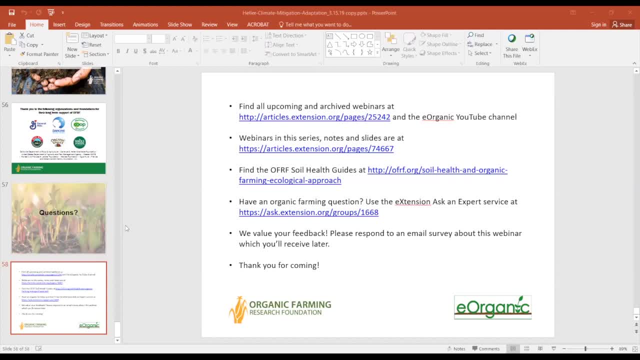 the crop no-till prescribed grazing conservation crop rotation, simply adding a third crop to corn soy. any of those can get cost share through EQIP. The Conservation Stewardship Program offers enhancements where you're going from a simple cover crop to a more diverse, higher biomass cover crop. 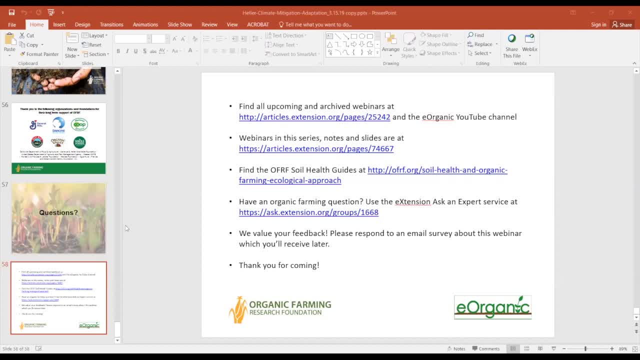 going from prescribed grazing as an EQIP practice to management-intensive rotational grazing. In fact, the new field is going to be a new field. So we're going to be going from a new field to a new field. So we're going to be going from a new field to a new field. So we're going to be going from a new field, So we're going. 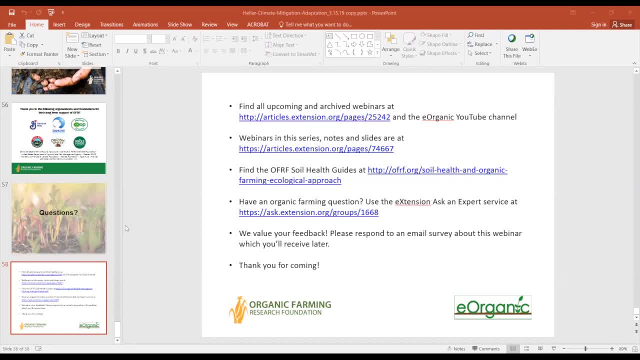 from a new field to a new field. So we're going from a new field, So we're going to be going from actual farm farm- возye-owl farming and emergency farm and emergency farm- Westernrod picotr authority garden business to managers from Glacier Bay. to managers from Glacier Bay. we're going to have a couple of closer calls with them, So they're certainly looking at that. we're also going to have an badge crack on their card. This is mentioned by the Department of the Department of cuts- that climate change is needed for socialyorsunal景 printer, And so I'm curious. 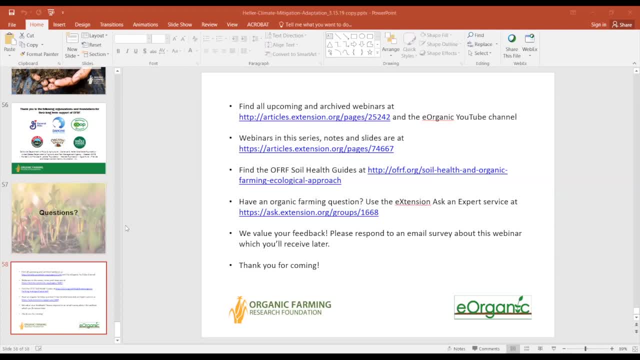 hedgerow That hedgerow. there was an example of an NRCS cost-shared practice. So yes, there is quite a bit of support and the more demand there is for it, the more chances are that we will increase funding and future farm bills for this very important work. 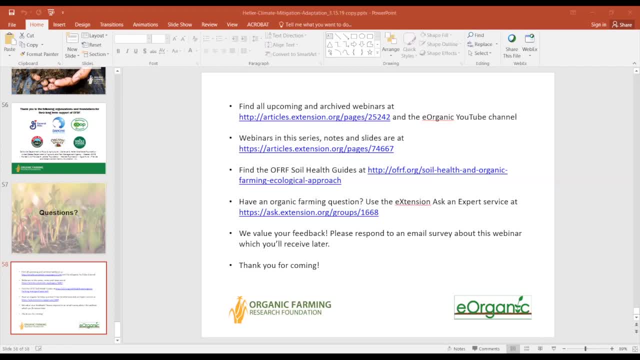 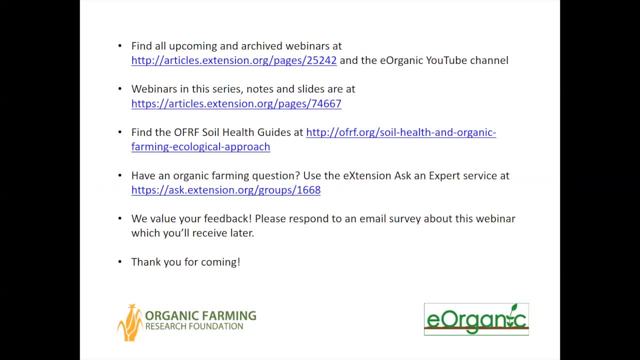 Okay, we had another question from the person who asked about whether you knew of any successful large organic no-till farms, and he was interested in knowing more about some of the new tools and techniques to till more effectively. We did have a webinar, by the way, on practical. 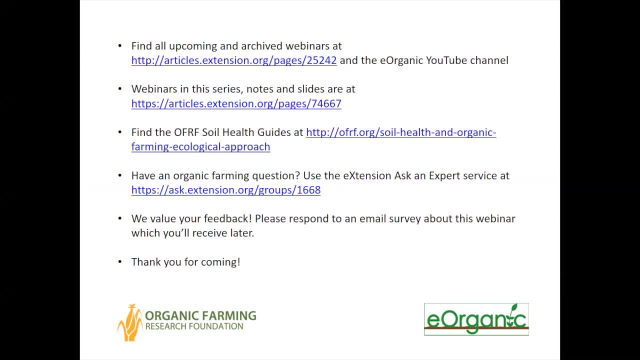 conservation tillage, so you might want to check that out as well in the eOrganic webinar archive, the link for which is on your screen. Well, I would first note that you can even do full-width tillage and do a lot less. 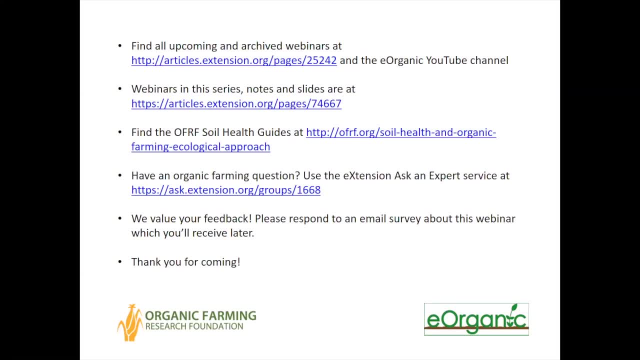 You can do a lot less damage to your soil than the classic plow disc. The spading machine was shown to greatly reduce compaction. I don't know what it does in terms of soil carbon sequestration, but anything that eases up on the. The two things to avoid are inversion and pulverizing. 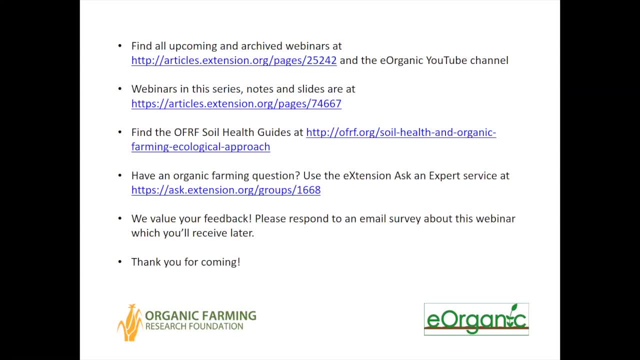 of aggregates And what the spading machine does, and this is most practical for a smallish intensive vegetable farm, but it basically It basically works the soil deeply but fairly gently, so you get a seed bed but you have a crumb structure that's preserved. You don't have it pulverized- A much more very low-tech solution. 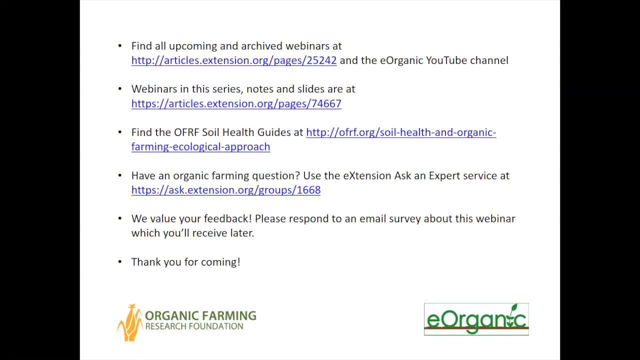 that a farmer in Virginia developed is to simply take the rototiller, which is infamous for beating the heck out of the top four inches of your soil. slow down the PTO so it's not turning as fast, but speed up your tractor so you're not hovering over any one spot for as many years as possible. 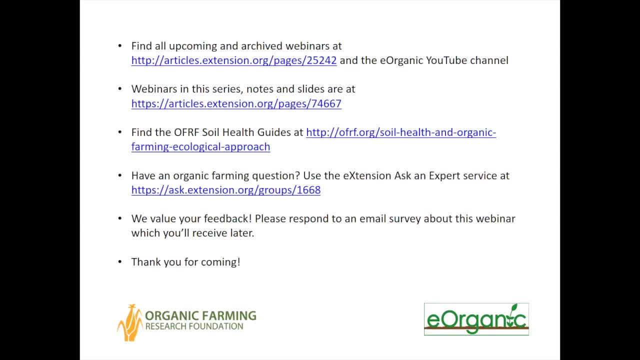 So, as a result, the rototiller acts more like a rotary harrow. and actually this farmer is farming on a very, very sandy soil and yet is able to see crumb structure remaining after the tillage pass, which is once a year. and he tills in a high biomass cover crop. That's another thing. 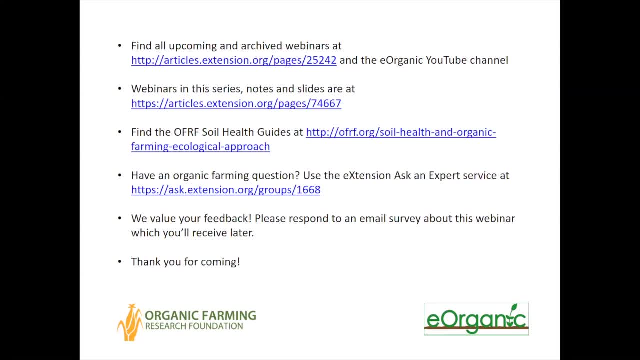 It's a matter of combining the practices. I would definitely refer you to that tillage webinar. Other tools that are exciting are the rotary harrow. That's a relatively new implement. There are various rigs being developed by Penn State University, Cornell and some of the 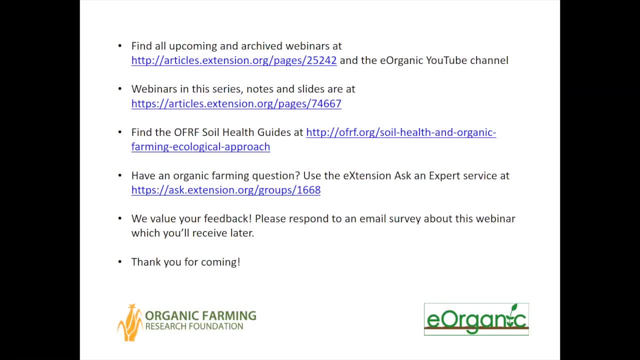 research facilities out west where you have like a coulter and then a shank and then a small rolling basket or other implement to strip till You till a narrow strip. That picture of careful tillage, as I called it, is actually a strip tiller. So yeah, there are many practices that do not. 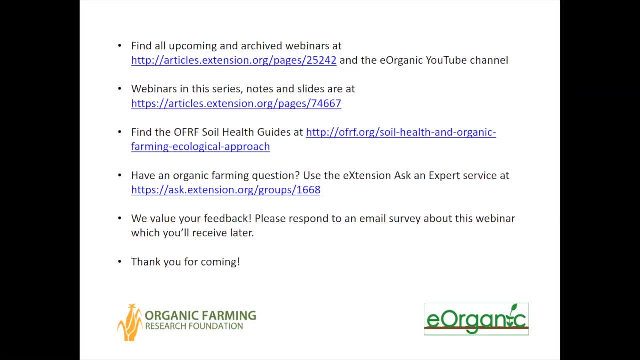 commit you to full, continuous no-till, but can greatly reduce the amount of damage to the soil. The sweet plow undercutter is really good for drier conditions. It's not so effective in wet soils or high rainfall climates. Okay, let's just leave one more minute or so in case someone else wants to type in a question. 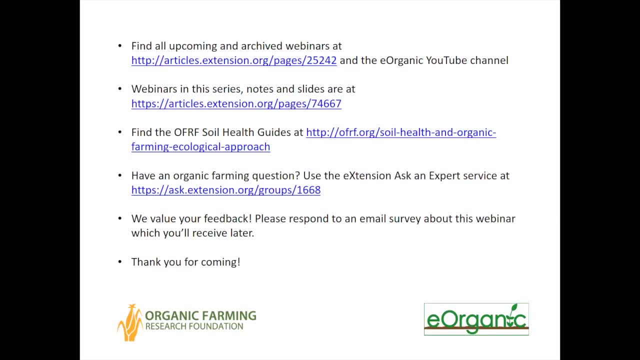 because we've gone through the ones that we had in the queue and this is your opportunity, if you're still on, to ask Mark a question. So we'll just wait one more minute here And again, I will say that the links to all the webinars in the series are here on your screen.